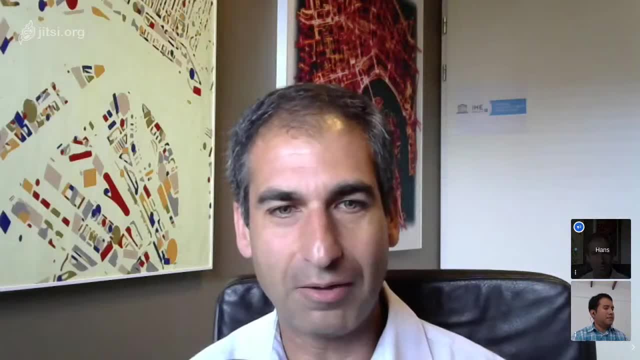 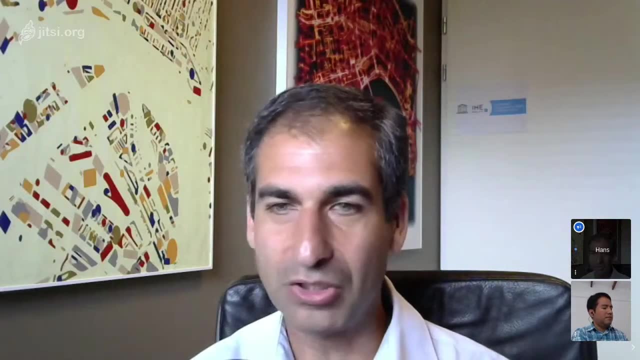 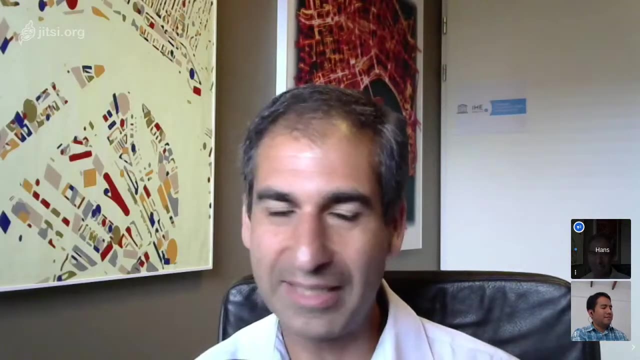 but I welcome you all. Please use the chat to introduce yourself And if you have any questions, also put it in the chat And then later we will give those questions to Sol Montoya from Hattari Labs. He's our guest Later. he will be joined by Gabriela, who will also answer. 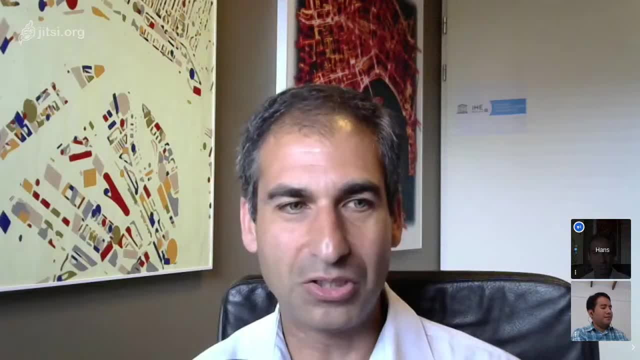 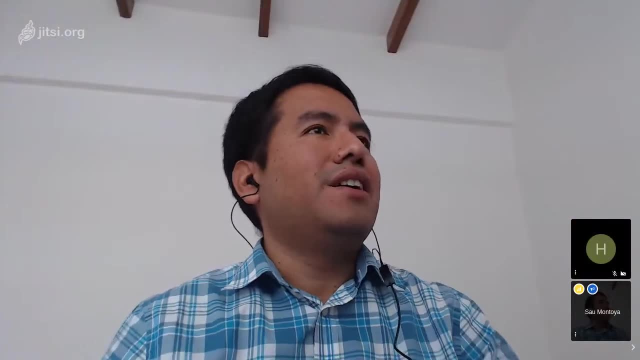 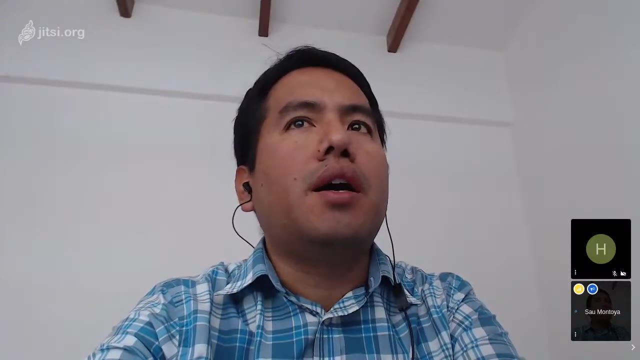 questions in the chat. So I'm going to give the floor to Sol Montoya. Sol Montoya, Sorry, Hi, Hi, Do you hear me? I hope that you hear me. well, My name is Sol Montoya. I am from Hattari Labs. 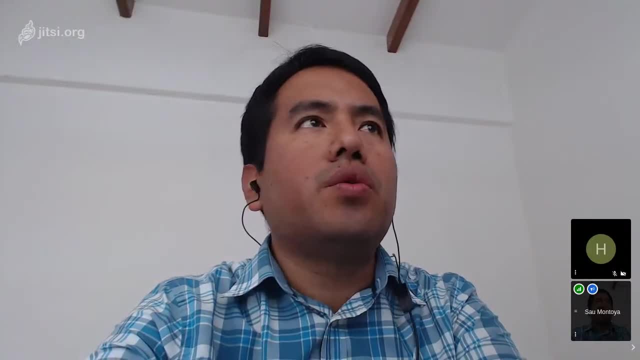 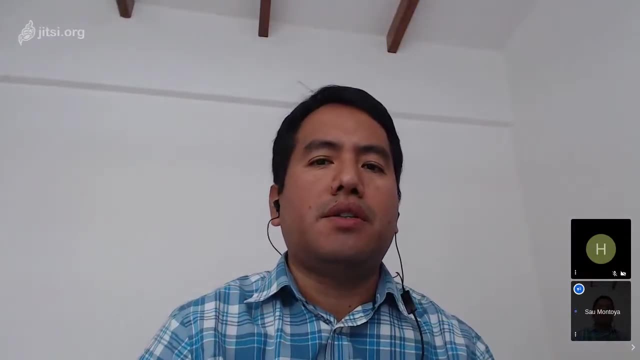 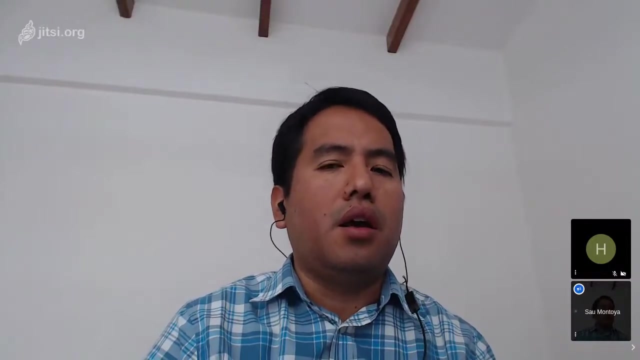 I am a geologist numerical modeler. We are going to give a course in groundwater modeling. This course is intended for general audience. I mean, this course is intended for people that know nothing about groundwater modeling, for people that have some knowledge in hydrogeology. 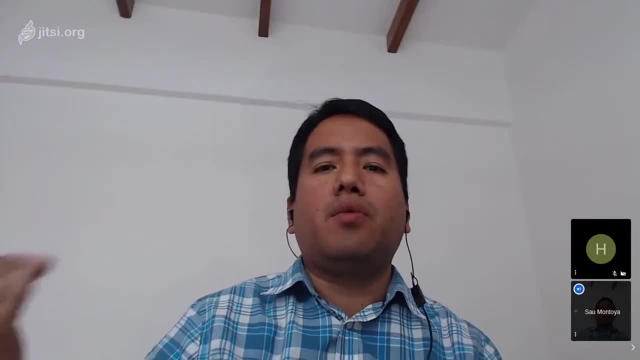 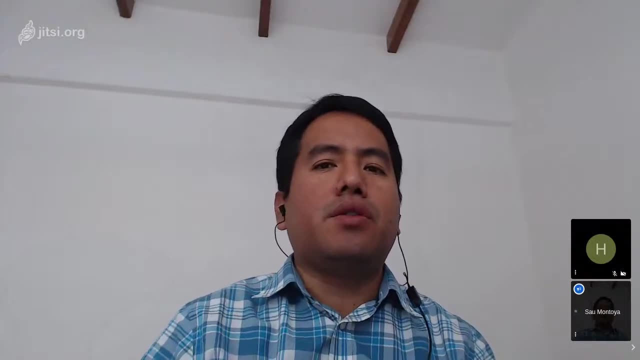 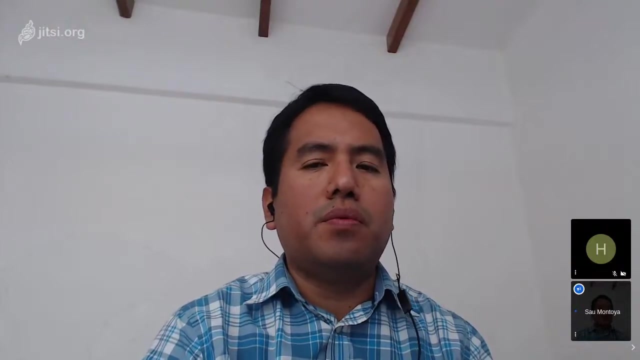 and for people that were using another software and they want to switch to this open source software. Okay, I will share my screen, So this is the last time that they actually will see my face. There is a great support over YouTube, So when you have any, 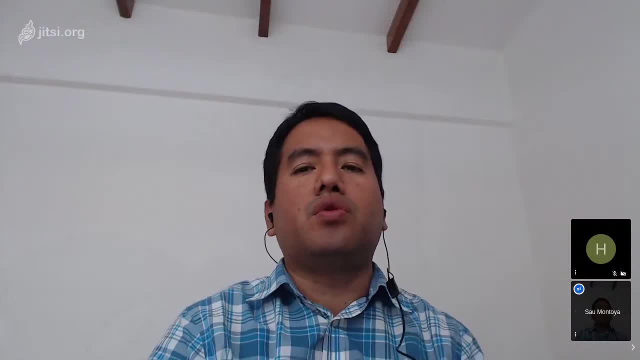 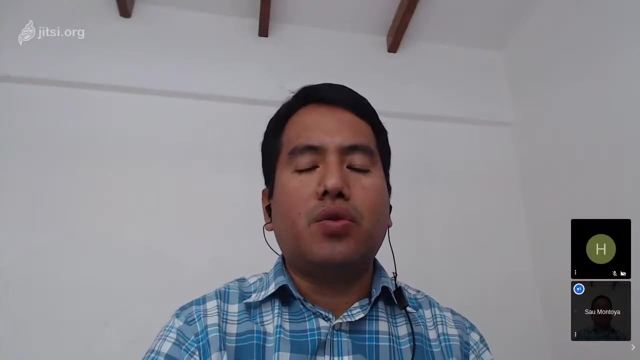 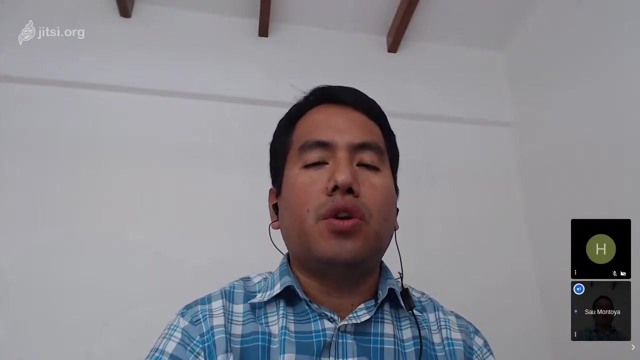 questions. you can make your questions through YouTube. Gabriela will be supporting and giving answers through YouTube And I will ask some. This is a new step on the online classes, because I want to know how well you are doing So, if you are. 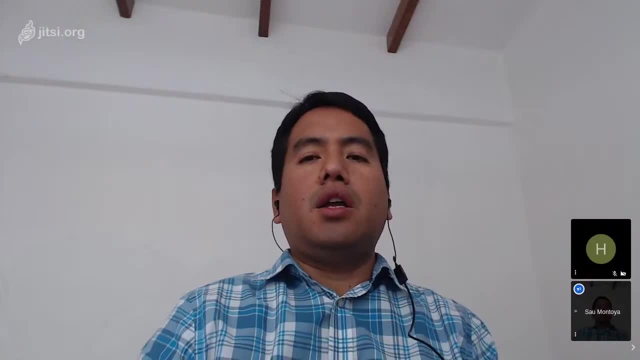 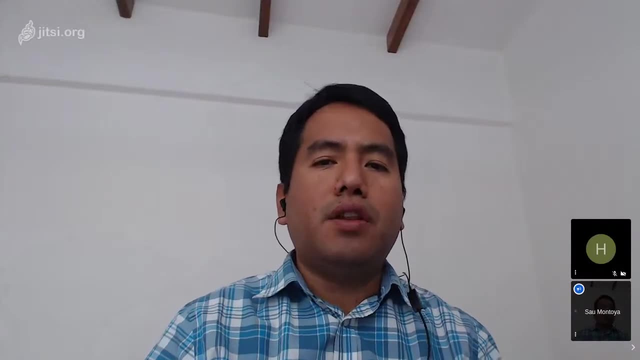 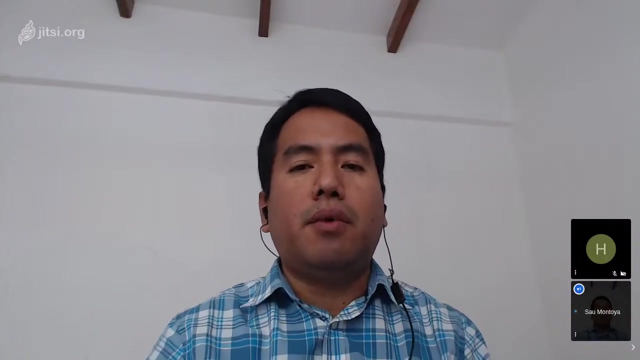 doing well. I'm going to ask some questions about if you are at this point, please type yes one, yes two, yes three or yes four. Why? Because for me it's the feedback if you are doing great or maybe you get lost, Okay. So if I don't receive this feedback, we might have some problems because I can't. 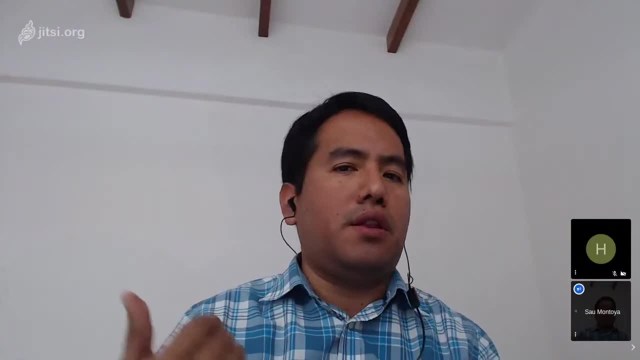 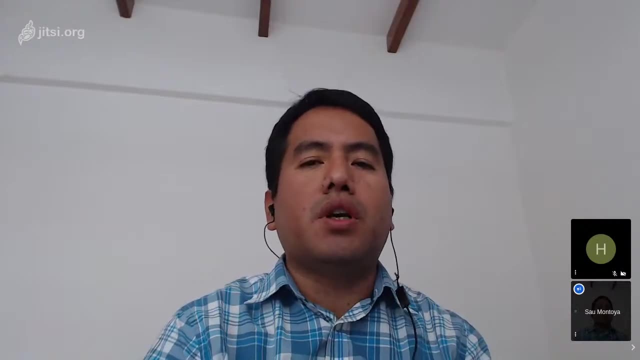 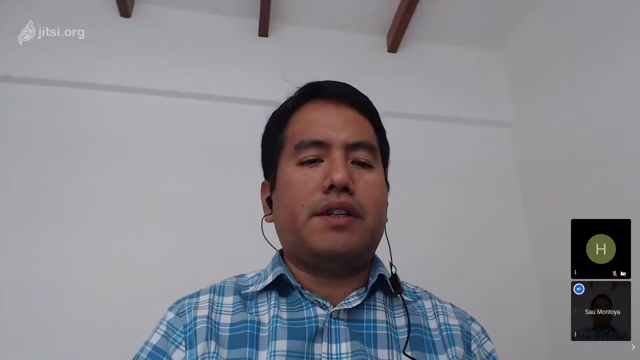 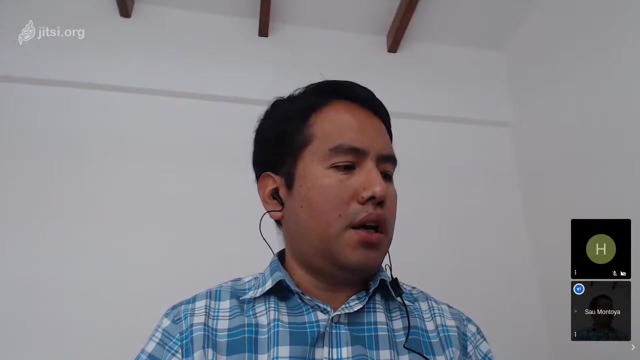 do? I mean, I've been dealing with software more like 15 years with the groundwater software, and I can do things much, much quicker. So if I don't hear from you, I think that I can do a much faster speed, a faster step. Okay, So, Hans, if everything is right with the mission, can I ask? can I start? 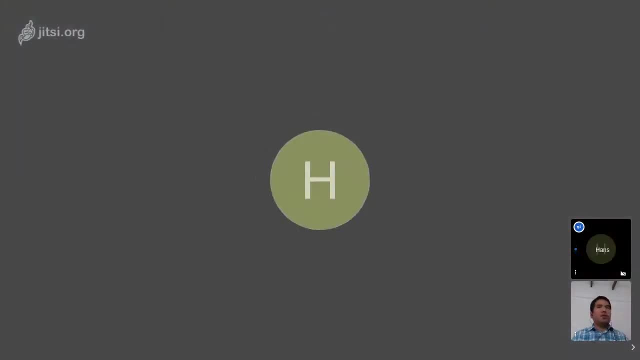 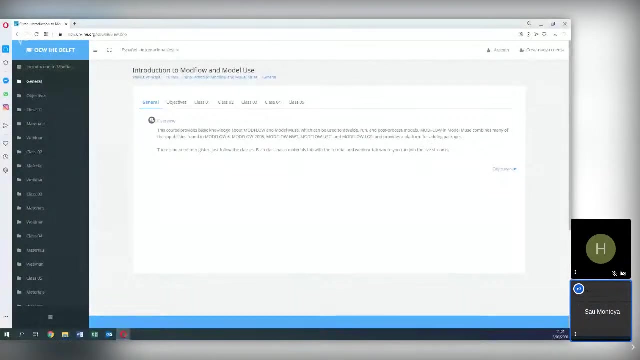 the course. Yes, So go ahead. Everything, Everything is on and we have 99 people in the live stream and they're interacting, So go ahead, Okay. So I will share my screen, Okay. So let's have a review on the objectives of this course. The 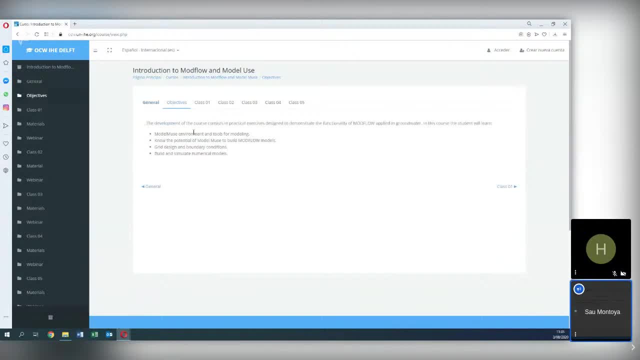 So with this course you will know the model mills, environment tools for modeling. They know the potential of model mills to build model models- grid design and water conditions- and to build and simulate numerical models. Okay, We Hydrela Apps was designed as a website for a consulting company. 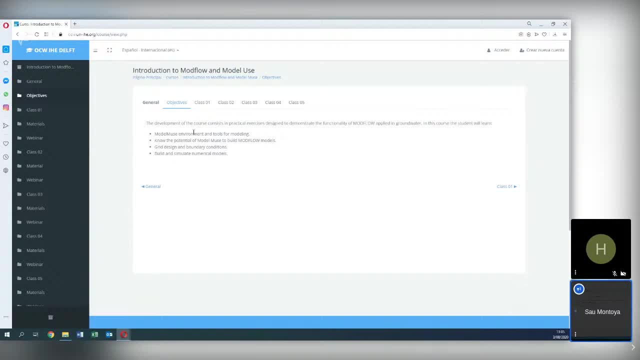 but later on it turned into a blog, Okay, And in this blog we have lots of stuff on groundwater modeling, Maybe, and it might be like the main repositories of tutorials on Modblog, okay, but these tutorials are applied tutorials, so in this course, we will give the basics in order to 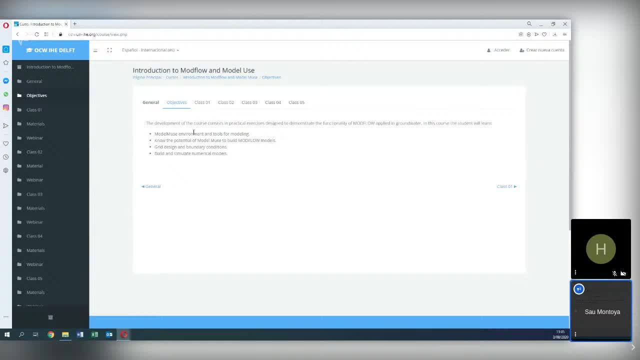 understand the software so you can do like it's like kind of tutorial or a case that is close of what you are doing, okay, or your interest, okay, great. so on the, on the first class, we are going to have a description of Model Muse, the buttons and so on. however, yeah, there is a tutorial here. there was a tutorial. 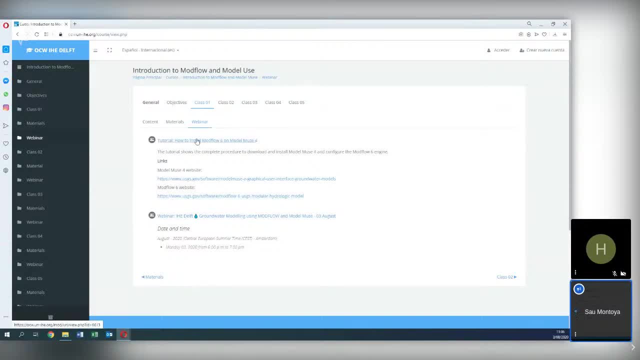 here. that is this tutorial to install Modflow 6 and Model Muse 4. yeah, I hope this was on the that. you have on Modflow 6 already on your computer. I hope so. yeah, and if you have this on your computer, please type yes. 1. so now we are, we will start with. 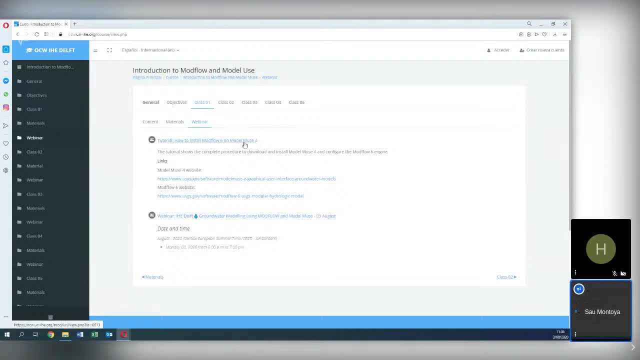 these questions, if you have, if you have followed this tutorial and then you have Modflow 6 and Model Muse 4 on your computer, please type yes 1. okay, yes 1, yes 1. the number is is really important because we are going to be yes. 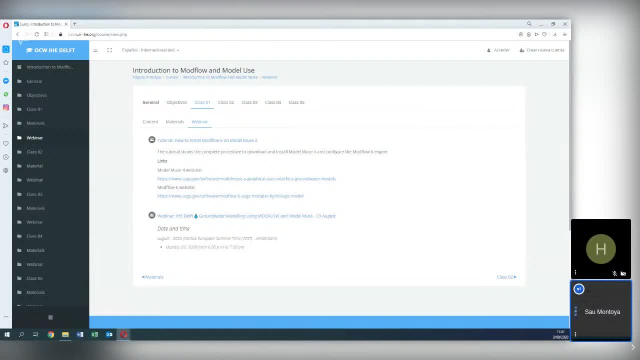 15, something like that. so it's really enough. okay, great, so you are. you are great in the tutorial. okay, well, let's see the website of model muse. but because is very important to see where everything comes from, okay material, let's talk about a little bit of model muse. yeah, model muse is a graphical user. 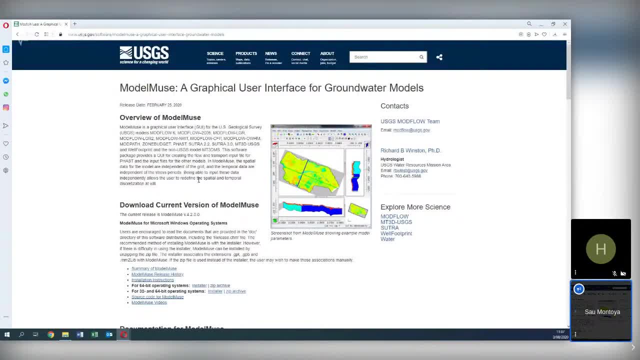 interface. so what is mean graphical user interface is is the normal environment where you have buttons to do actions. okay in, okay. so this similar of what you do in windows. so you have a button down open a document. you have a button where you can edit, you have a button where you can say: yeah, this is a. 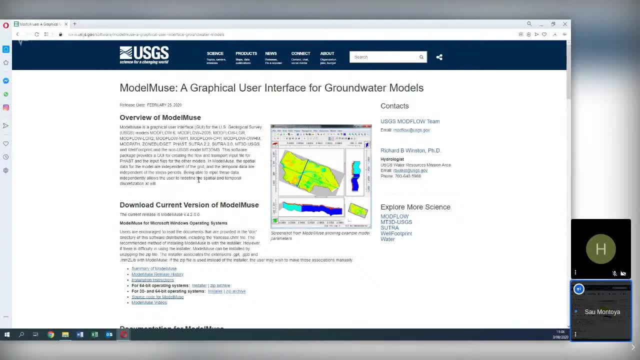 graphical user and model news is a graphical interface for groundwater models. okay, and in model news you can do and you can work, you can build, you can run and then you can analyze models that were done not only in modflow. okay, so you can work models in modflow 6, modflow 2005, modflow lgr, modflow lgr2. 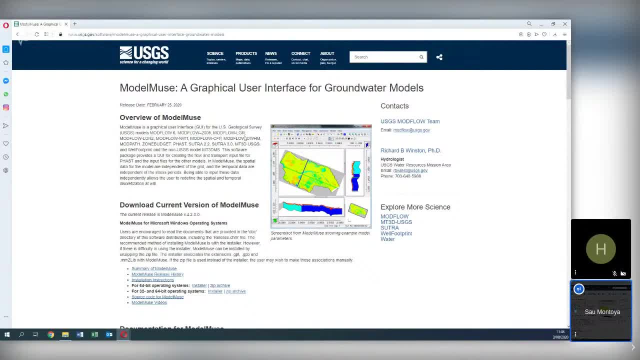 modflow, nwt, modflow, cfp, modflow, uhm, modpacks on budget pass sutra- and mt3d, ms and mt3d. so, as you see, there is a lot, of, a lot of model types done by the usds. okay, well, this is for you, because you will see. 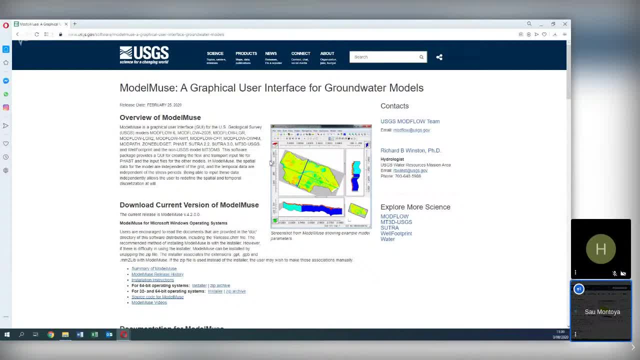 those options. on modern news, this course is intended to work with modflow 2005, i guess. yeah, the the word procedure is really similar of what you will do in module 6. okay, and for example, here we have, there is a summary of modern news. uh, if you are, i strongly recommend that. 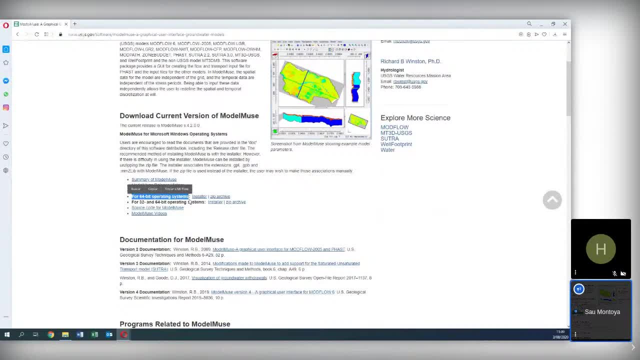 you work on the 64 operating system. i don't know if any of you have a 32 operating system computer. however, and in my experience, um, i see that there are more bugs on the 32 than on the 64.. okay, okay, great. so if you haven't, 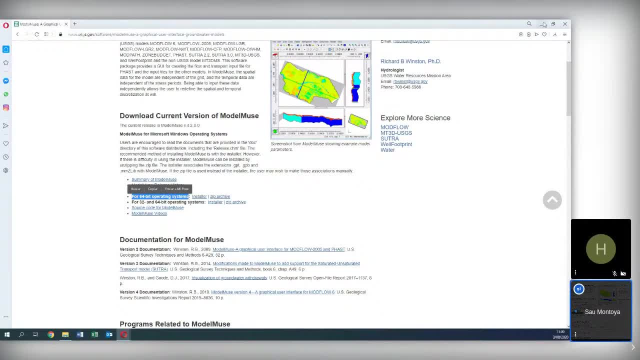 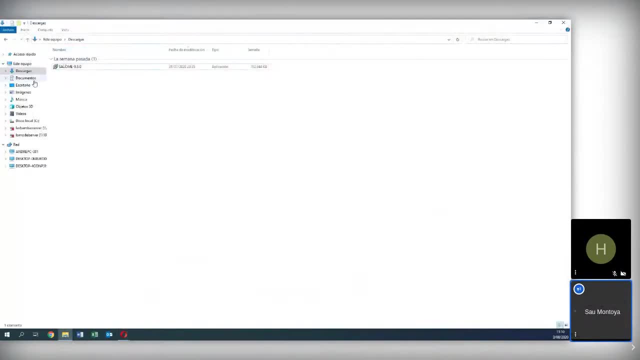 already. there are some material on the course that are the pdfs, and this is something great about those pds, because we are going to work with the pdf, so we are. we are not going to do anything that is outside the pdf. okay, and this is great. 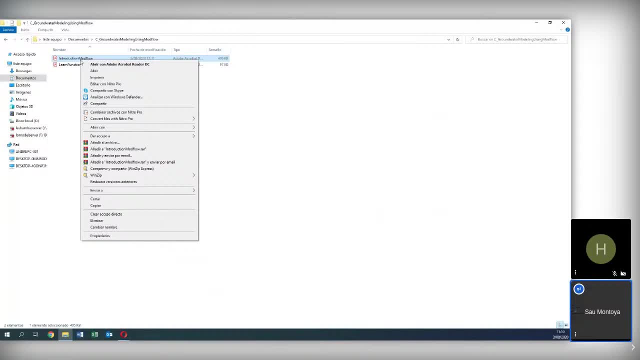 because if you want to recreate, or if you want to go back and see, or do it by your own. and this is the topic of doing by your own is really important, because what it happens on the course is that you, on the course, everything is perfect. so in everything, 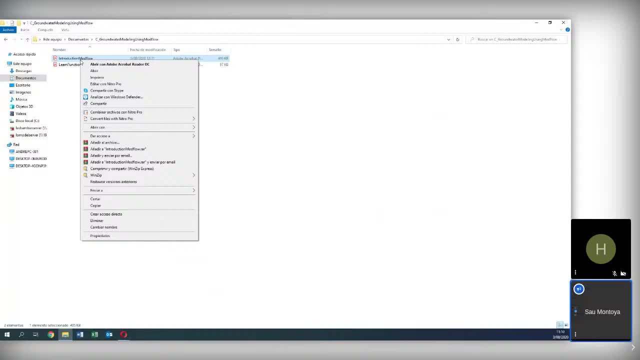 is, everything is great. so you work very well. you do your model, the model compares, you get the results and so on, and everyone is happy. but when you do by your own, you face a lot of challenge because- because models are not the same, So you have a model with another boundary condition. 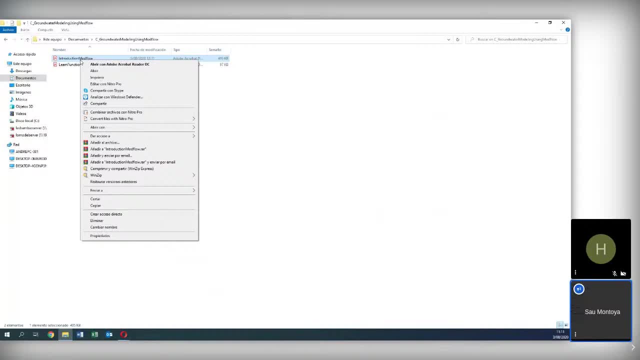 you have models with another challenge, on the boundary conditions or in this situation and so on. So that's why you need to have, like a guidance or say: okay, of course, what have we done in this step? Ah, okay, this is the step that we have done, okay. 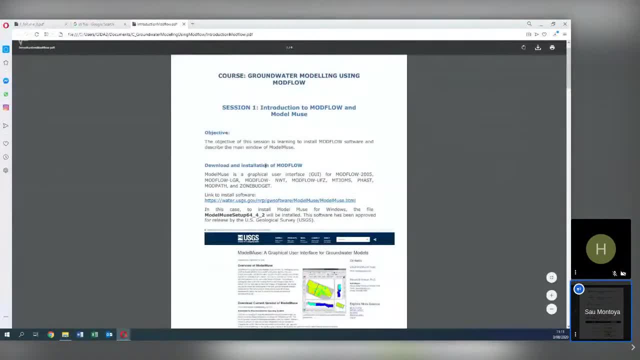 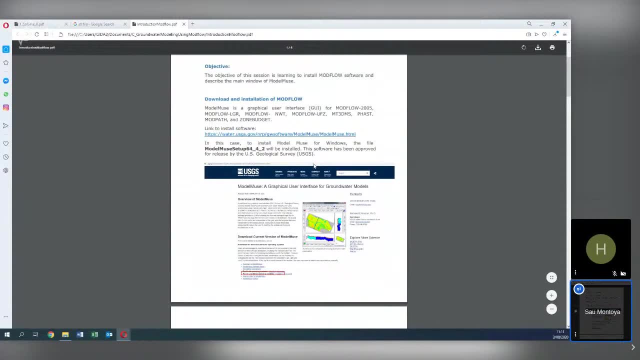 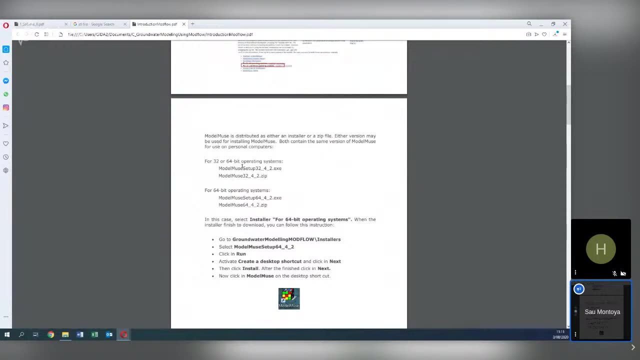 So I will open this and then: okay. So, as we have said, ModelMuse actually works with all of these models, okay, And there, well, you have already downloaded and you have already installed it. that's why you have told me. 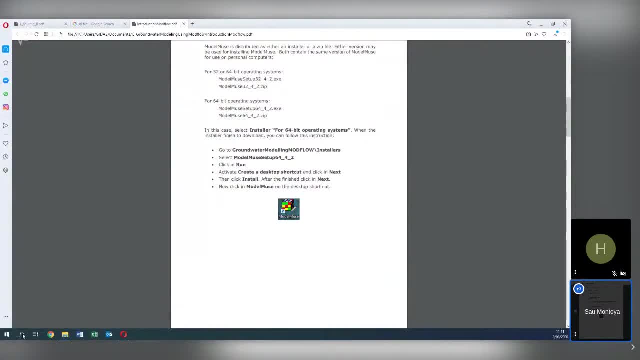 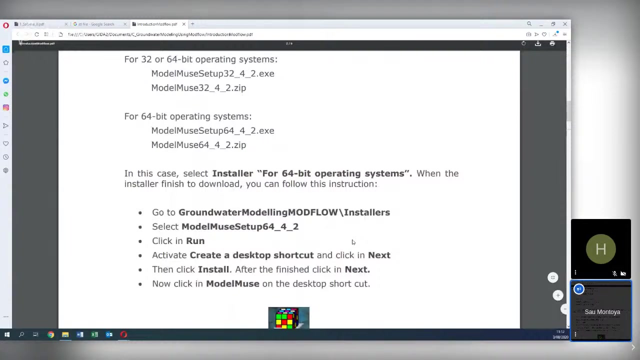 and then we are going to open ModelMuse. okay, So here In your computer, look for ModelMuse. Actually it opens in the other screen. okay, So here I will open in ModelMuse. okay, And let's see. 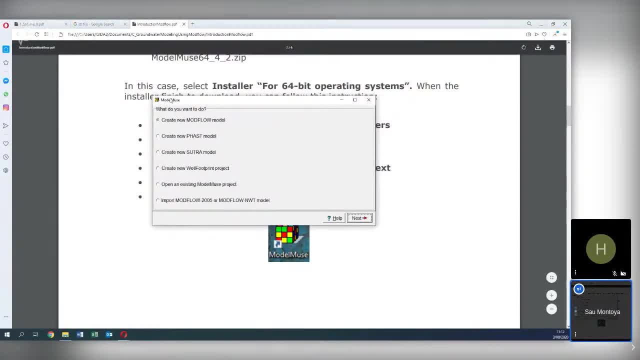 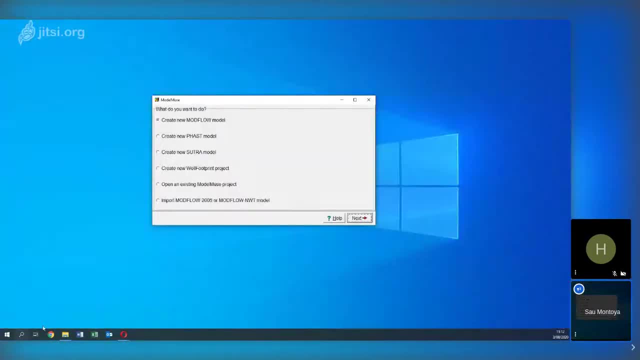 And then here, this is what disappear, okay, After I press on this, and maybe you can have it on your desktop. I don't know. No, I don't have it on my desktop. okay, But if I type ModelMuse, actually it appears here. okay. 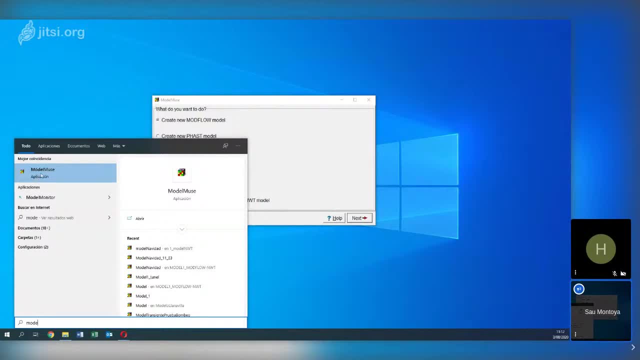 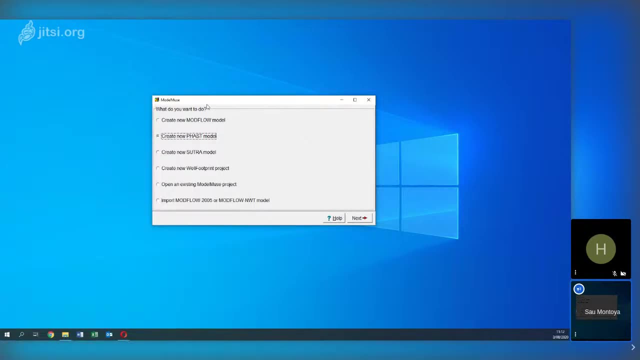 Yeah, it appears here. okay, And then you have these options. If you are here with me, type yes to. So I'll begin this thing. it will take me a minute, but you can add the options. Yes to, please. 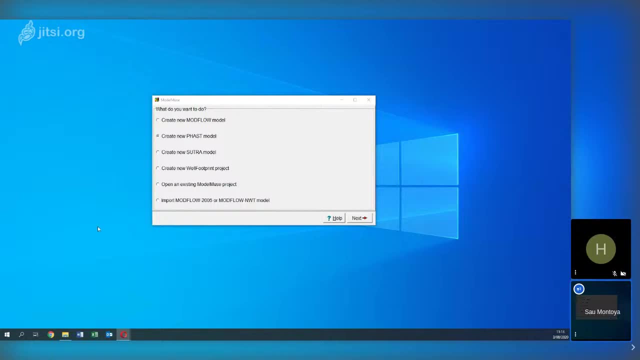 Okay, great, So I will explain what is here. okay, you, what you can do. you can create a new mode flow model. you can create and completely new model, but you can also create a fast model. what is fast model? fast model is a transport reaction model that implements another code, that is. 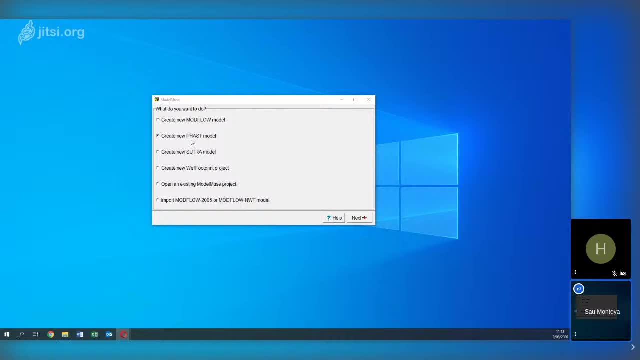 called XTD. I guess for me you have to check plus flixi. okay, so it's a transport reaction. so this model it will be required when you have, for example, a contaminant blue and this contaminant blue is actually degraded, for the contaminant species art are being associated in another chemical. 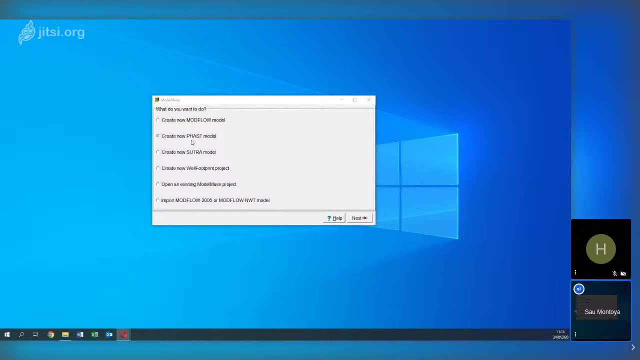 compounds: okay. so when you want to deal with that, I will strongly fast, okay. so then we have sutra. what is sutra? sutra is a mold code as well from the USGS that create finite different, finite different model. okay, finite element model: okay. so mode flow: okay, this is a. this is a kind. 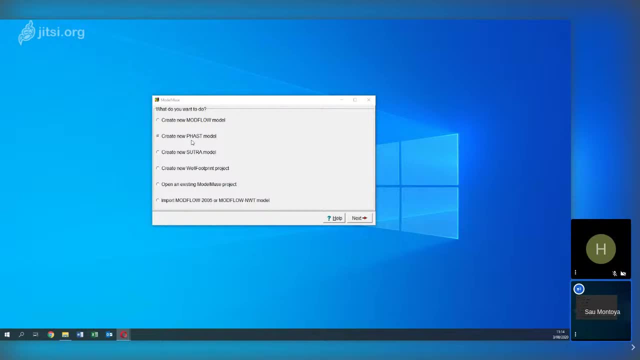 of telenovela, yeah, and it's of opera, because mode flow was finite, different model, but it was still mode flow 2005 in mode flow. in mode flow six, we have this triangular discre, we have the we can do triangular discretization, mode flow and then we can do boronoy discretisation in mode flow. 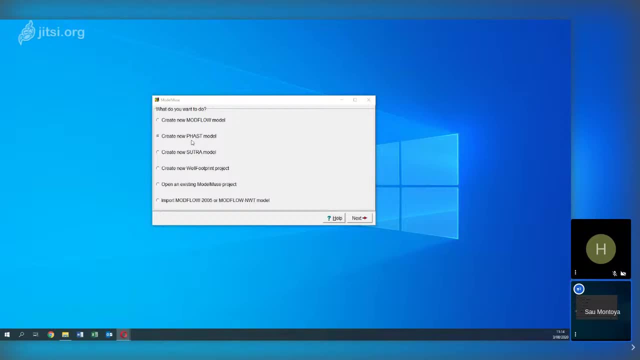 almost any discretization mode flow. okay, that was not possible in mode flow 2005, but now it's. but well, but at the time that where you have mode flow 2005, in mode flow you can create grid like jamming, regular array of rows and columns, while with sutra you can create triangular grids. 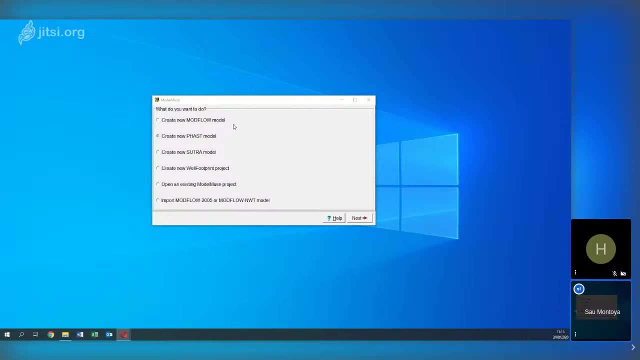 okay, but now in modflow 6 you can also do triangular grids. okay, i hope that you are not get lost. just well, i um, i want to give you as much information as possible, but also, if you have any questions, i am, i am, i watch it, i watch the chat, and so i can answer that on the spot, okay, there. 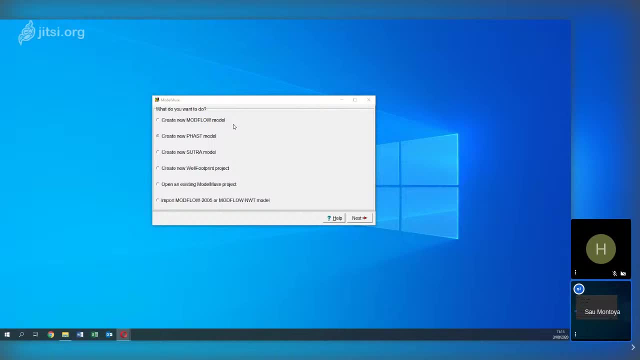 is another topic of water well footprint. well footprint is related of the capture area of wells. richard minston- that is, the developer of modern news, has a tutorial of white footprint. actually, i haven't done, i have done, i have been working in, but if you see the tutorial of richard winston, so you just have to look. 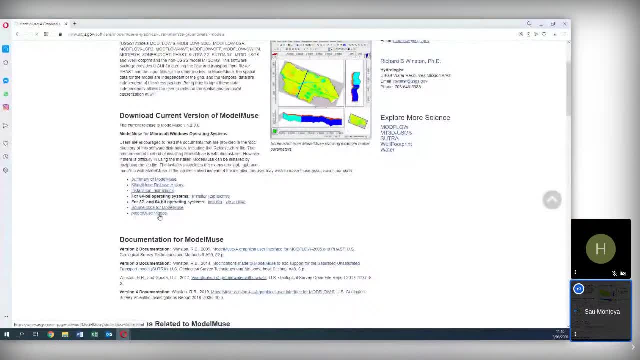 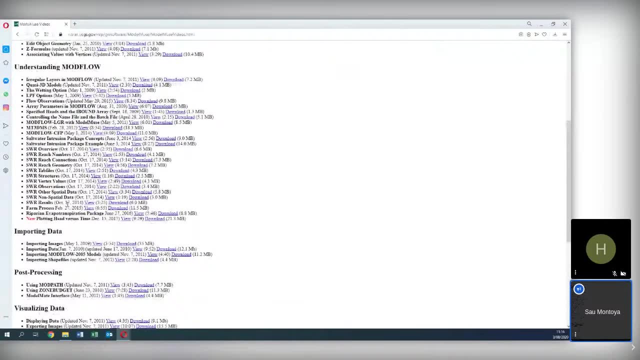 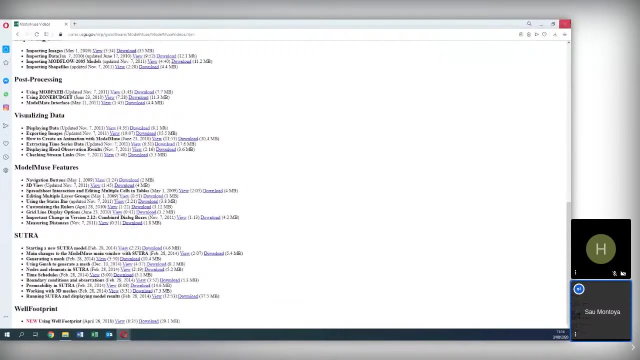 yes, there are some videos on here on modern news videos. there is a new one in: well, it's not new, i'm well. well, it's new for 2018, okay, so then, okay, if you are learning it already, you want to do consulting or research or your master thesis or something? i will strongly 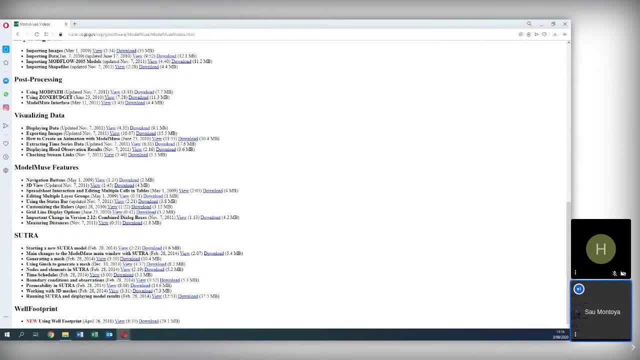 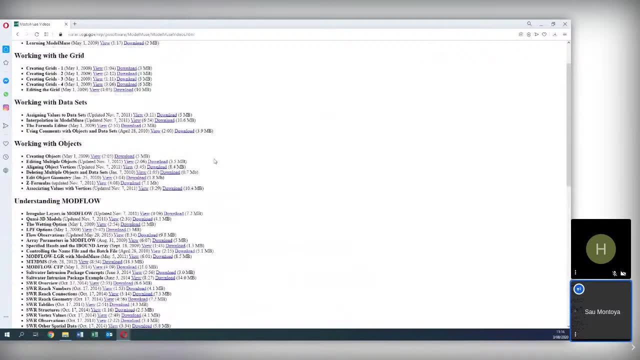 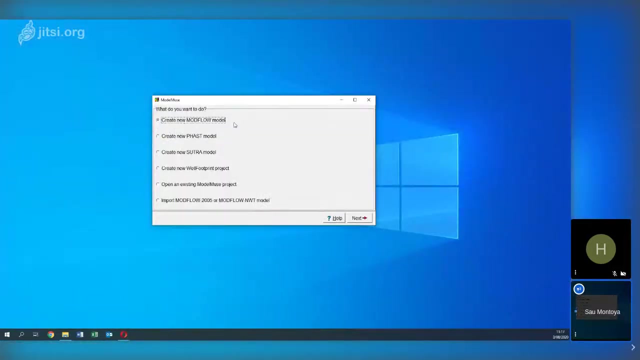 recommend as well to see, to watch these videos. okay, because these videos are really, really important if you want to know more about the software. i have watched almost all of them. okay, yeah, okay. so everybody create a new workflow model and type next, okay, okay. so if you are here, 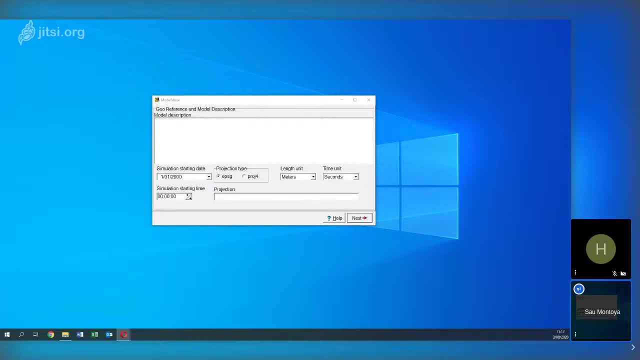 yeah, here, this is the mod flow model, so it is here, okay. so everybody create a new modflow model and type next: okay, Here this screen is almost. how can I, how can we tell you this screen is informative? only okay. And then- and I hope that you are here with me- 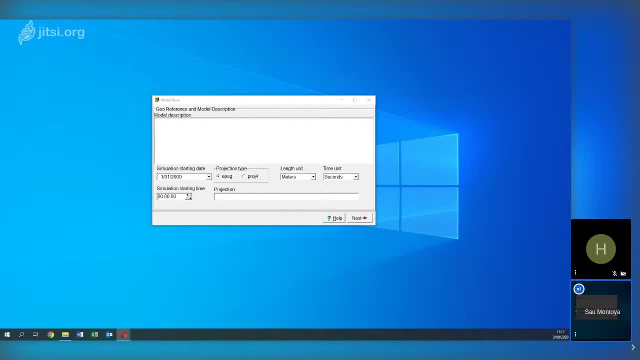 because otherwise it can be like: very okay, let's talk about the special temporal topic of model with ModFlow and model news. okay, If you work in ModFlow, ModFlow actually do not care where the model is located, because what ModFlow will care is about the grid. 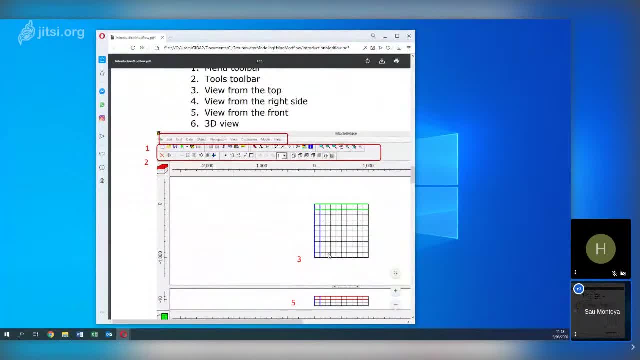 and the position of one object in the grid. okay, Wait, this is the first thing that you have to remember. Okay, So the model, actually actually for the model, a coordinate system is a coordinate system that can allow you to put any object in the grid. okay, 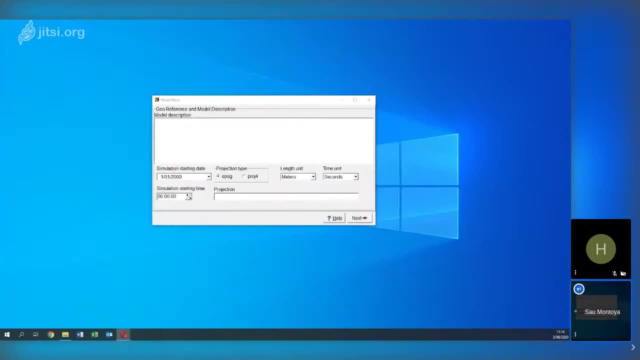 Great, But, however, what will happen if you, for example, have to do a repository of your model and then any person from here to five years have to do have to know where the model is located? okay, Because, for example, something happened. 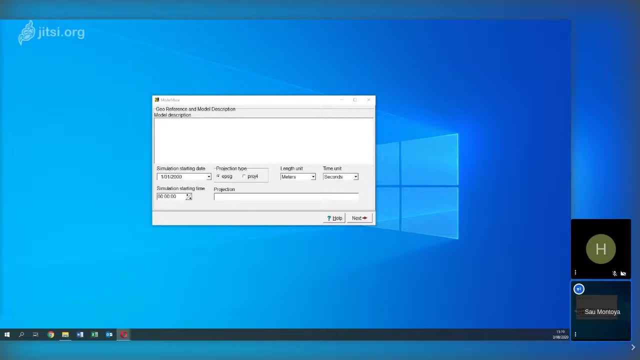 and then a guy only found a file that say model one, And then the guy say: oh, what is this, what is this? what is this model located? okay, I don't know. I mean in the period of basing. 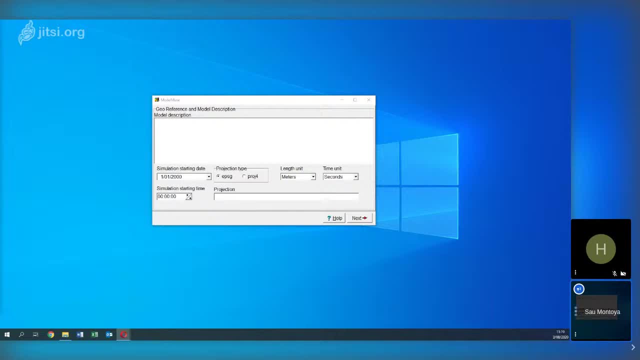 but I don't know where which basing refers to. okay, So that is why here you can. okay, So that is why here you can. okay, So that is why here you can put some metadata regarding to the system of projection. 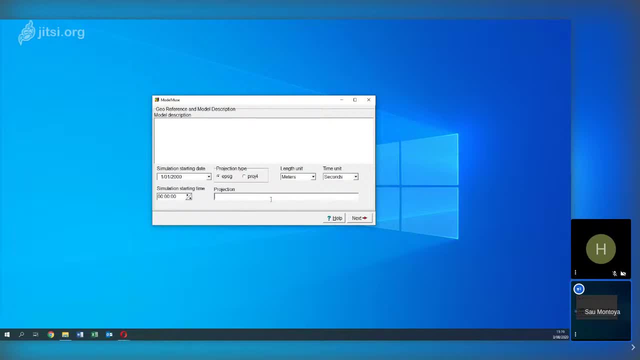 So with this system of projections, a future user or like a colleague, can locate exactly where your model is located, So it can work with EPSG on project four. but you can type, for example: here in Peru, we are in two. 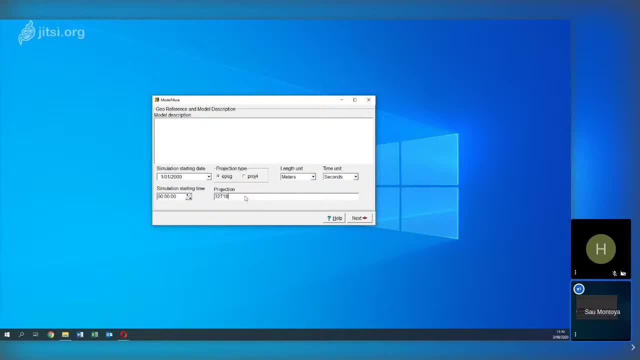 this is our EPSG code. okay, Three, two, seven, 18.. So it means three, two, that is WGS UTM, seven because we are in the south hemisphere and 18 because we are in the zone 18, yeah. 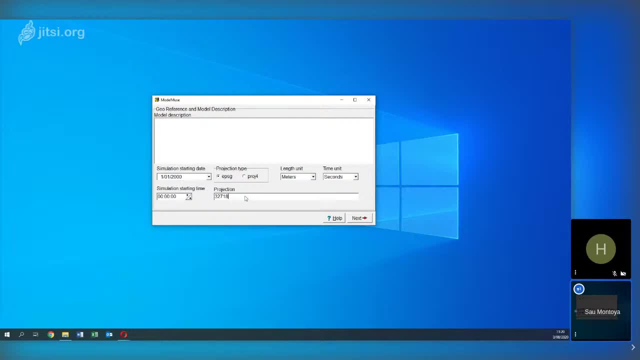 But this is only the clarity. I mean, actually, you are not required to do, you are not required to do the more during the simulation. this data won't be used in any, in any part of the simulation, or? yeah, This is just. this is just to provide the right metadata. 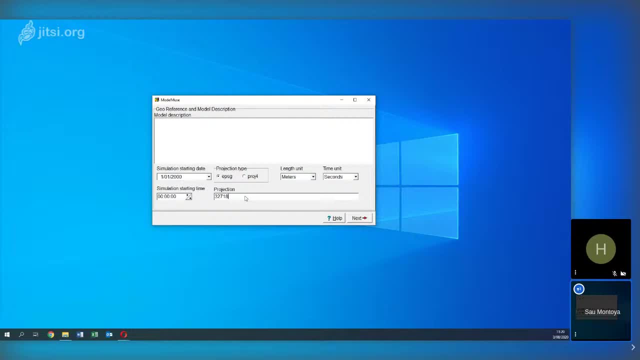 for a right interoperability of the model. okay, Great, If you are here with me, type this three: If you have any questions, you can drop your questions anytime as well. Okay, great, So you say you can put. you can. 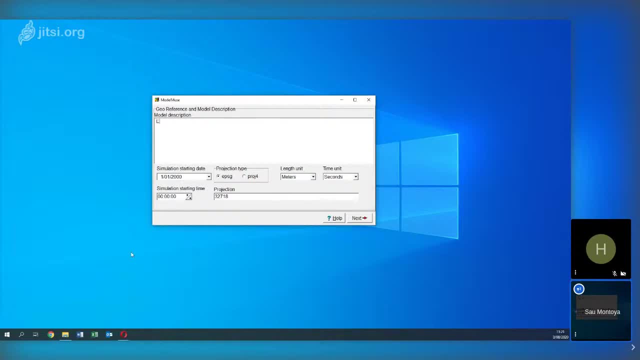 you can put, but as well, this is only the clarity. So example of task one: Okay, the starting time is as well, the clarity okay. And then you have the length units and the time units. Okay, from all of these, these are the two that 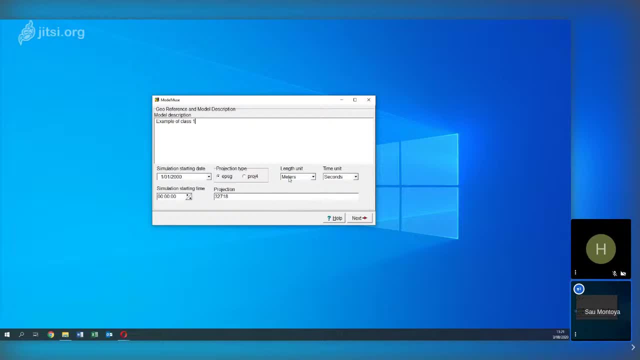 they will be used on your numerical simulation. This, these only two, will be used on the numerical simulation So you can work with meters or feet You have. since the code is done in the US, they always have these imperial, I think. system unit. 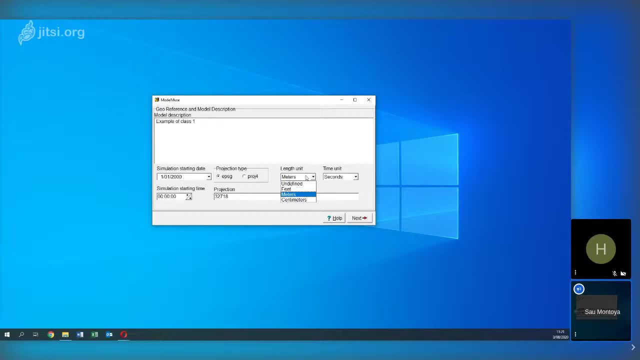 They work with feet. For us, I will strongly recommend that you use meters in the national system where the unit 한국 verrkean of length is meter And for time unit you have seconds, minutes, days and years, And this I'm kind of more flexible here. 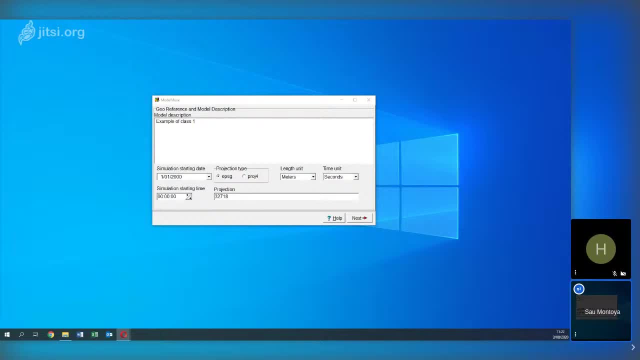 Why? Okay, there is a good question from Naga that say: how do we know the projection code for a present location? This is great, because you have to know your UTM and your system of projection and I guess, well, it really depends on the other one. 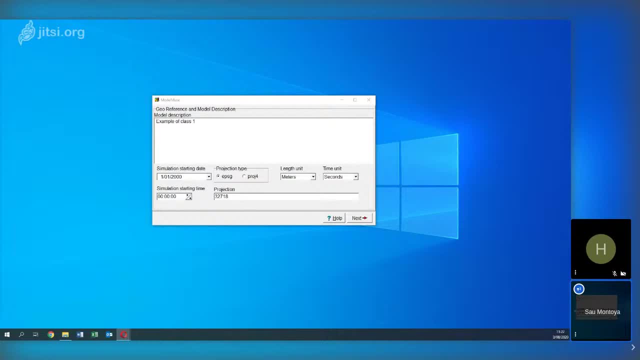 Yeah, it really depends on the country that you are. Maybe we can, later on, we can provide you some links regarding that. okay, Okay, so okay, Sometimes transmissivity is being reported in meters per day. okay, Or, like a draft, conductivity is reported in meters per day. 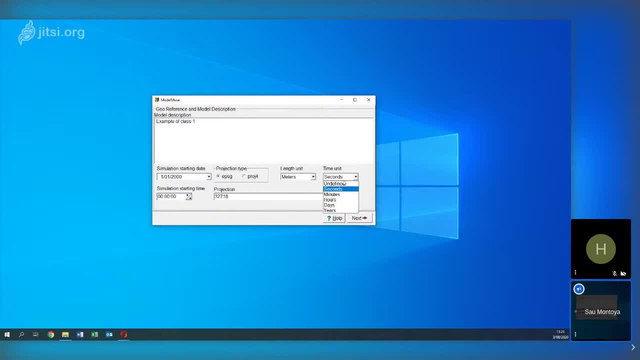 That is great, I mean. however, I use meters per second And it's really up to you to select which is your time unit, because if you work with days, you will have. it would be easier to work like transit simulation over three years, five years. 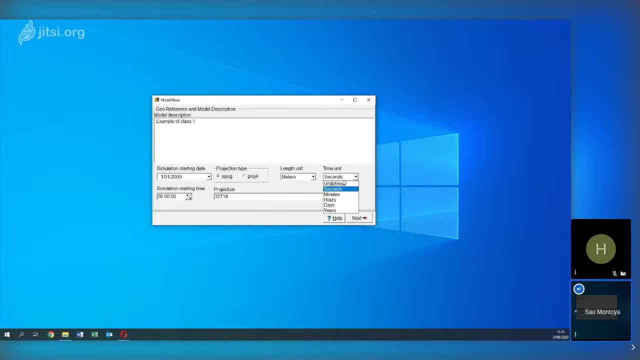 six years, six years or because they you will have a number of days, or maybe even you can work with years. what is my, my recommendation? and please, please, know that, if you're not, if you are taking notes, that if you select any type of length unit and any time of time unit, you have to translate all your data to. 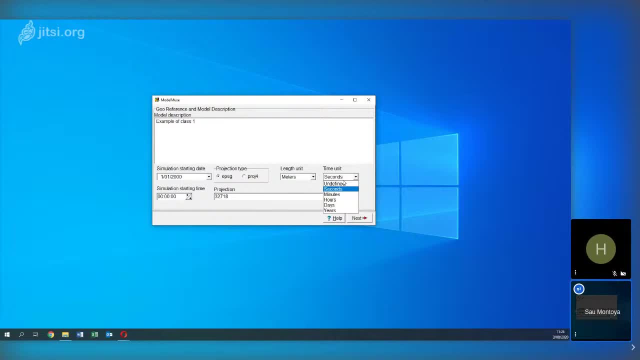 those units. okay, you have to translate all your data to those units. for example, you select the time unit two days. all your transmissivity, all your hydraulic conductivity has to be translated to these units, because I think later on there were some options to translate in model news. but 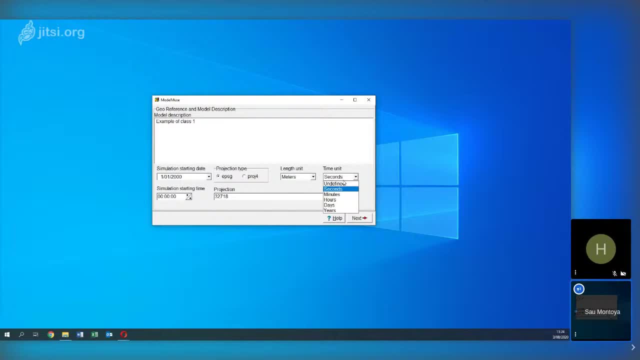 it's not that good, it's not a great quality practice, okay. so for me, as a modeler, I always relate everything to the units that I have selected to do the model. and then I start to do the model because later on you will have values and then you don't know if those values- where I mean you can get the value. but 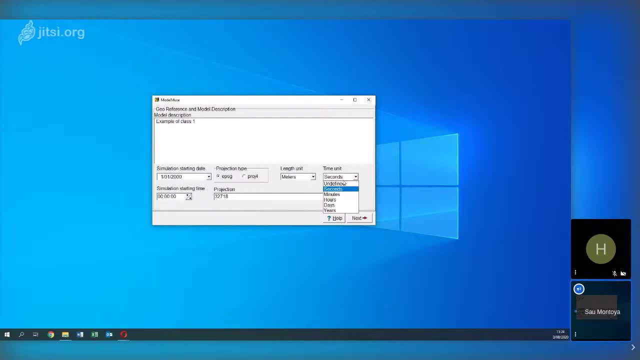 you don't know which was the time unit or the main unit of that value, okay, but, for example, if I work in meters a second, I know that all the other parameters that I have are expressed in meters second, square meters divided by second, and so okay, so in this case it's meters a second and as a my advice, if you select, 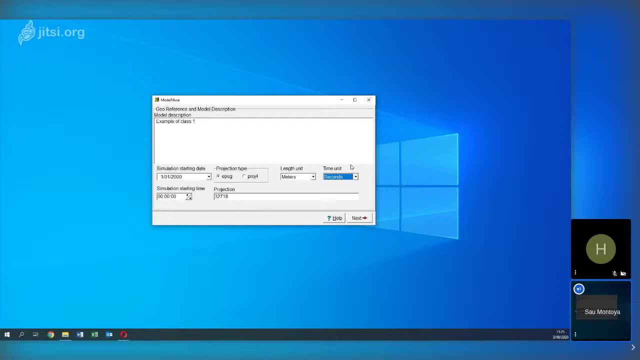 a length unit and a time unit. translate all your, all your information to those units. okay, next first break: are we here? if we are here, type yes 3, yes 4, yes 4. ok, real, here we have. we are in mother nossalauf six. ok, then we can also select. 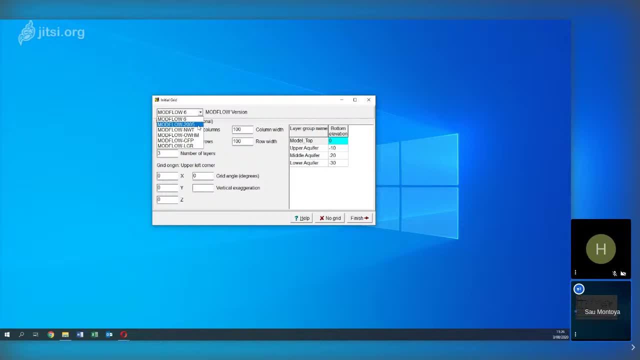 the much trabajo 2005. we can also select more flow integrity. we can also select to more slowly we do it. we can also select C in evil. lg are ok, let's have a review of what. what does mean? ok, Moffolo six is the latest version ofMo on, because 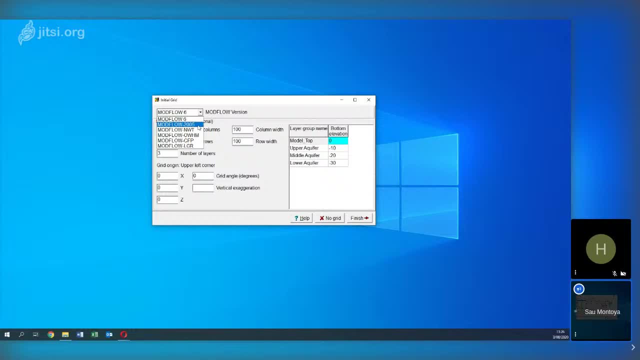 is the 6th ver. 6th ver of modflow. okay, so modflow the first version was from the 88. they become 96, then comes 2000, then they come 2005, and maybe i'm missing something. okay, so modflow 6 is the latest version of modflow. 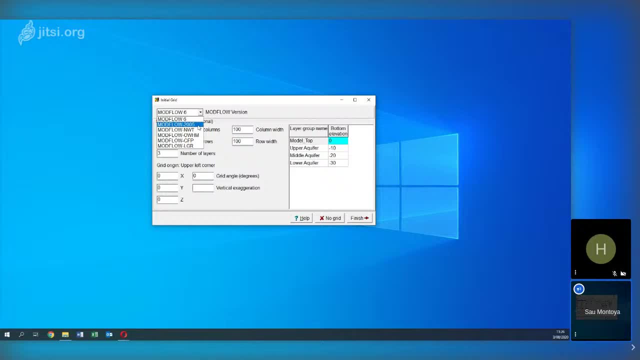 and some of the some of the tools of modflow 6 are available in model news, because model news actually do not implement the unstructured grid yet. okay, then we have modflow 2005. okay, modflow 2005 is only on- it's only on finding a different, find a different method. so i mean in 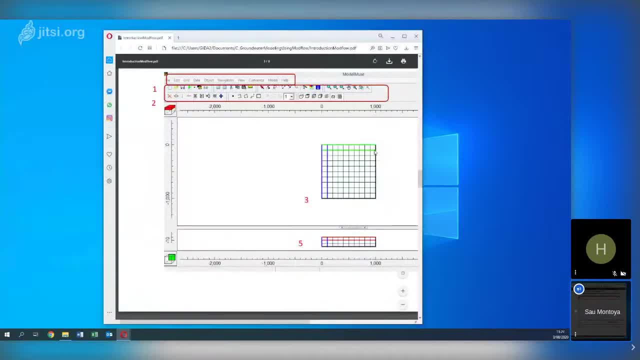 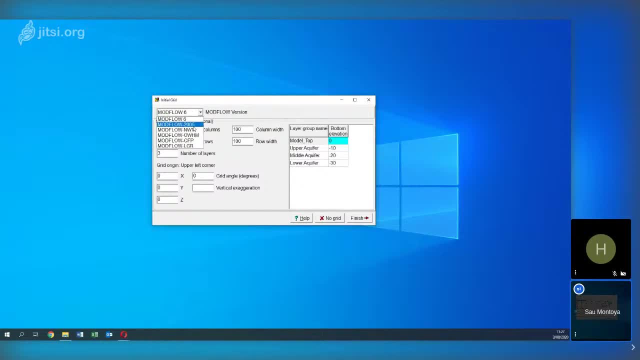 modflow 2005, you can create regular bits of raw and colors like this one. okay. however, for example, what happens to me? that if i wanted to do real modeling- i mean on the scale of basic modeling, i will, uh, of complex geometries- i could not reach the solution with modflow 2005. 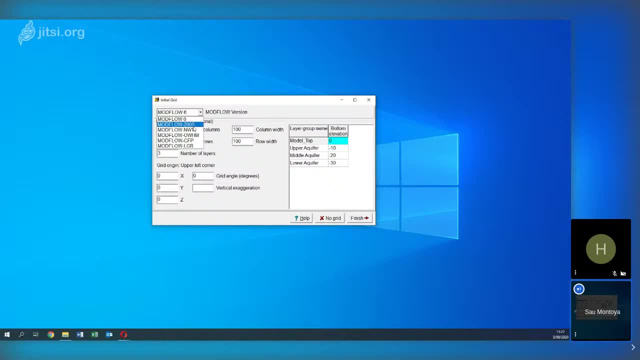 because the matrix was a kind of very intense, uh known diagonal. they have a number. because it was the, the solver could not um have a solution for the of the model. that's why it came. modflow nwt. motorinity is a newtonian solver, newton rape. 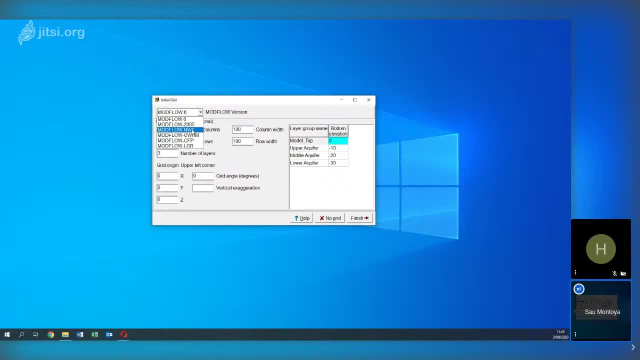 solver of the of the ground water flow. that kind is more flexible, is more flexible with complex geometries, is more flexible with dry cells. um, yeah, and we? i think that is more flexible with changes on ironic properties. so i mean, if you have a k of 1 to 10, to the minus 5 close to the 10, 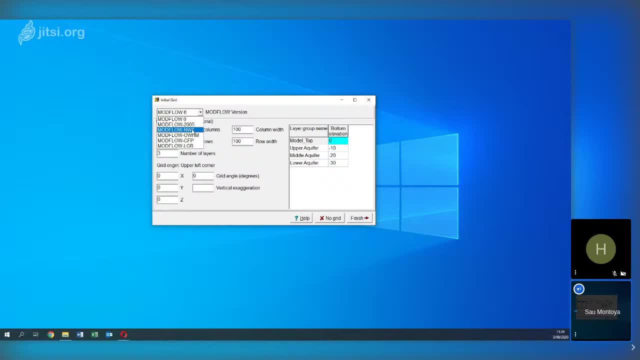 a k of 10 to the minus 3, you have to order a magnitude from one cell to the other cell and then sometimes, uh, not flowing duty, you can have better results. okay is remember: that is a solver okay and this is a solver okay and this is a really a great solver. for example, when i do 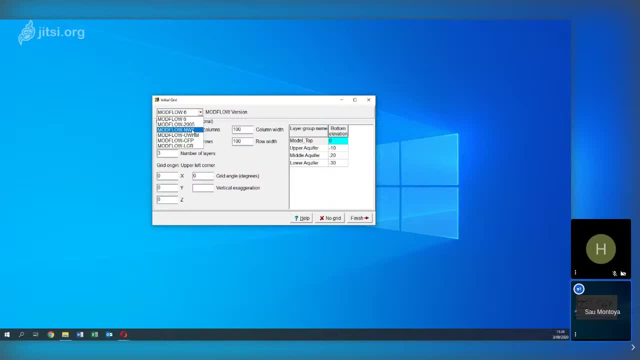 gradient modeling. i all i need for me and this is really for me. i use mod flow and duty instead of mod flow 6, because for me, what really works well, okay, i reach better solutions and i reach it in the right way. so this is a solver okay, and this is a solver okay, and this is a solver okay. 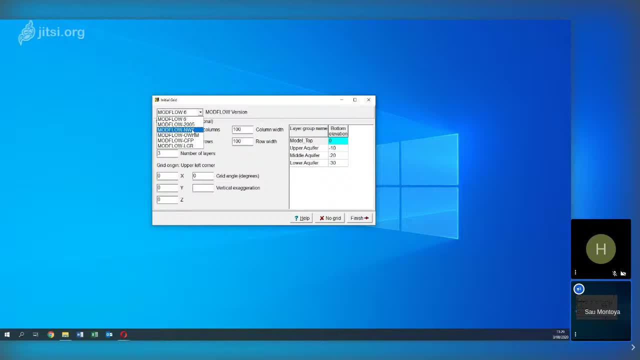 in this time. okay then, if you are planning dealing with, for example, if you have a basin that is under high stress and then you have a model that can diagnose the basin in real time, considering, uh, irrigation, pumping, transportation losses on channels and so on, i will strongly 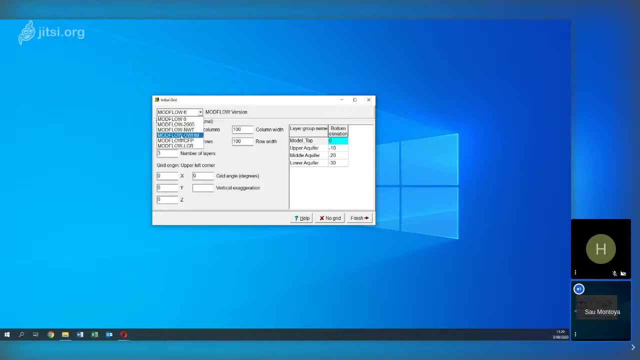 recommend to you the oil to hm. one water ecological model. okay, that is a model that represent most of the with higher complexity. what happens on the on uh as a value scale? okay, there are few models actually done in this code. okay, for example, there are more going in this code for some stress aquifers in the us. okay, in malbuquerque and. 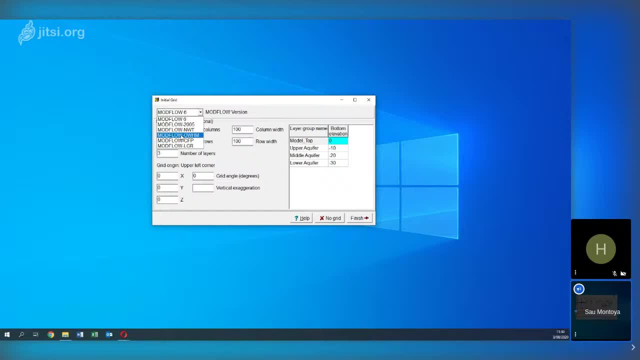 california. they have this model gone and they have sometimes they have this model connected to um, to a website, where, in the website, you can have the diagnose of the water levels and then you can apply some sustainable, some groundwater policies that, no, that say, do not pump if you. 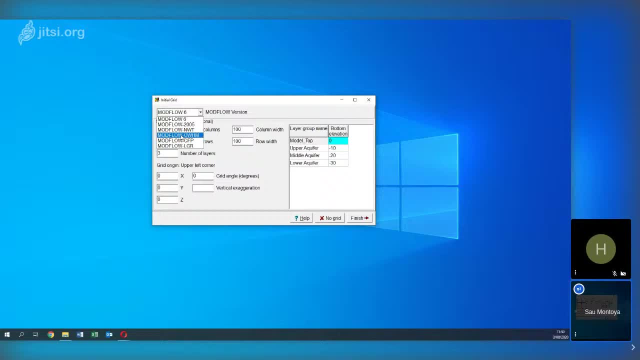 are under this level. so, yeah, the concept is is: it's great, and then you face some governability issues and you can do that with our new hm model, okay, great. and then we have the cfp. the cfp model is related when you have to, when you need to. 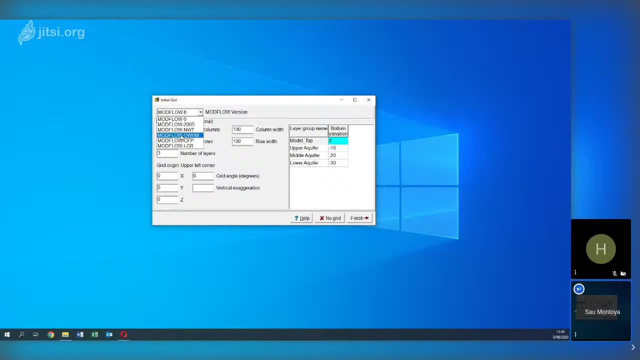 work with um fluid process, for example. okay, and what is the? what is the topic here? in moth flow, i mean in modflow, in a numerical model in a ground water following system like this, it is assumed that the flow is laminar. okay, so you have a. flow. alongside the spaces in the pores, I mean in the spaces on the pole. you have your groundwater flow, okay, but what will happen if you have a tunnel, or what will happen if you have a karstic conduit? then if you have a tunnel or if you have, 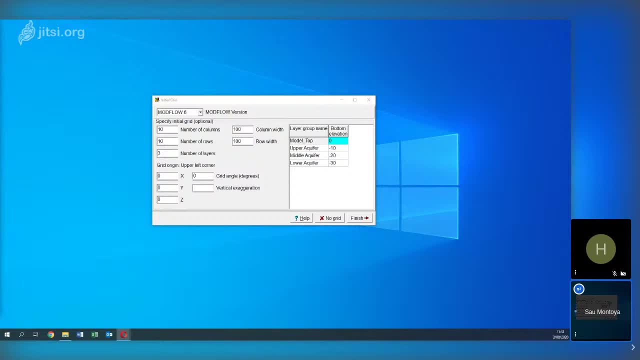 a karstic conduit, those flow there will be turbulent. okay, because you, they might be turbulent because we will read water will reach higher velocities, okay. so, Darcy, actually do not work with turbulent flow. Darcy, work only for laminar flow. is an impact, an approach on the laminar flow conditions? okay. so if 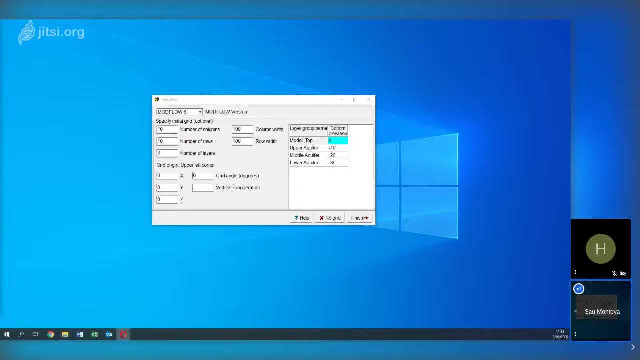 you want to work together with a tunnel or with a karstic conduit, together with the groundwater flow, I will strongly recommend to use mudflow CF. okay, and then if you want to do a local, a local grid refinement, this can be done better in mudflow 6, but if you want to do it with mudflow 2005, you can use this. 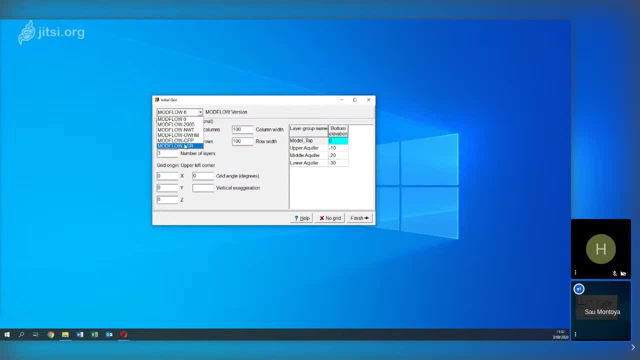 okay, if you are here with me, type yes 5 and if you need to do, you can use this. okay, this. I need to create at least my text on your screen last minute. how to work without's? I want to make sure that I'm staying on track. just Salem guys and then in the 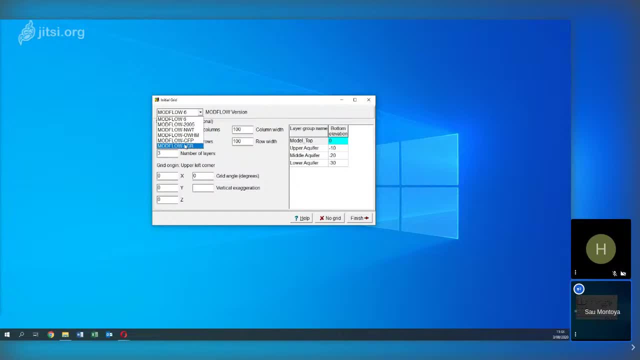 Holden bag. very simple, I'll show you how to do. okay for you, the en Freddy sure una vestida. and again, it's quite complicated. I'm going to go all the way. we are connecting and I think that what will not become up in your can dive the CV while You're connecting. it will be nice to. 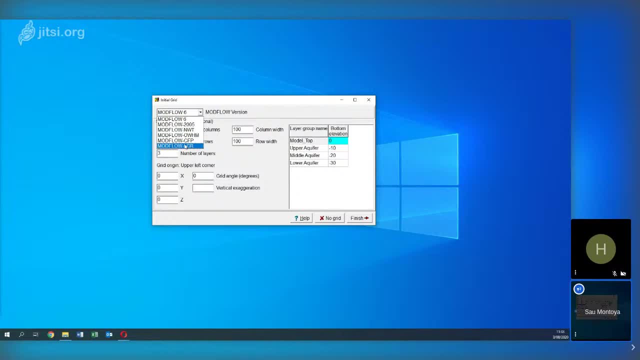 keep. yeah, let's do that. let's type hello and the city from where you are connected so I can see how. how is hello in your native language, in your native? let's type hello in your native language and the city where you are connected so I can know more about. 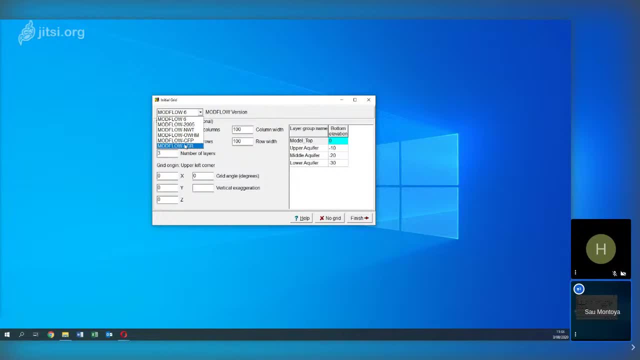 your, your language and where you are connected. okay, so here let's type: 20 columns, 30 rows, 30 columns, 30 rows, two layers of 50 and 50, and this will be- and this will be really not like- this will be called 100, and then we are going to have 40 meters of of science, or will be. 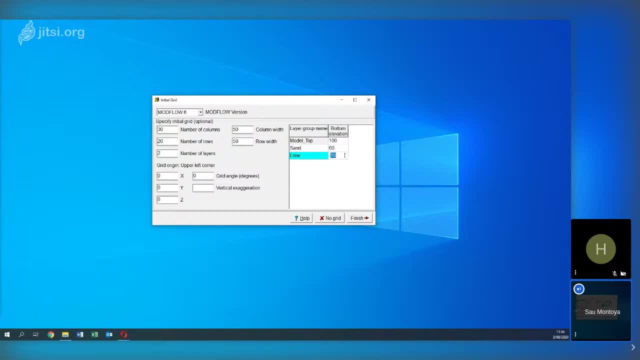 60 and it will be. we will have 50. okay, let's see. from Nicaragua, from hello with Rotterdam, hello from South Africa, wow, uh, I'm really sorry. I wish I like I can. I can speak Arabic, but I think that there are some conversation that I do not get um. 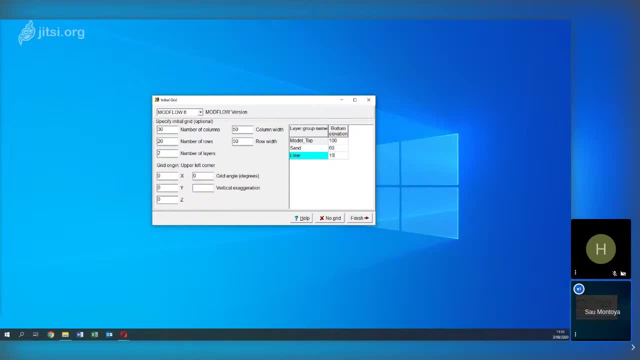 um, tanzania, South Africa. wow, great to give this. you are the most rich audience that I have, demographically rich audience that I have given any course, okay, okay. and there is a great question from Amali that say: what is the set of criteria? do you consider when? 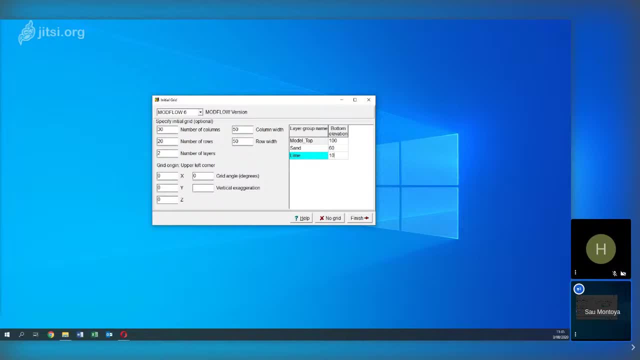 specifying the initial grid grade quest, for example. this is this I mean then when you define the grids. I mean when you define the extension is mostly for the first model. that you're going to do so is for a local model, and so on. later on you have this no grid option. do not press it, but 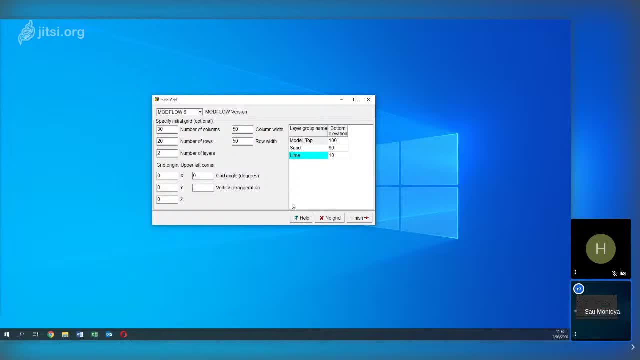 later on, when you see apply cases, you will use shell files and the shell files actually define the grid. okay, but since we are doing at the beginning, we only define the grid by ourselves, which is the criteria to define the grid there is. this is a strong question, very interesting why? because the size of the 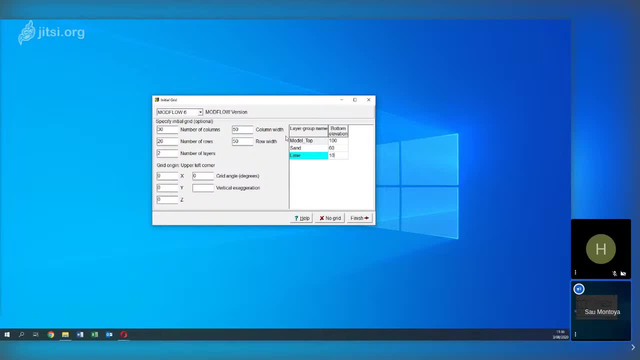 criteria is kind of custom engineering. ok, for example, if you have a facing, somebody told, somebody can tell you: oh, you have to model these on a, we jeopardize our видим, because that will bring you, that will bring you resolution. and they say, okay, that's right, you can have your facing on a grid of 1 meter by meter. 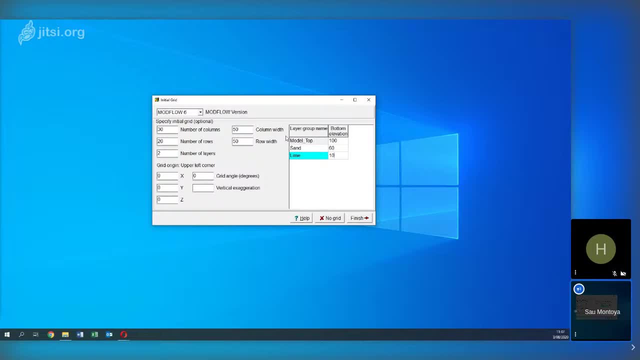 one meter. however, there is the computational, the computation. you have to take into account the computational report resources. okay, the even model views is not designed to work, for example, with grids of 1000 columns and one thousand rows, because actually the graphic user interface- and and i have tried- will be all blocked, it will be all crossing, which is the word of that one. 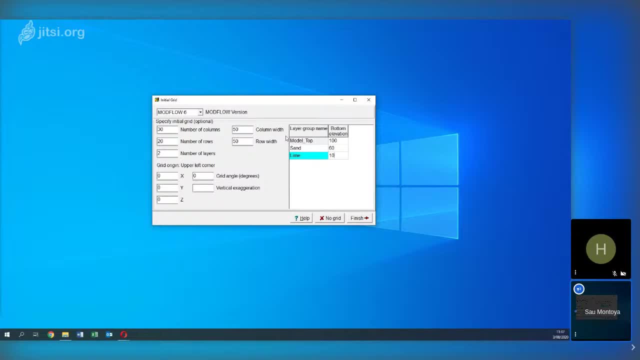 when you have it all together and very tight among each other. okay, yeah, you will have it like this. okay, and, for example, you cannot have indefinite layers. why? because, as well you will have, um, you will have an, a model with a large number of cells. okay, so, actually, the grid, cell size. 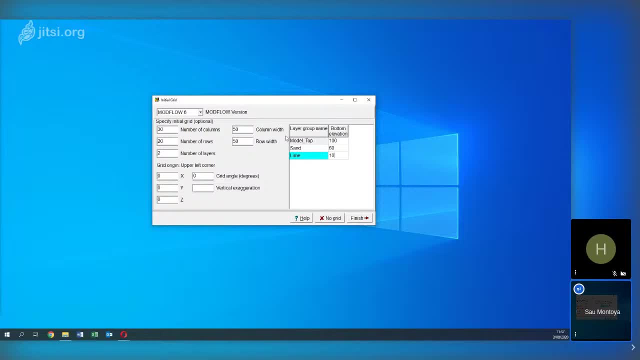 is defined. i mean the grid cell size is defined in order that you have an adequate number of cells. for me, in my experience, a number of cells of 500 000- okay, if you are doing a, a model, you have 500 000 cells. is is right. i mean you don't. i mean if you can do it. 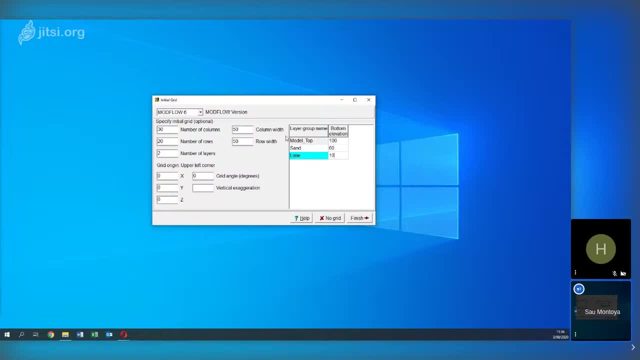 with less cells is better, but if you have 500 000 cells- yeah, the model news can work with that- you can work with one million cells, but then you will see that all the steps actually became to require lots of time, so the workflow is really slow. yeah, i have also worked with one million cells. 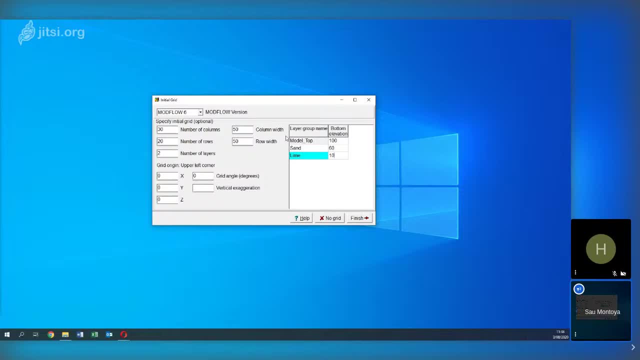 once. okay, but i won't try. i want, and i won't do any model that will be higher than one million cell and i i don't even recommend to do any model at least above 500 000 cells. okay, then there is another. there is a model where i was working with many cells, around 700 000 cells. 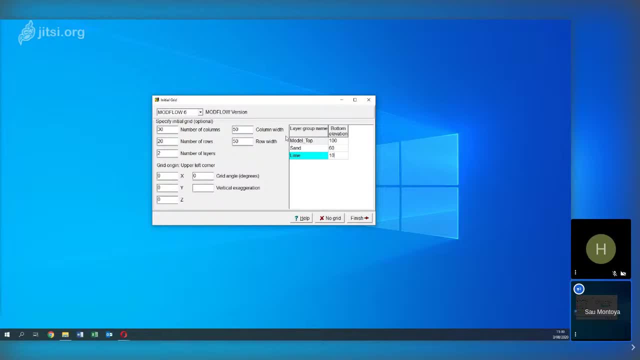 but i haven't done that in modern news, i haven't done that in in flow by python and i have um. i was really, really aware of the resources and i, i, i kept the um and i did it in linux okay, because i wanted all the the power to be dedicated to this process, okay. 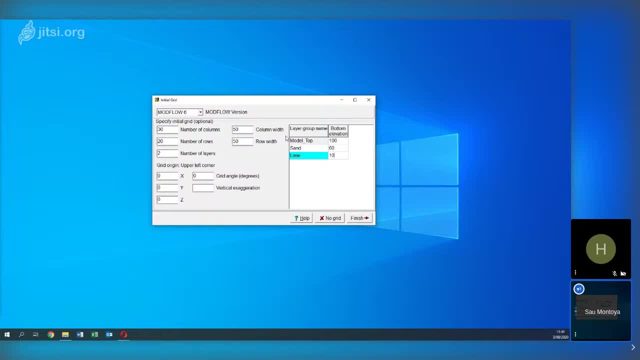 so i hope that this answers your question. okay, so here, um, this is um, this is something good, because you have to remember that in numerical modeling and in that, and as будем Haller models, you don't, you don't define the layer thickness, the lady, the layer thickness is defined. 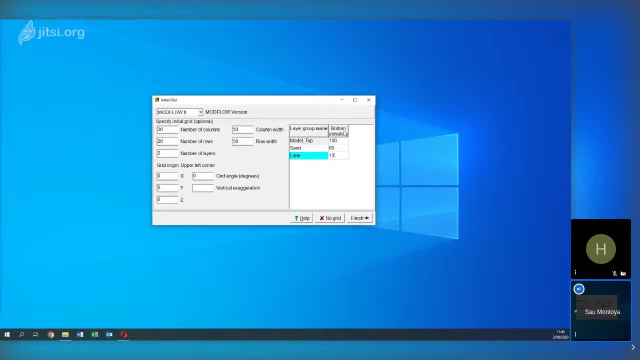 by the interface among the top of the layer and the bottom of the layer. so this is the top, this is model top, multi top, um. it appears on um and with the great background, because model top is available. model muse: okay, and this model top with capital m and capital g and underscore: okay, model top. 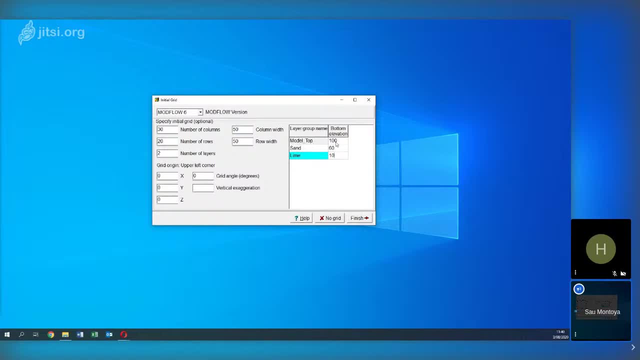 reflects the surface, and the surface in this case is 100 meters. and then it appears the bottom elevation of the first layer. the first layer for us will be sand, and this sand will be the bottom elevation will is 60 meters. so then tell me on the chart which will be the thickness of the layer. 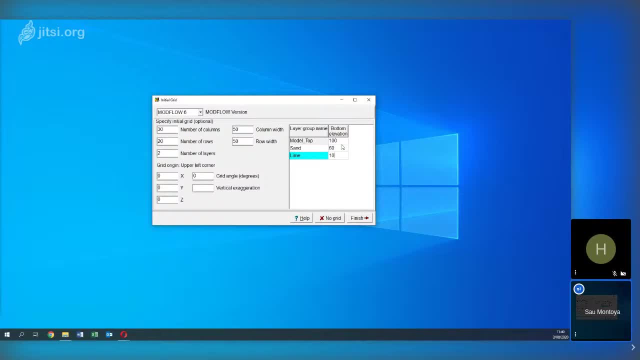 okay, on the chart please write which is the thickness of the layer. okay, great is bored. so you have 40 after the emptiness. okay, then we have the thickness, so you can have for the after the thickness. okay, then we have the line and the bottom of the line is thin. okay, so tell me which is the if, the. 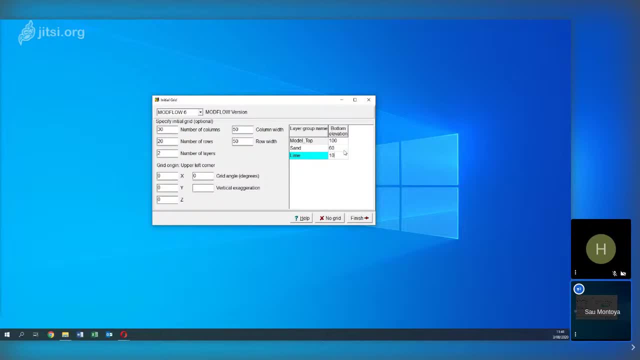 bottom of the sand was 60, and if the bottom of the line layer is thin and the sand is above the line layer, which is the thickness of our line layer, okay, 50, great. so this is how you define the layer thickness: by defining the top and. 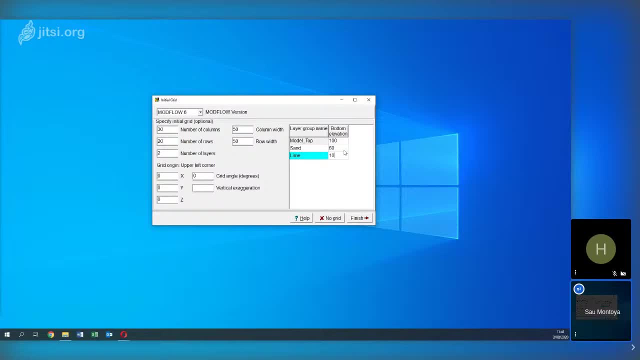 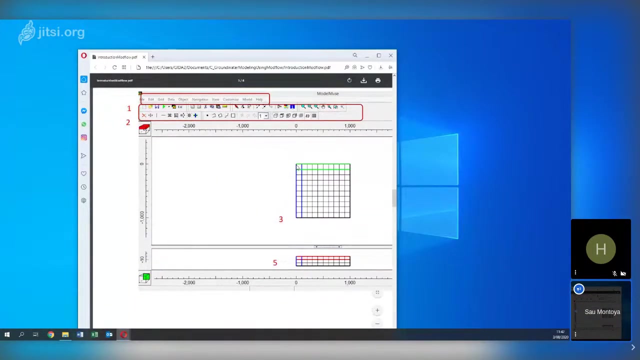 the bottom. okay, great. so with that, this is to define the onion of the upper left corner. so, and what is it? only on the lateral left corner, because, since this is- this is not Captain Sun, this is something is working matrix. everything is done from this point, because rows, I mean rows, this is 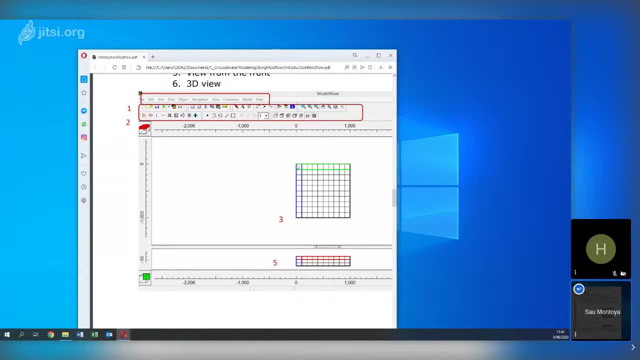 the first row, second row, third row, fourth row, and this is the column first column, second column, third column. so actually you have to define this. this will be your zero. that is not the same as the geospatial zero origin, because this is the geospatial origin, but for the matrix. 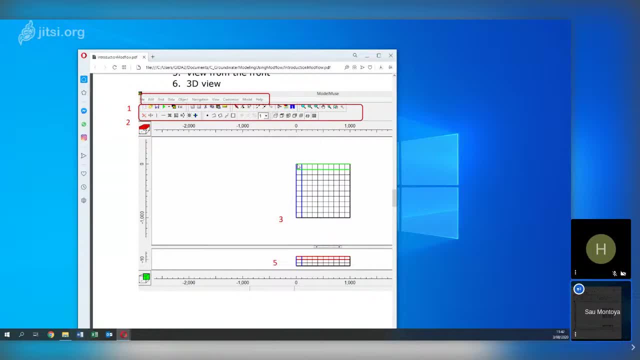 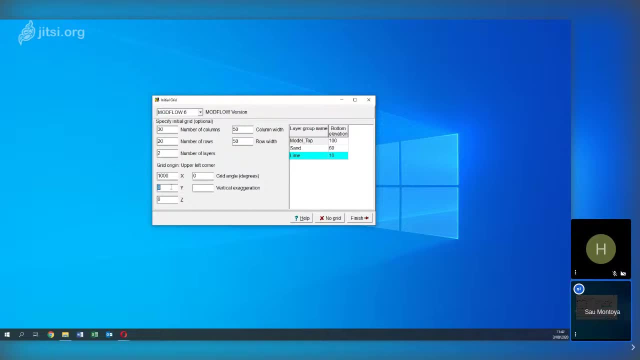 this is. it is the row, this is the origin. okay, so in our case will be 1,000.. 1,100- okay, if you are here with me, type finish and write on the chat: yes, 60- okay, if you are here with me, press finish. 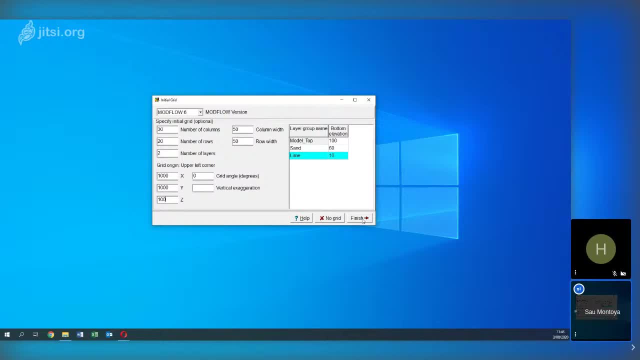 and type on the chat: 60, yes, six. okay, I have questions. should we take layers from the ball hole or your technical data? sure, sure you can have. you can insert all your geological model and there are tutorial for that. okay, but these are, Jose, if you are easy. it's like. 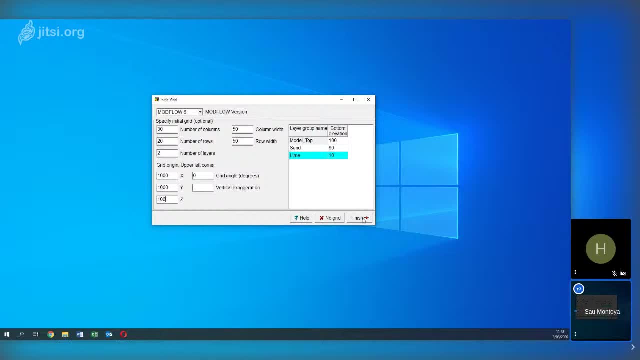 kind of doing the tour de france, if you have not managed to learn how to write a bicycle, okay. then Tahira asked: that's love helps here, for fine, yes, sure, sure, I mean there are. there are tutorials about how to implement geological models in multiple, okay, but the procedure is much advanced and is different. for that, okay. 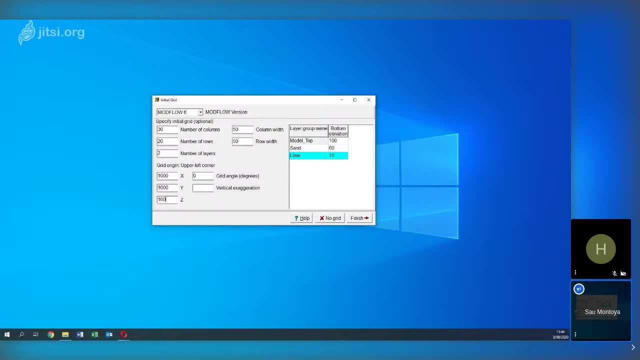 this is a simple model where everybody has his first step. in America, mine, okay, there is a. what is significant, this is the size of the of the column and this is the cell size and we will see on the degree and what if I area difference, difference for the segments. okay, this as well, please. this is very 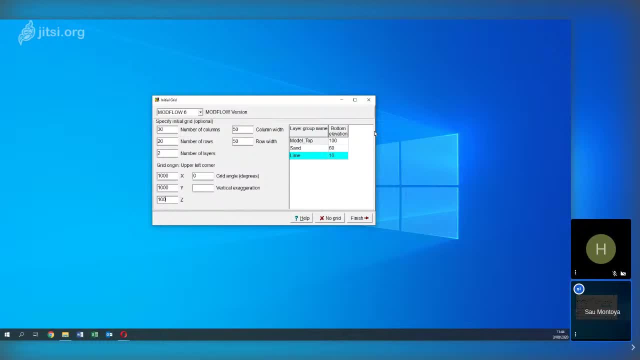 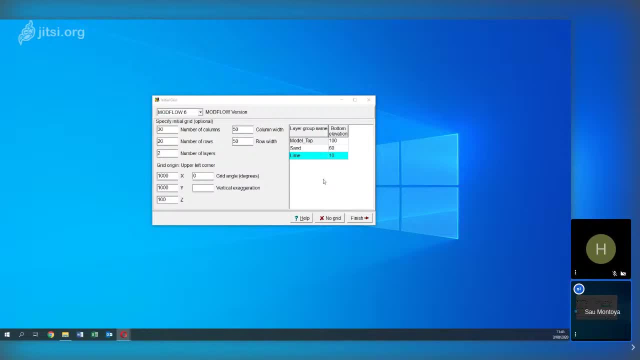 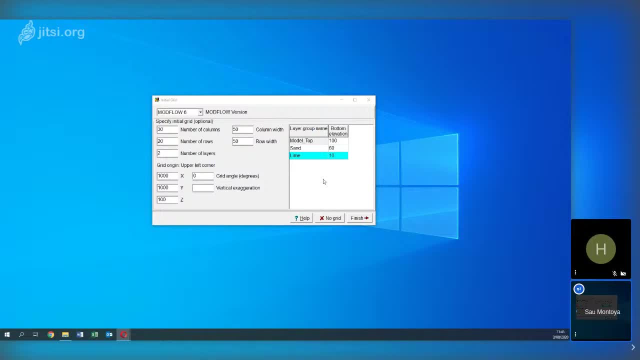 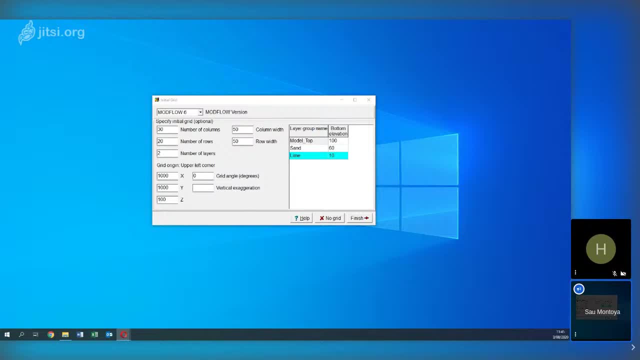 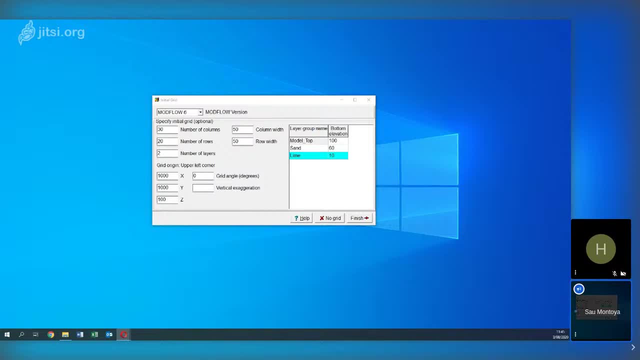 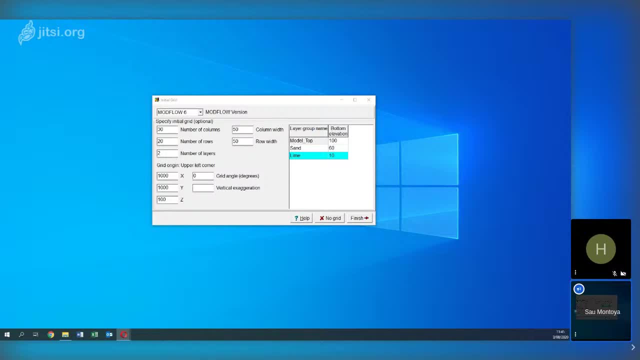 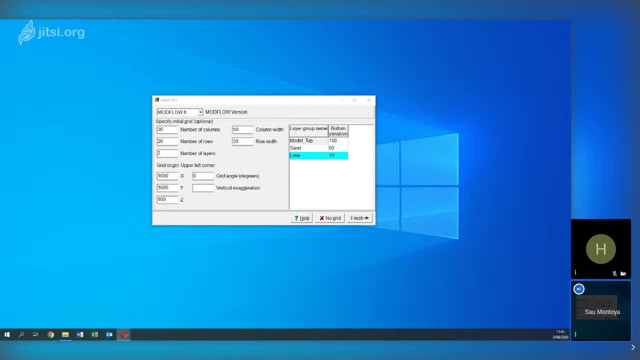 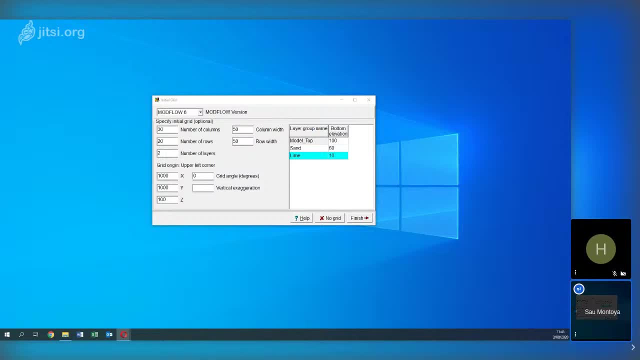 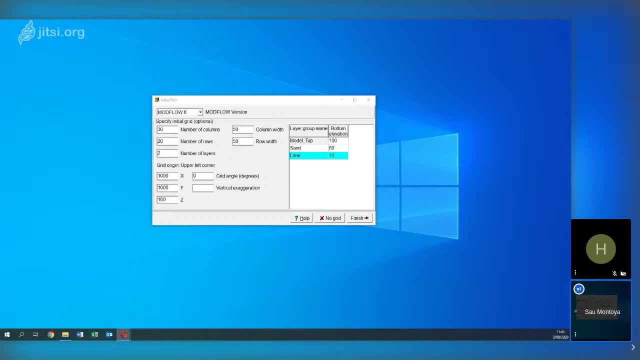 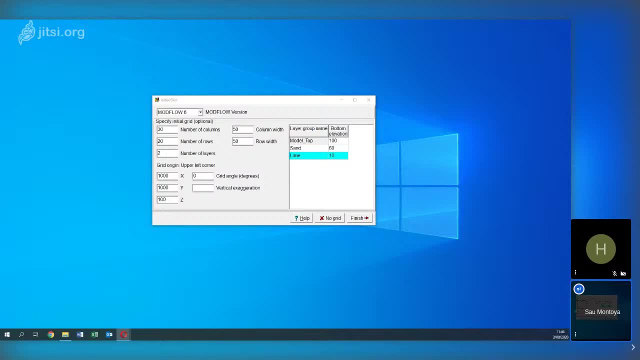 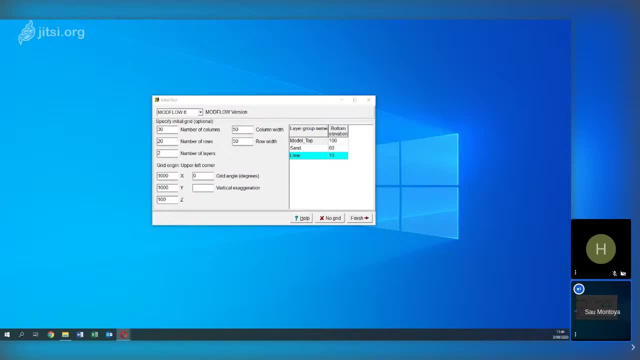 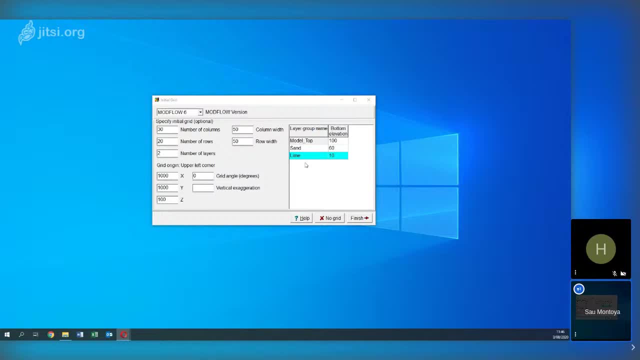 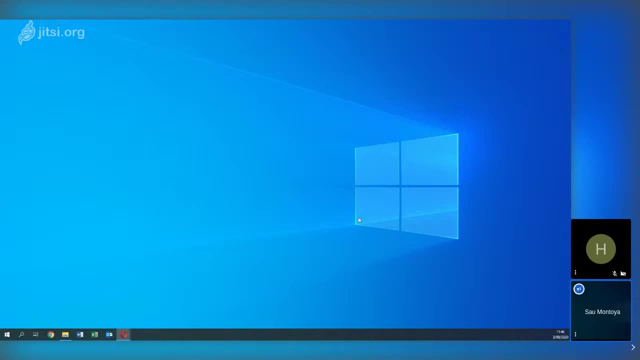 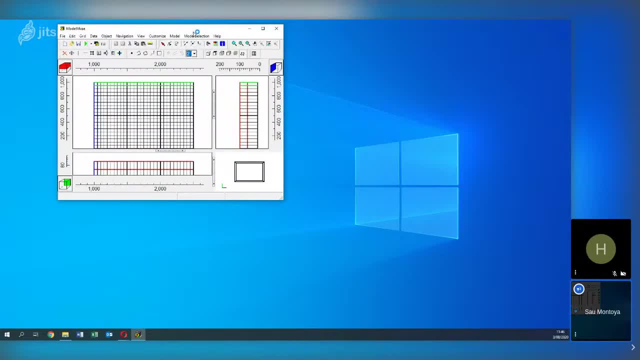 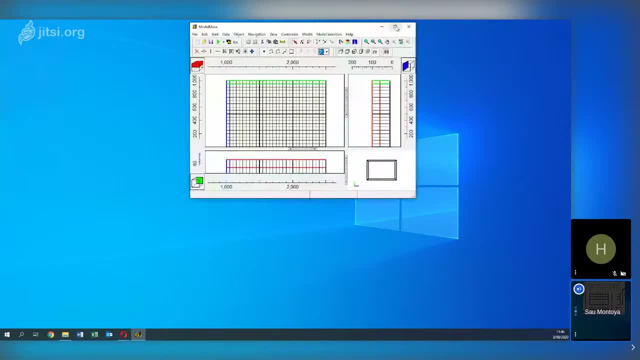 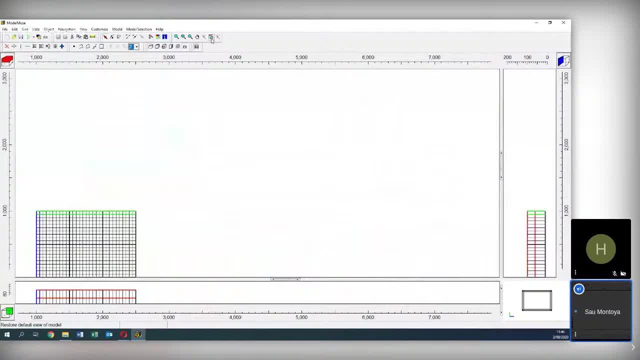 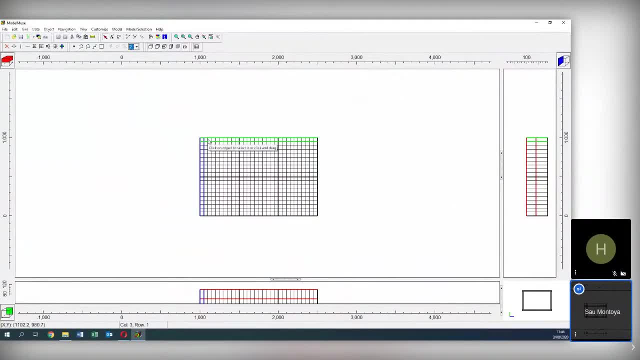 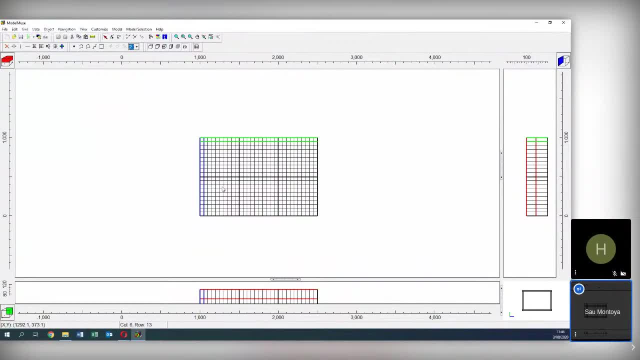 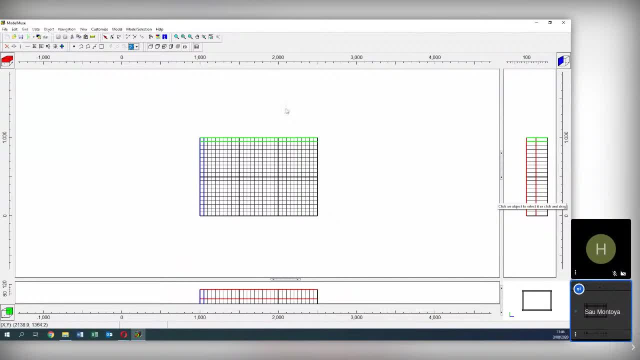 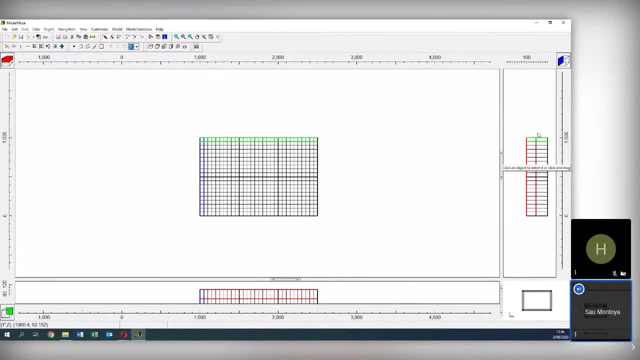 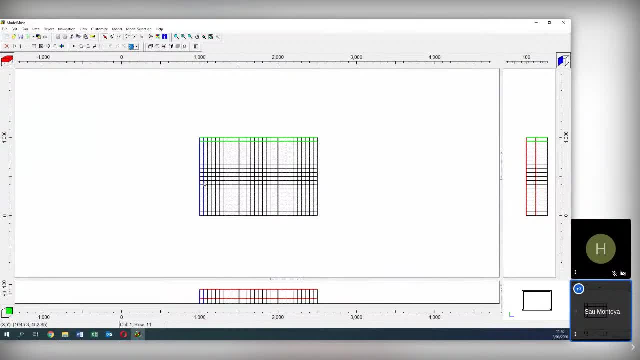 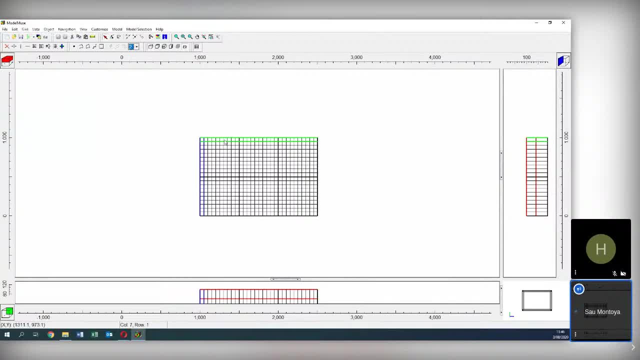 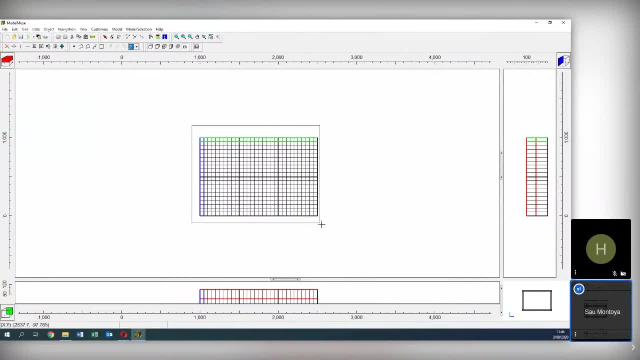 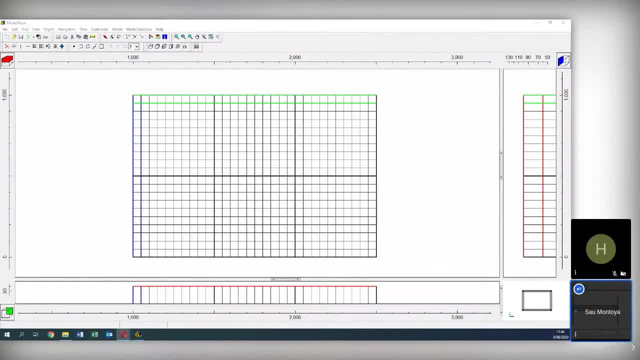 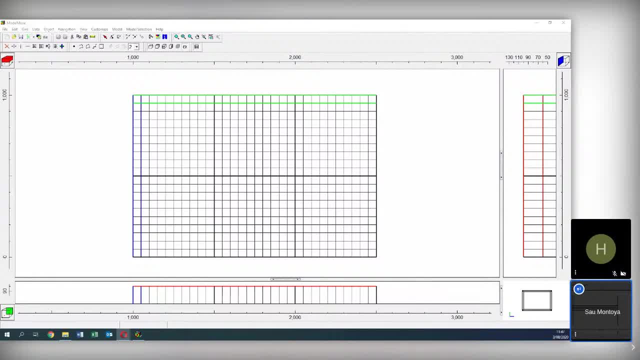 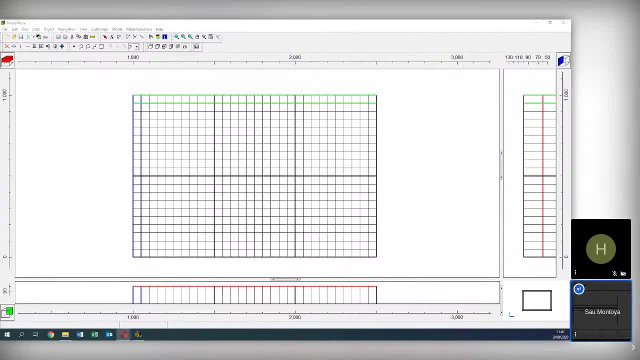 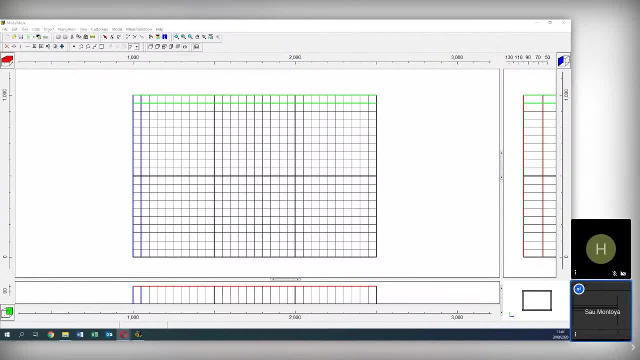 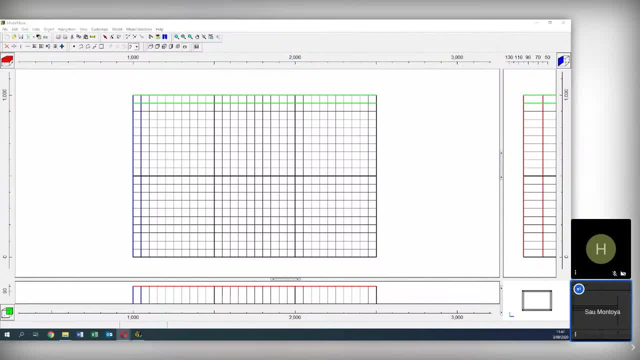 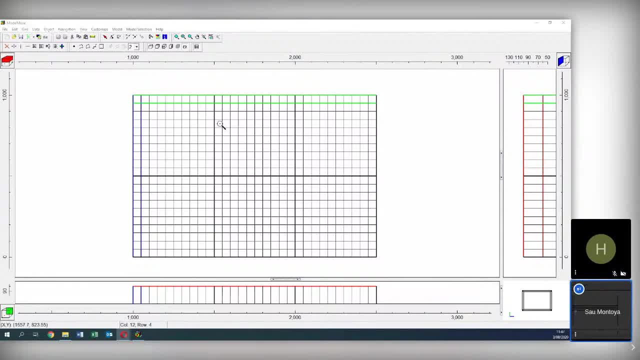 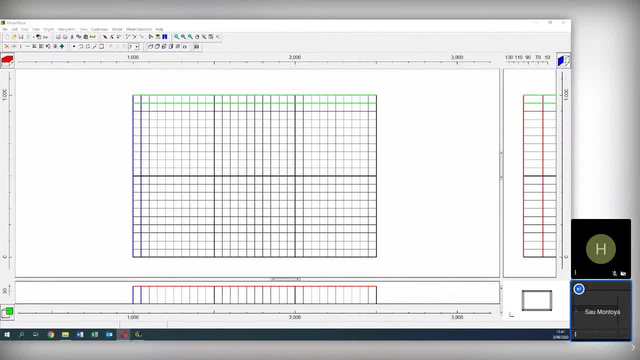 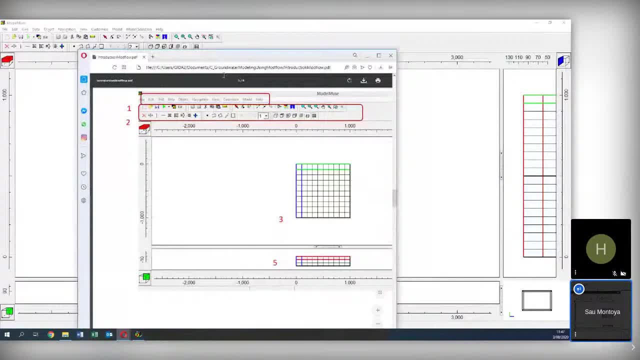 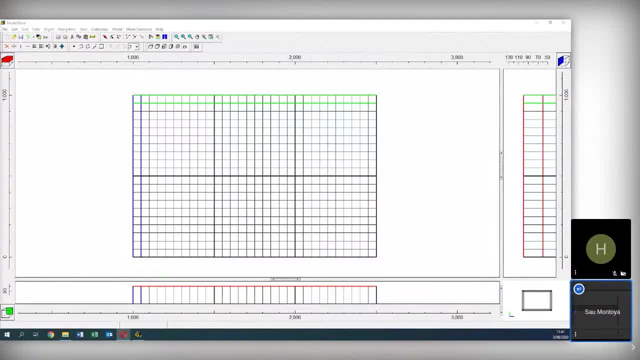 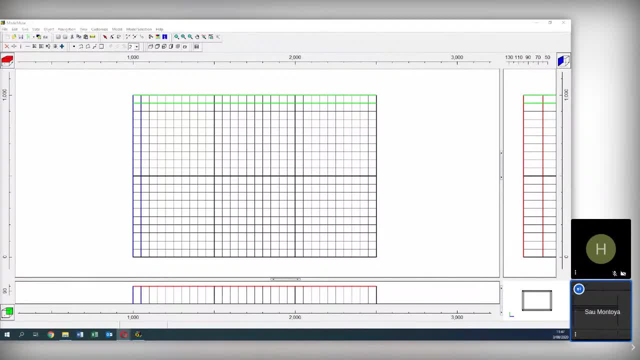 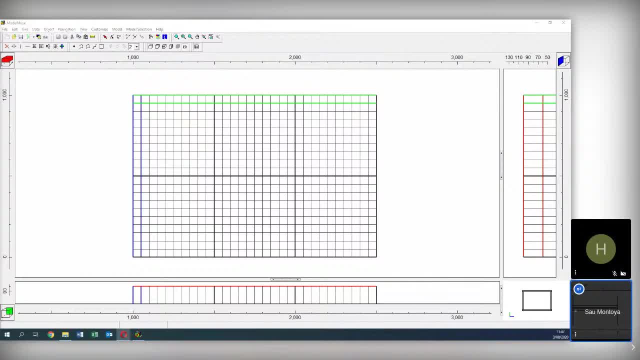 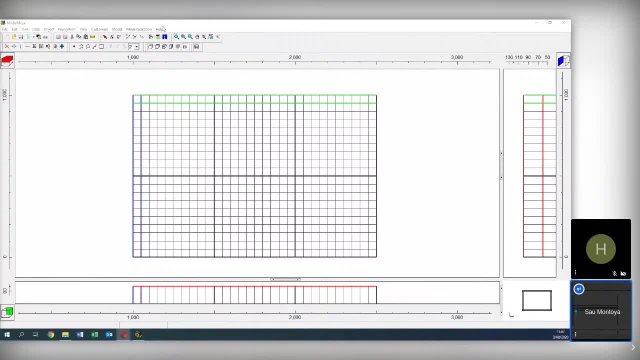 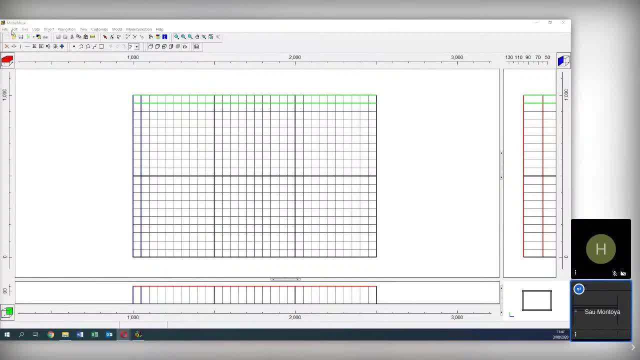 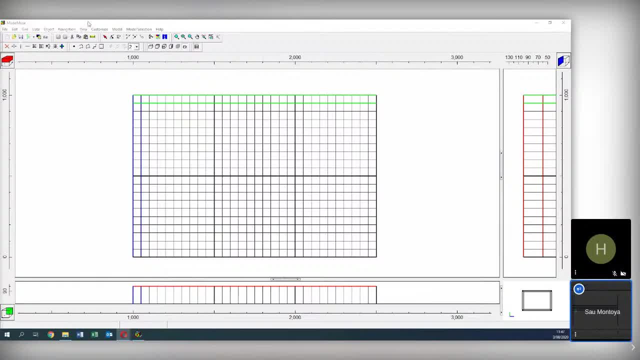 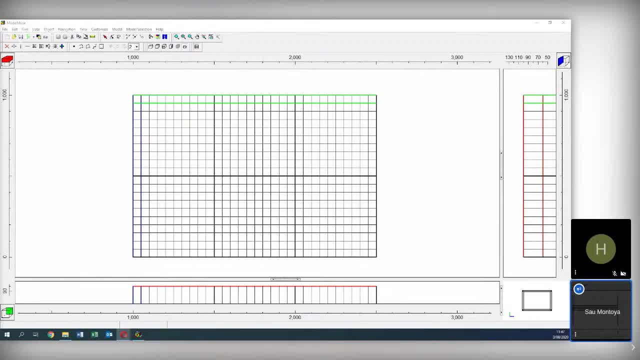 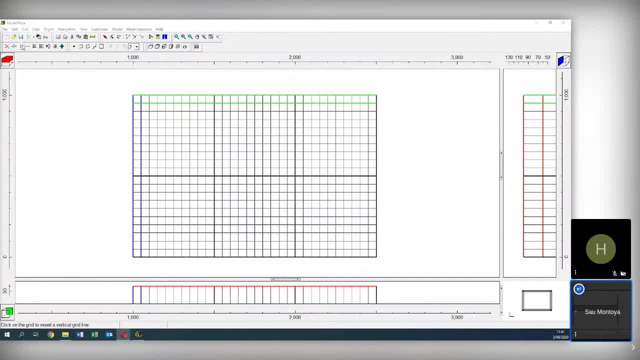 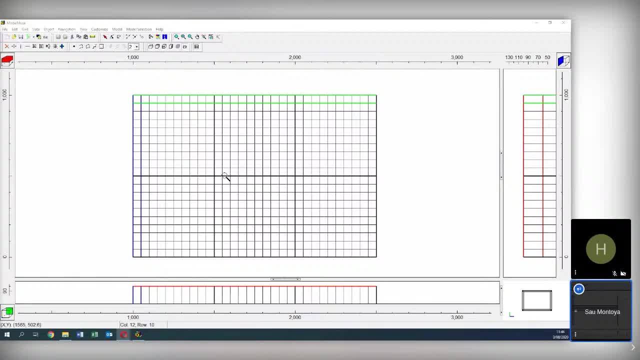 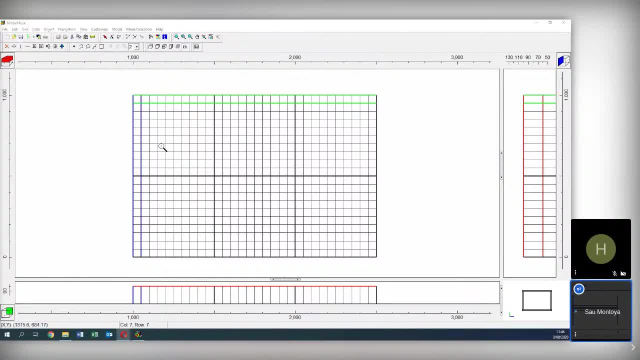 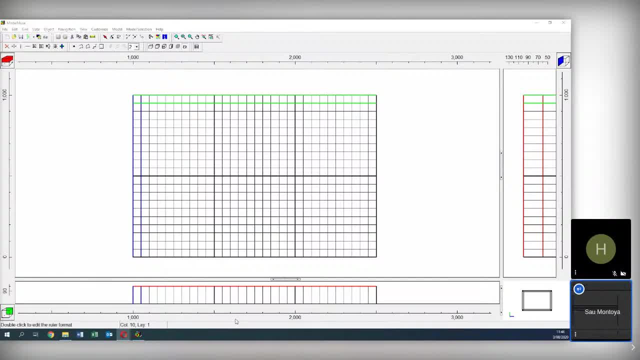 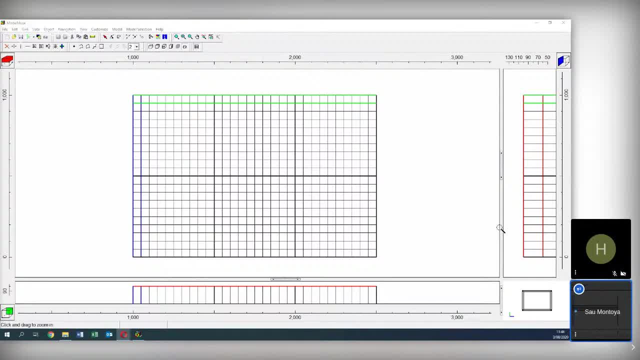 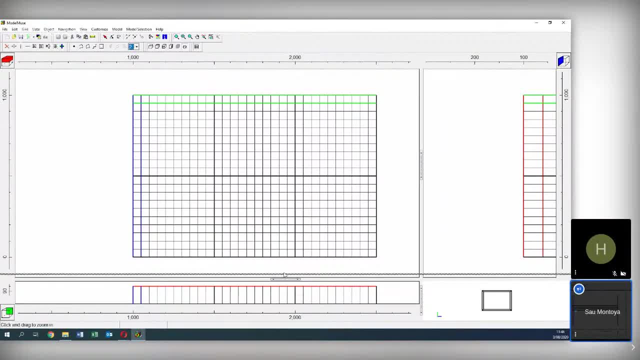 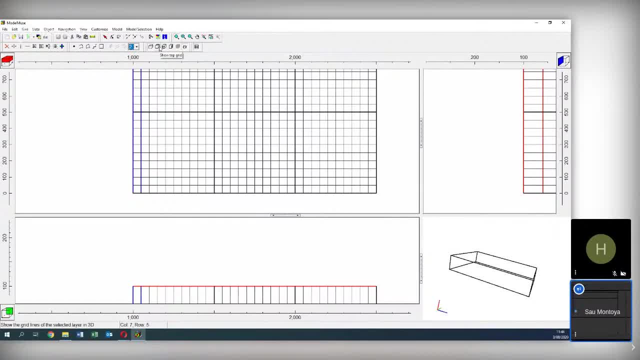 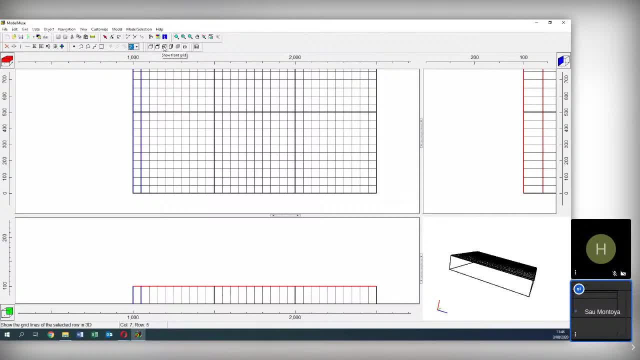 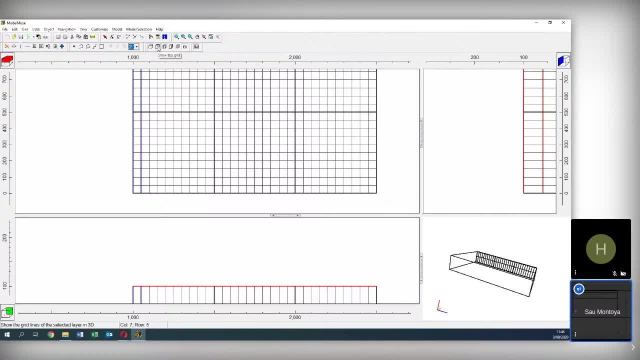 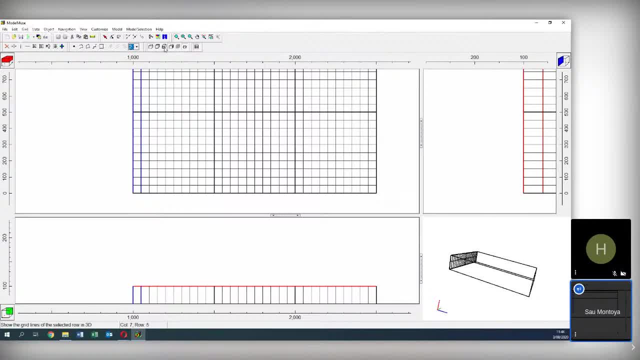 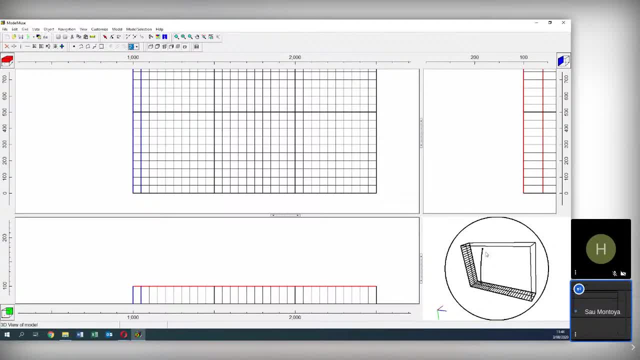 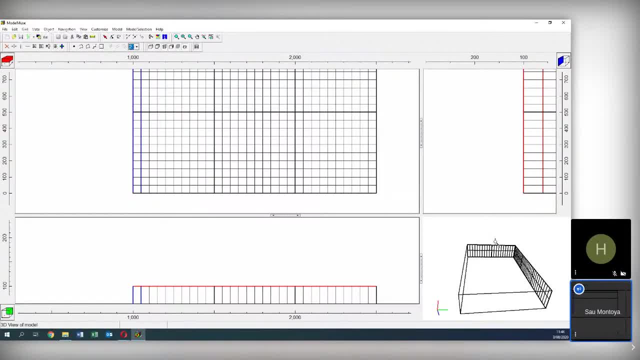 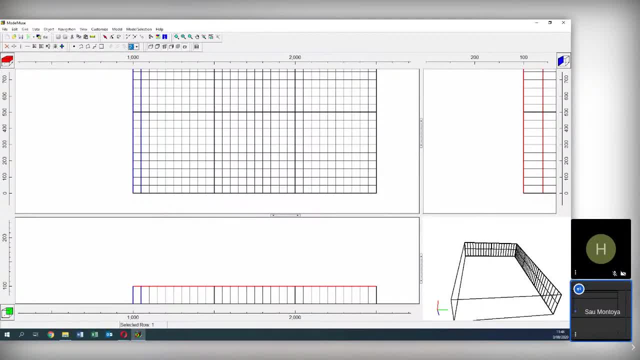 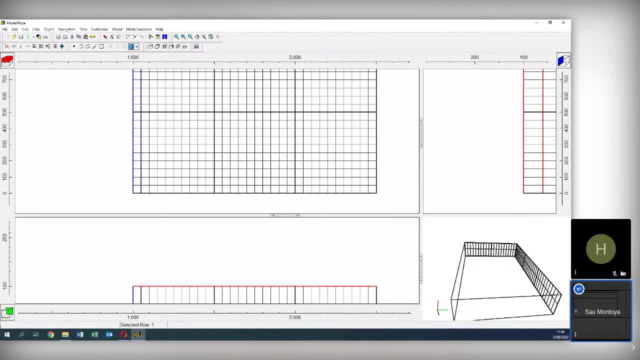 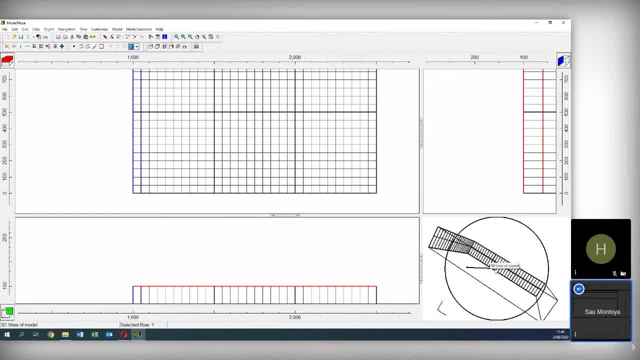 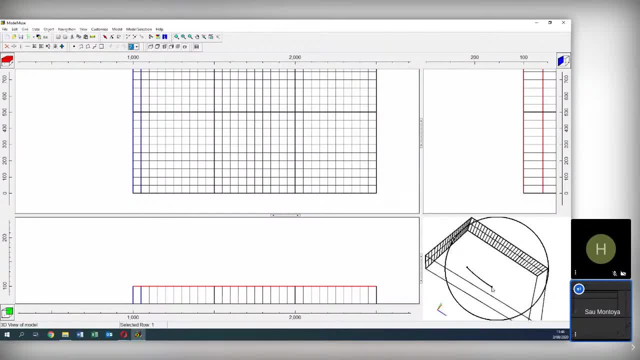 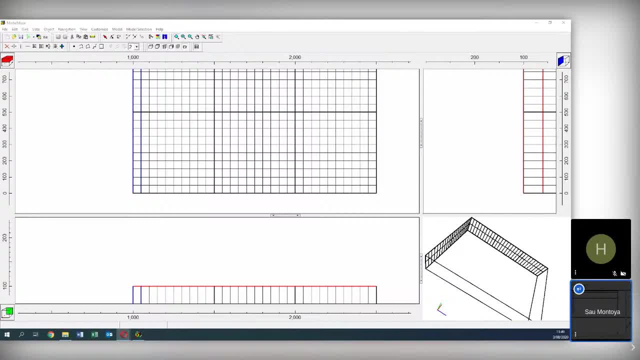 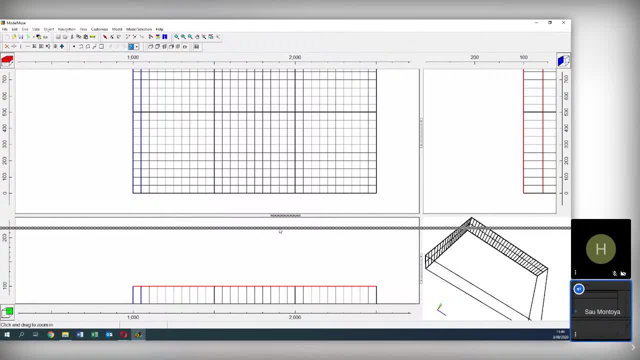 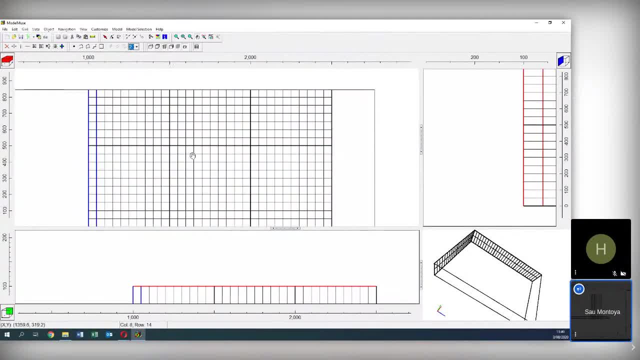 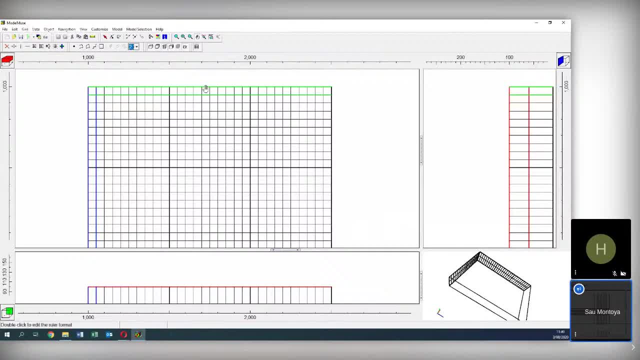 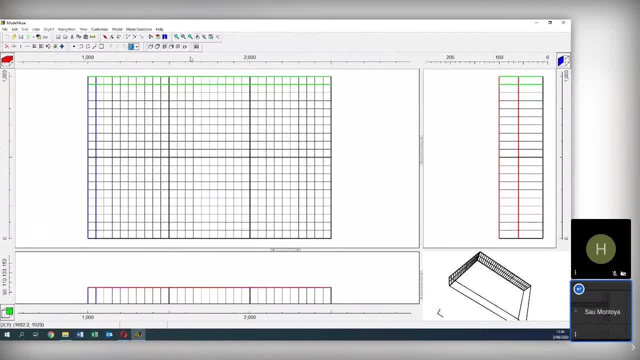 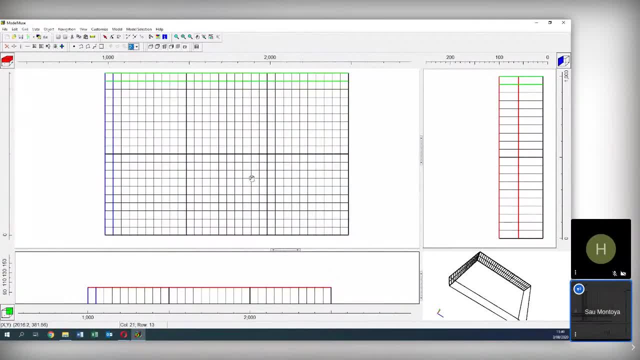 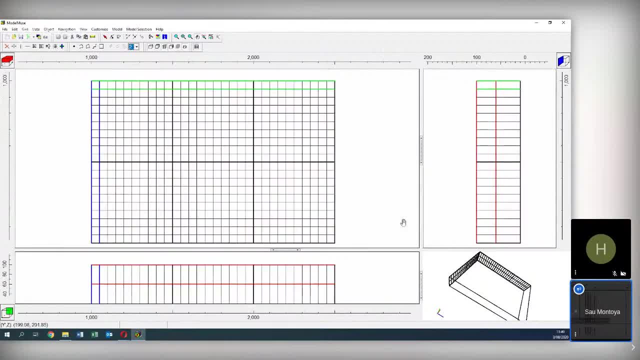 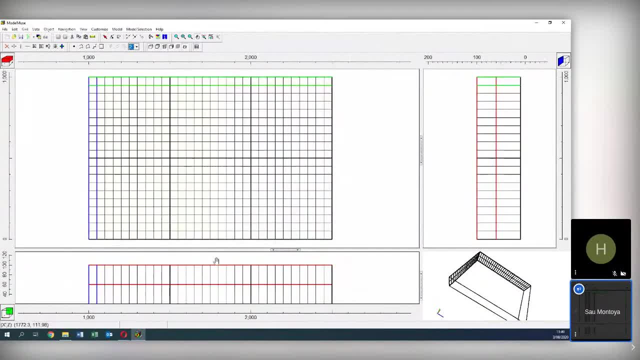 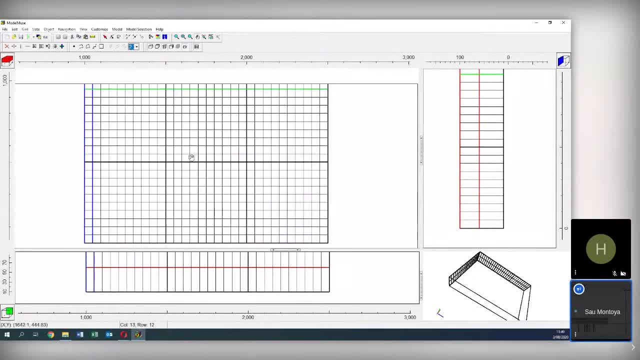 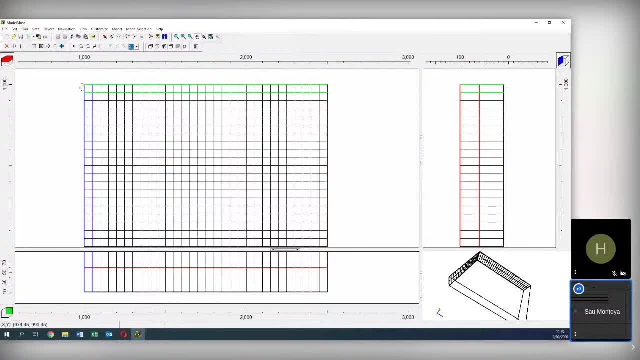 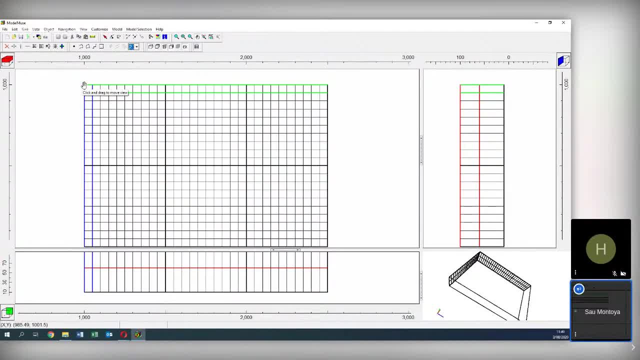 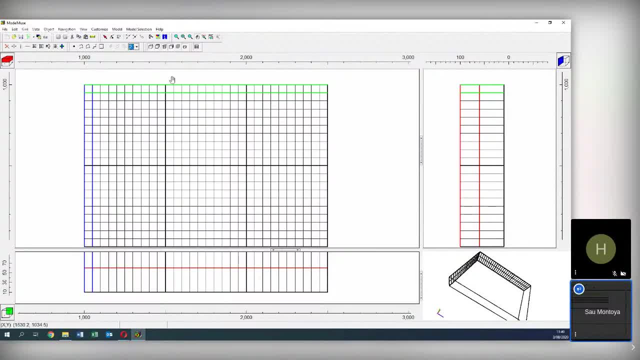 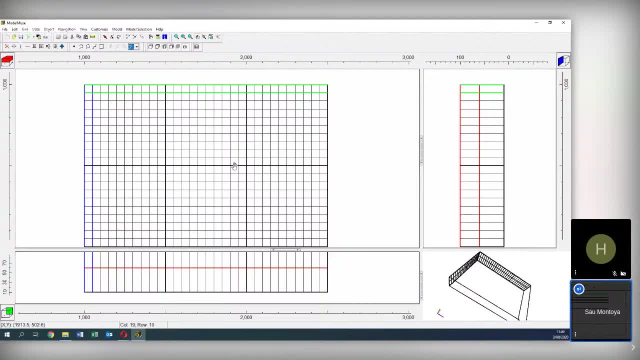 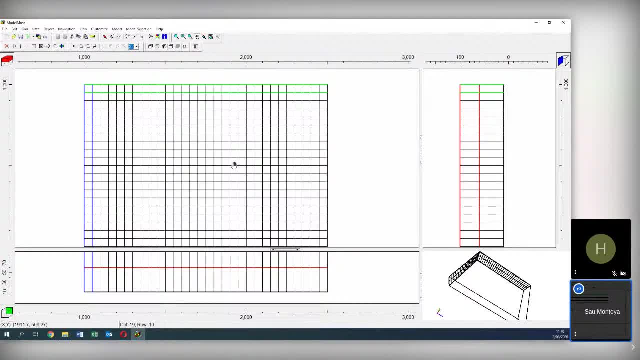 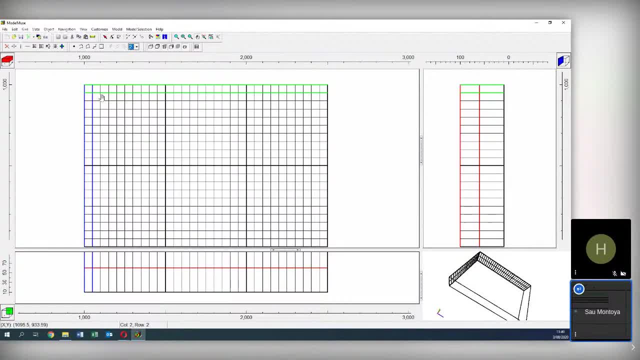 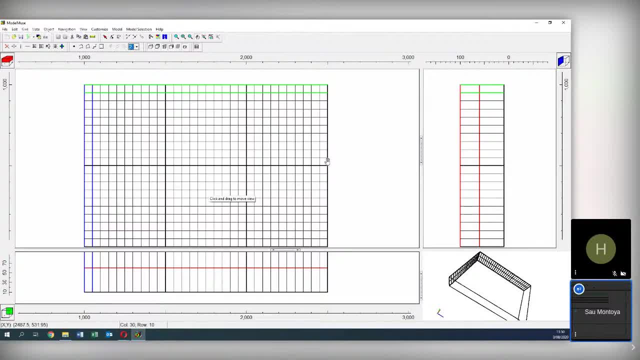 that this line is more than the other ones. okay, and what does it mean? when a line of the grid is more, is thicker than the other ones, that means that is a multiple of 10. so I mean say this is my first column, my second column, my third. 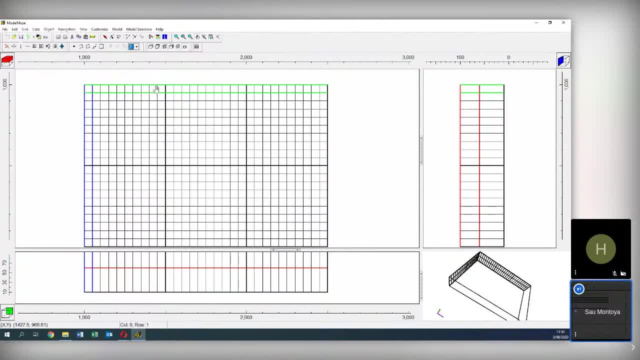 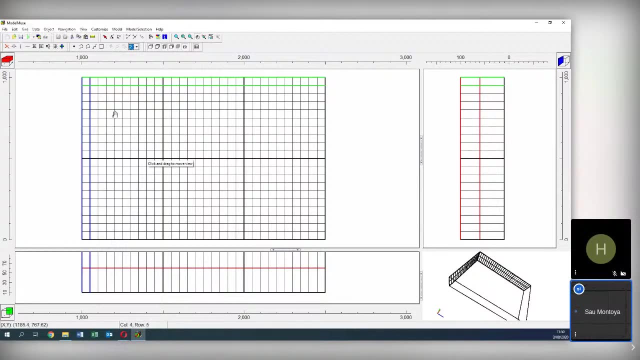 column 4, 6, 7, 8, 9, 10, and then you have to teach, okay, and then you have 10, and then you have the big line. so instead, for example, if I, if somebody asked me which are the number of columns of row that they have, they say, okay, rows 10 and 10. 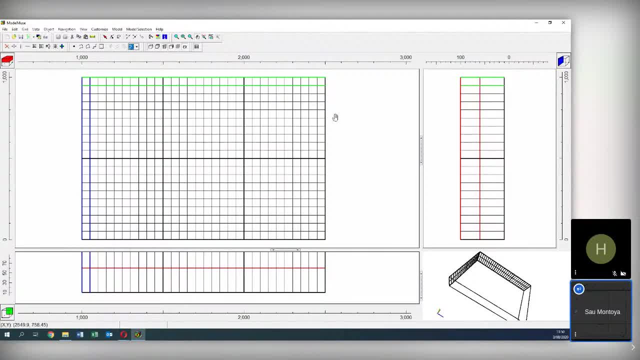 20 rows and columns: 10, 10, 10, 30 columns. okay, you okay, great, okay, let's see, let's go ahead. for example, here we're in the first layer but we go go to the second layer. okay with this, if I press here and can, 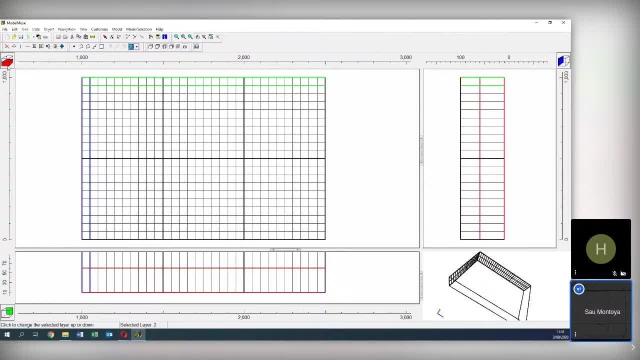 go to the second layer and then go to the second layer and then go to the second layer, and then i get to the translate. since this, the first layer, the second layer has the same geometry and probably parameters. nothing will be seen. okay, and here as well, you can do it with the cross sections. 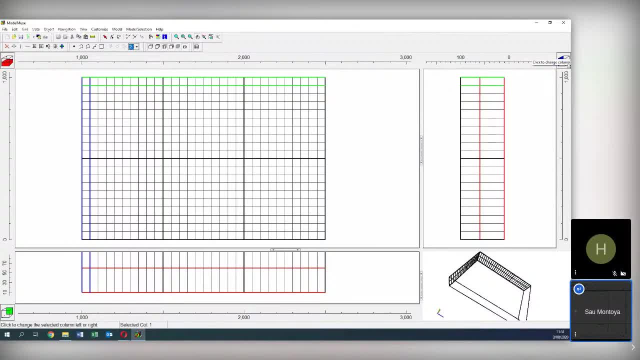 here you will see some changes, because if you press here this, you will see actually the cross section in this alignment, since the geometry in the same is nothing. but i mean you will see the same cross section. but when you are dealing with regional modeling, actually there is a big difference on what you see at every cross section. 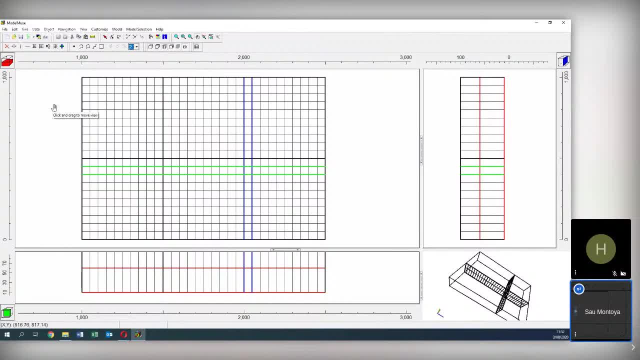 okay, great, what else? then we have the- this is the ruler, and then we have another ruler here, okay, so here we have something that, for example, i can i have say: which is my grid space. my cell size is 50 by 50, so i can check this. so this is around 15, great, and this is around 15.. so i can tell you: 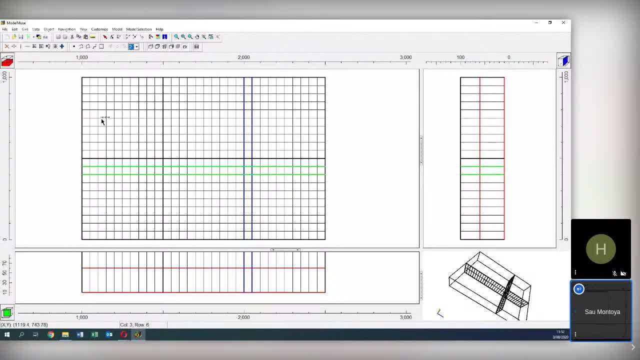 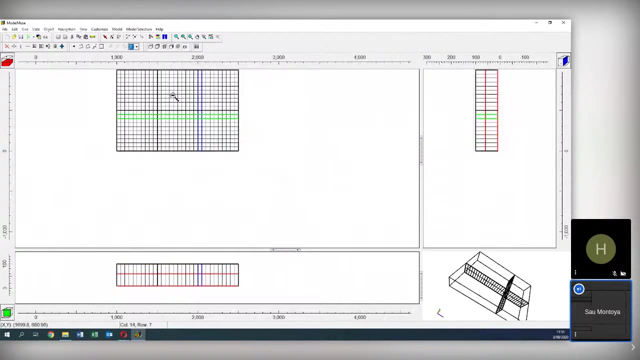 that maybe that my what i have. now i can tell you that the same size is actually 50 by 50. okay, great, uh, and then here you can see the coordinates, what else? and then i can do assume here with this one, and then i can do a zoom out with this one. 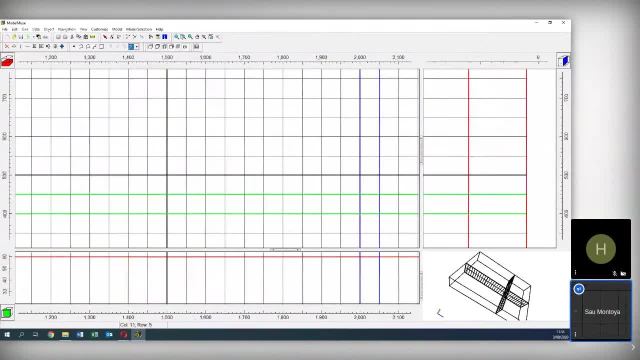 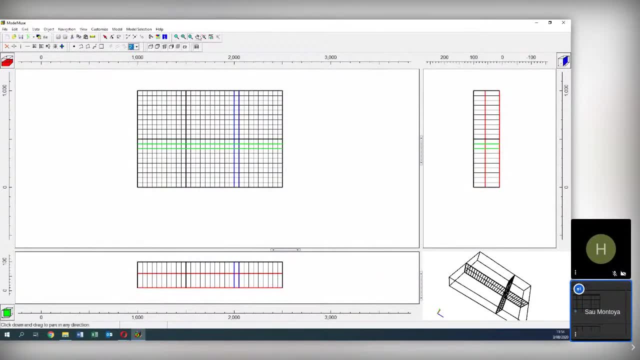 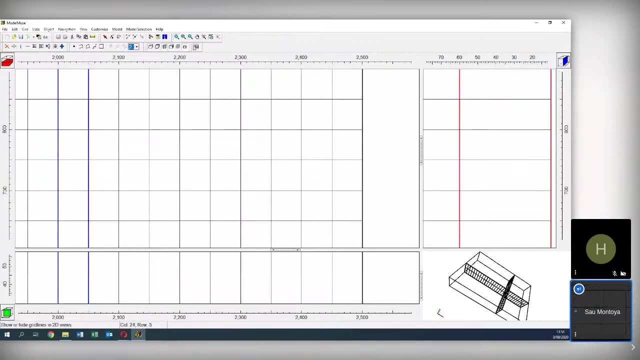 and then this is some window with this. i can do some there, we know, and then i can do something else. okay, so some windows, zooming, zoom out, and this is zoom to preview. so what? what does it mean? so, if i have have done assume here, and I want to go to the latest one, 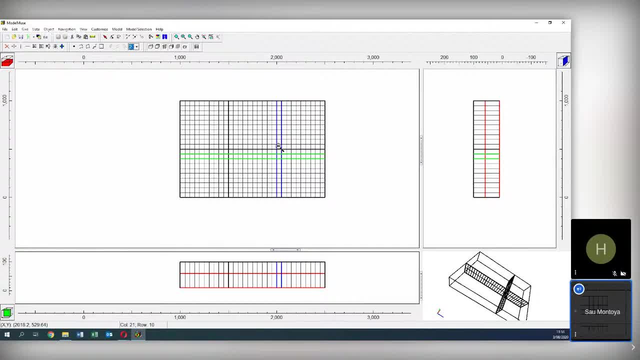 then is a question here. shouldn't the colors in the vertical views be opposite? I should have two cells in each, and I mean why? okay, the green color means this cross-section and the blue color means this position? only the notes, the. the green color means this cross-section and the blue color means this cross-section. only the notes, the- the. 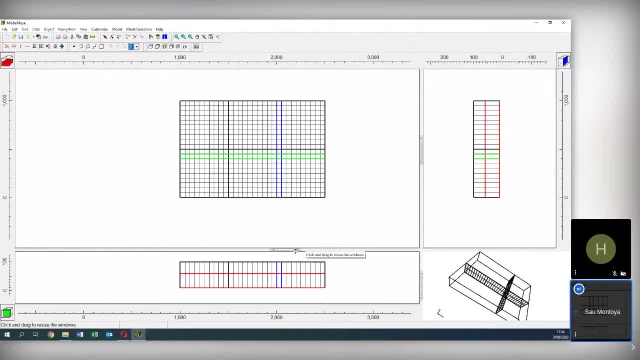 only the notes where the cross-section what? what we are seeing on the post cross-section? okay, great, let's go and let's move. okay, if you are, if you have followed my tutorial, okay, you should have this on your phone. if you have followed the tutorial of the installation you have, you should have. 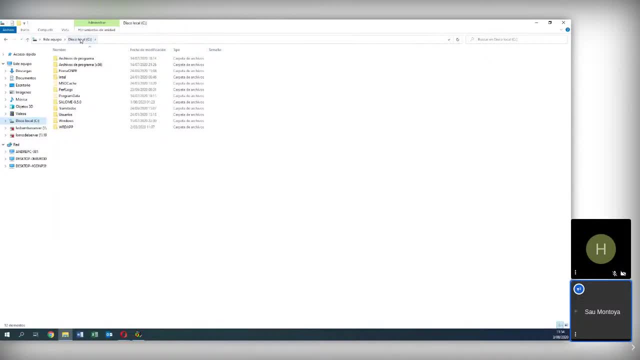 all you have in that we see the red P and then, for example, here I have more photos in five in the beauty and some value. okay, maybe, for example, here I need the mod flow and what I will need is mod flow. six, for example: okay, if you have this folder on your C drive, please type yes. eight, if you. 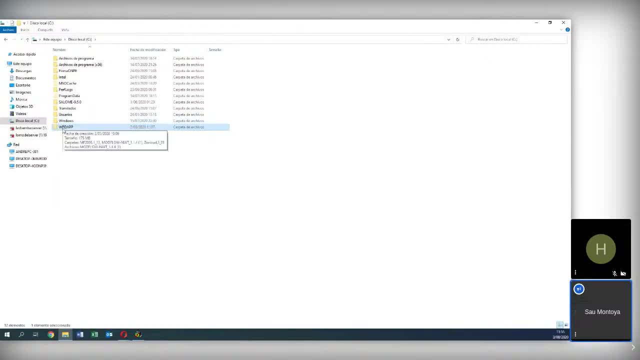 have these very black rice color inside your scenario, please sign yes me. a state is eight. if you have these, order because this folder is. if you have this folder, please type just a. if you have this all of, because this folder is. if you have finished the tutorial in other courses. when I ask: everybody have. 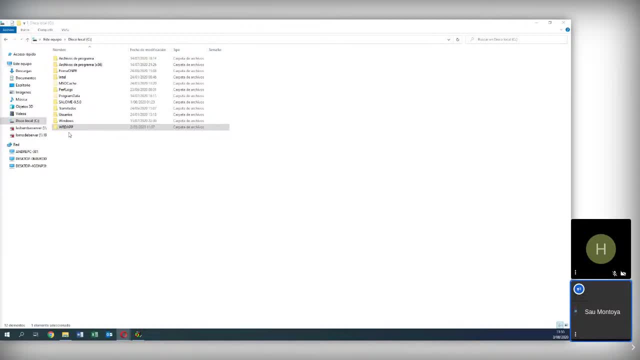 modflow installed and everybody tell me yes, because they have model views installed. but this folder is actually the engines that will run model views. ok, if you don't have it, don't worry, there is the tutorial. that on the tutorial. go till the end of the tutorial, because in the end of the tutorial is where we are going to install this, for. 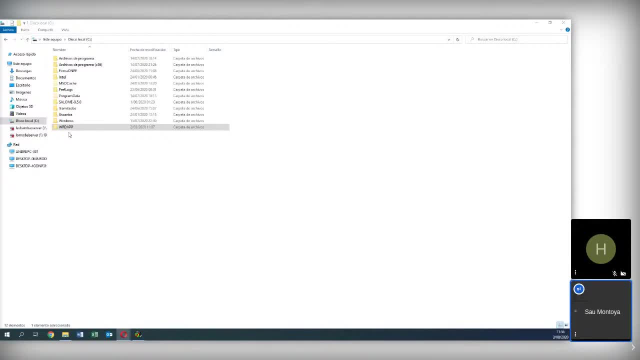 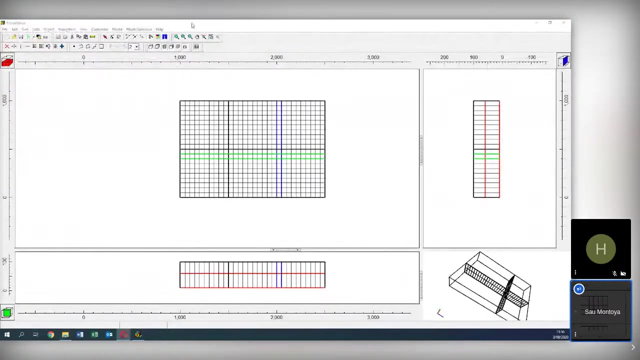 example, I will do. I know that I don't have the WDL app completed because I don't here- in my case, I don't have the modflow 6, so I will do it and for the people that has already done is a refresh and for the other people will be the. 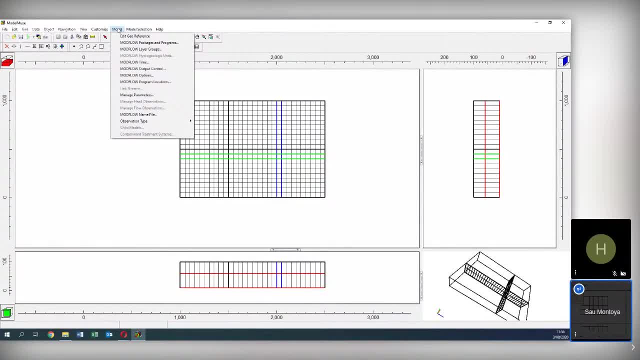 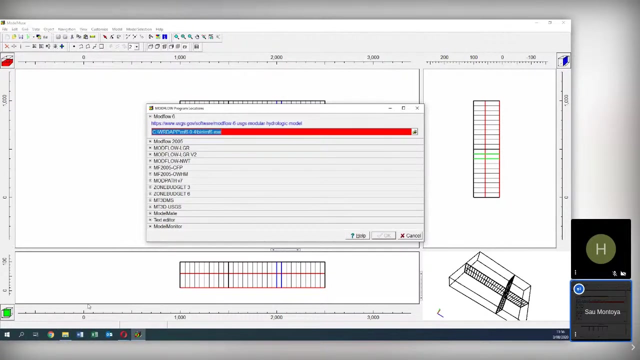 extent that you will do after this class. so in model, everybody goes to model and then goes to program locations. okay, so in model, everybody goes to model, modflow and modflow program locations. Wow, yeah, my advice is to to do the complete tutorial, please. ok, so the complete tutorial will be. 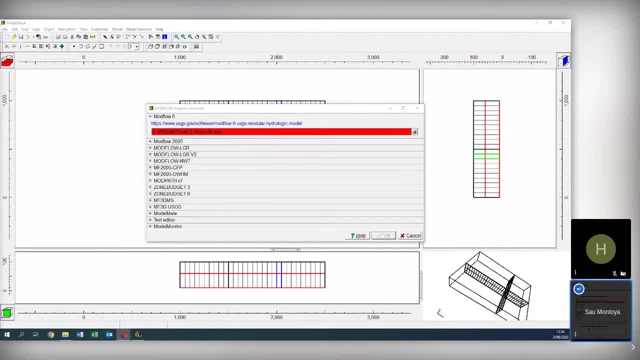 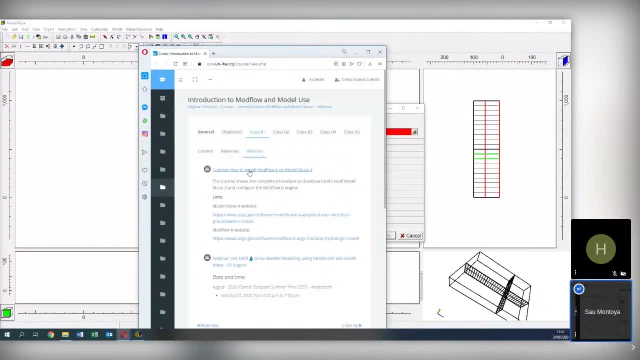 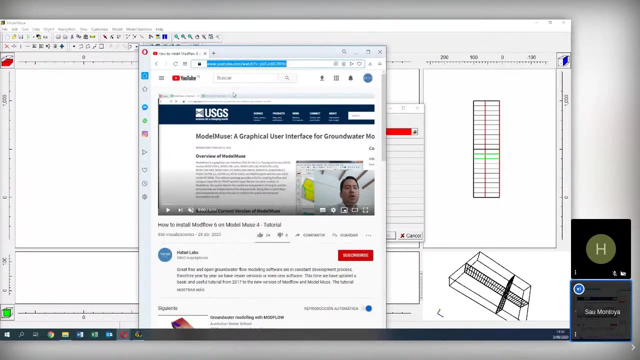 here on the course to install tutorial, to install model of news. and then here my face and I will drop this, the chat, and then you will see the WKD app. you will have to create it by your own and then you have to place the files. okay, so the end of the tutorial slorm up…………………………………………. 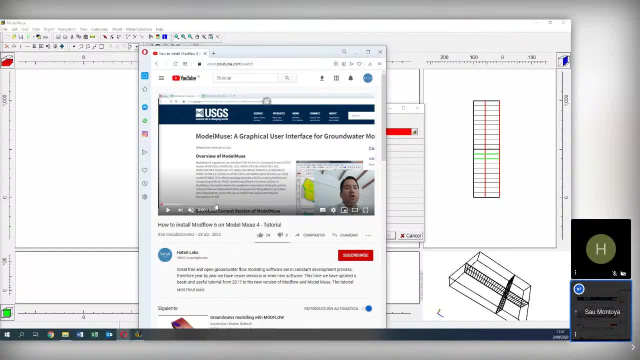 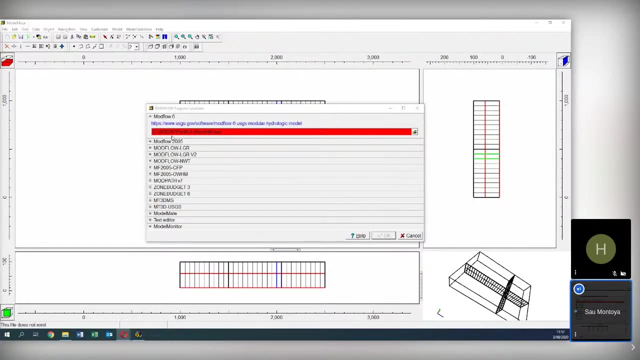 so see Fah's video tutorial to install modflow on model musl successful. okay, so here, for example, I don't have my process, I do not have this, but I have here a link, so I, what I do, is I when I have a double click here, or 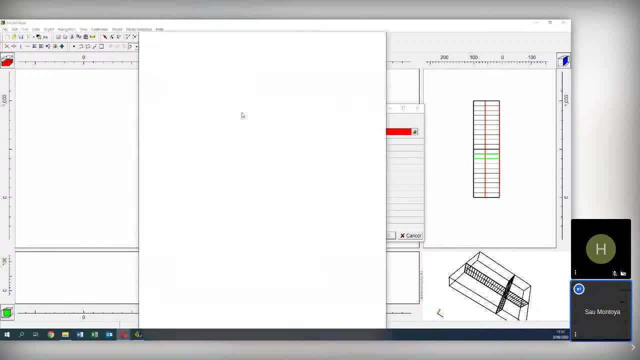 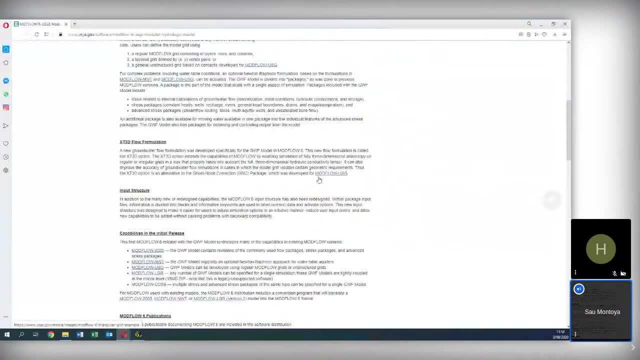 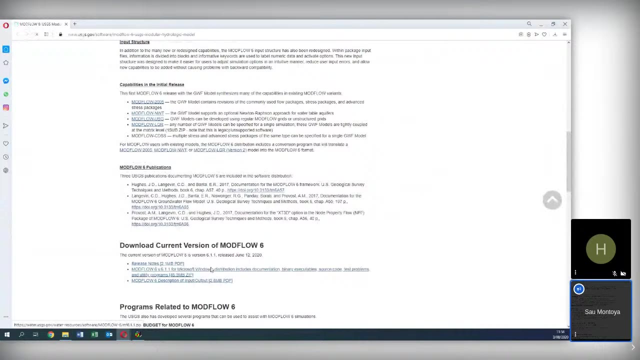 click here and it will redirect me to them, to the MoFlo 6 website, and I say, okay, I want to download MoFlo 6 for Microsoft Windows. yes, open this and it will start downloading MoFlo 6. that is 6.11, that is released on the latest June. 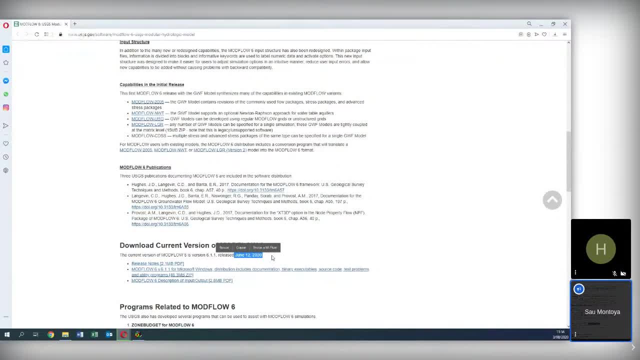 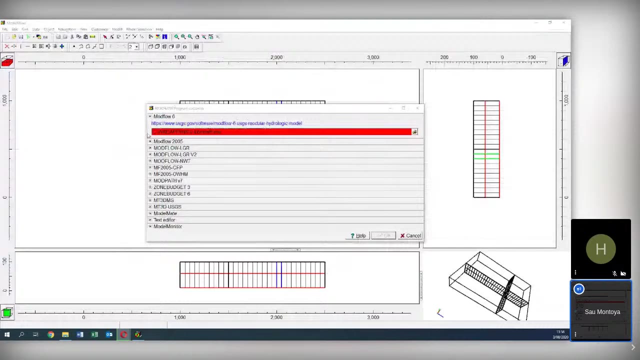 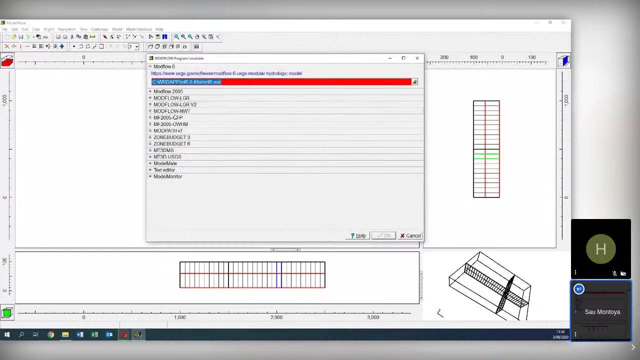 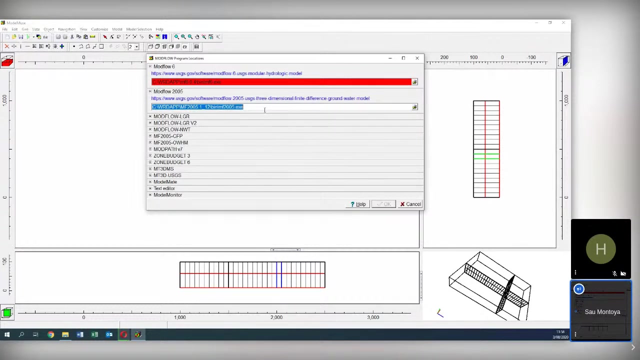 okay, actually it is downloading and it is kind of okay with it. some time I can explain some things here. okay, here it appears, some of the MoFlo options, together with some other options for pre and post processing. okay, so here we have the engine for modflow 6. we have here the engine, for example, here i do have installed modflow 2005. 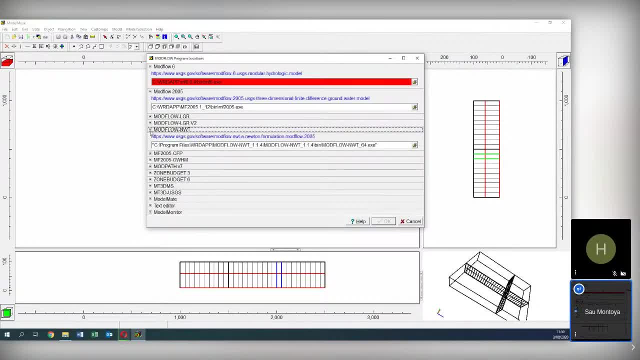 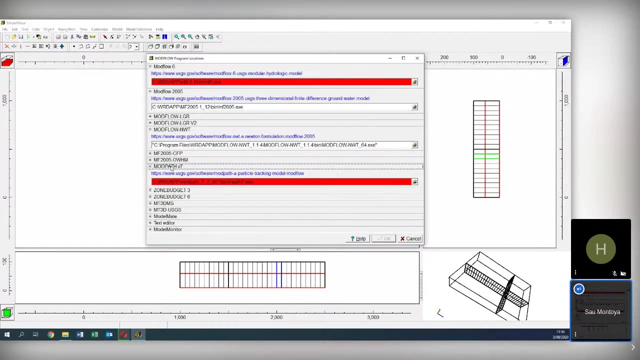 i do not have modflow lgr. i do have modflow nwt. i don't have modflow cfp. i don't have modflow, only the uhm and, for example, not. but what is mode? but not, but it's a particle tracking model. okay, so, and this is coupled to modflow. what does it mean? that if i have a groundwater model and 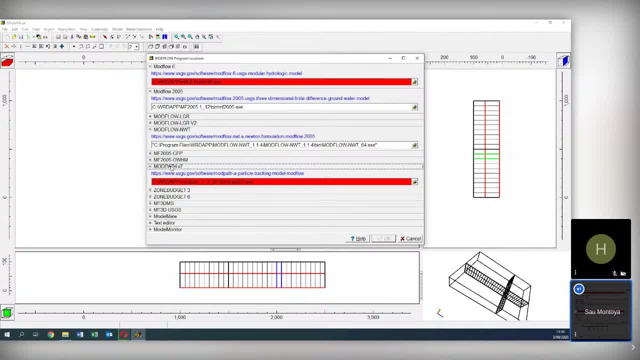 then i want to see which is the trajectory of any particle. this particle has to uh. modpad can simulate the predictoring, the path length of this part. Then you have some bucket and what is some bucket. If you want to do a water analysis of a certain part, 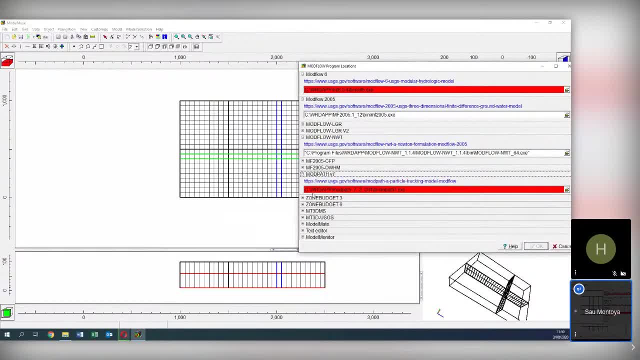 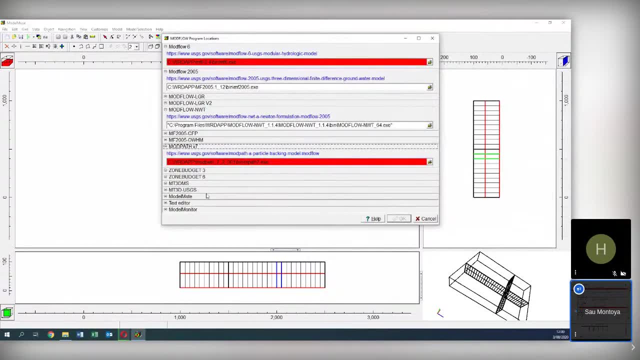 of a certain boundary condition, or so you can do it with defining as some bucket. Then you have this MT3D-MS and MT3D-USGS. What is this? This is a transform model that is also coupled to Moxflow. 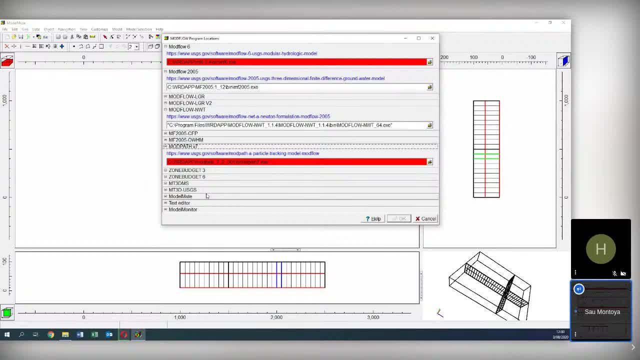 And MT3D-MS was done by the University of Alabama, like year 2000,, I guess- or maybe I can be wrong- And there is a latest version of the MT3D-USGS that is a code developed by the USGS. 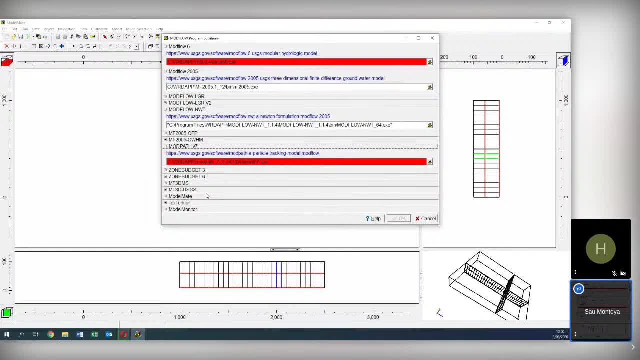 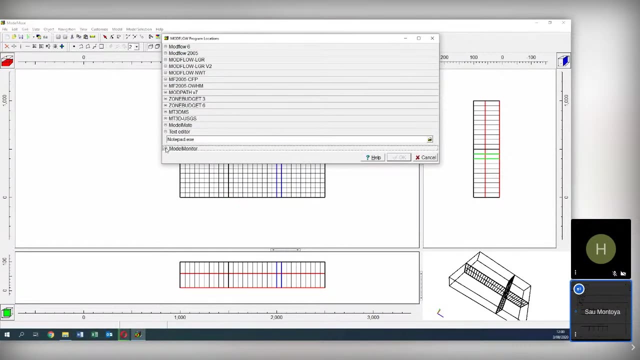 that was released five years ago, I guess. okay, If you want to do some sensibility analysis or automatic parametrization, you can use ModelMe, And then the text editor by default is defined as the notepad and the model monitor is this one. 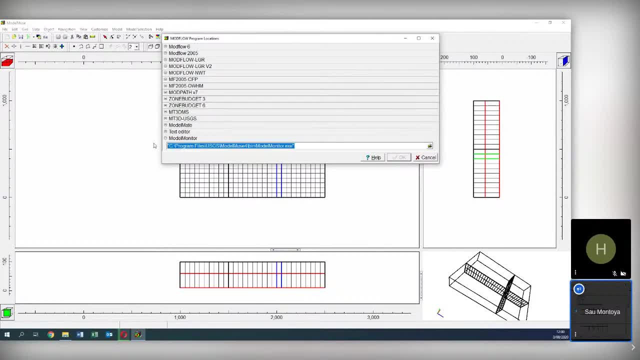 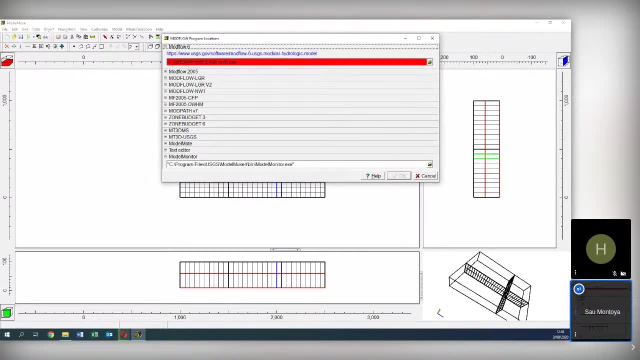 And this is a utility that will help us when you run a model. Okay, So please tell me which. you have Moxflow 6 installed on your computer. If you have Moxflow 6 installed on your computer, please type yes, nine. 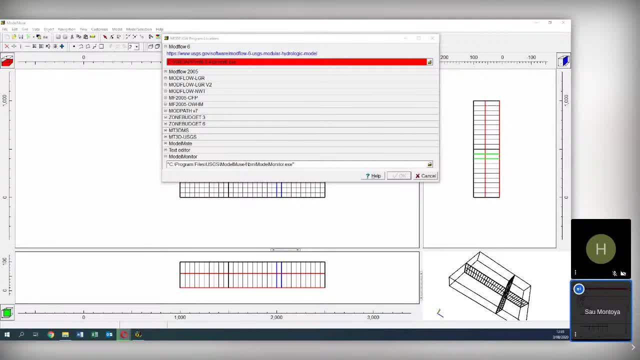 And this will help you do the all the recognize and see the data. Yeah, that's all right. Yeah, So now I can get done. Okay, Hans, are you there? Yes, I'm there, Hans. it will be, let's say, methodological or pedagogic. 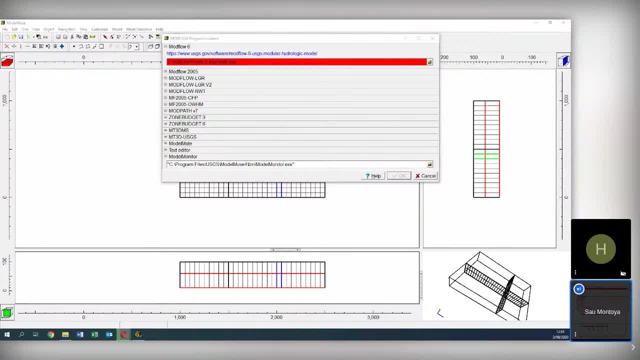 everything in the row. I mean, it's really up to you. How long do you still have to cover The half, Because it was designed for one hour? Okay, I think you can better continue, given that people have reserved the time now and their bandwidths. Okay, so let's continue. 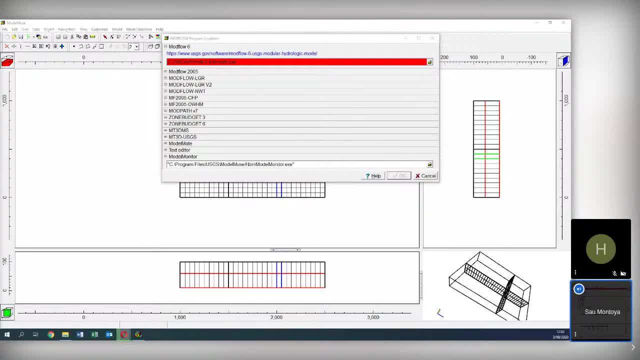 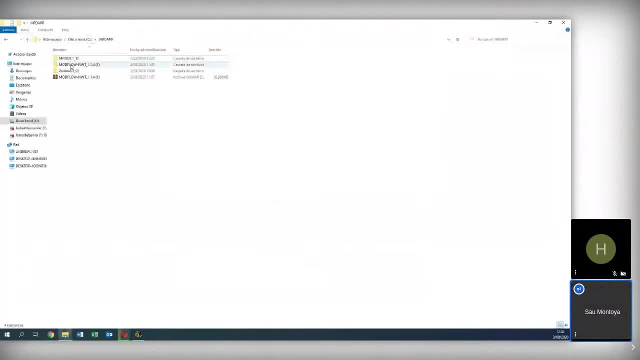 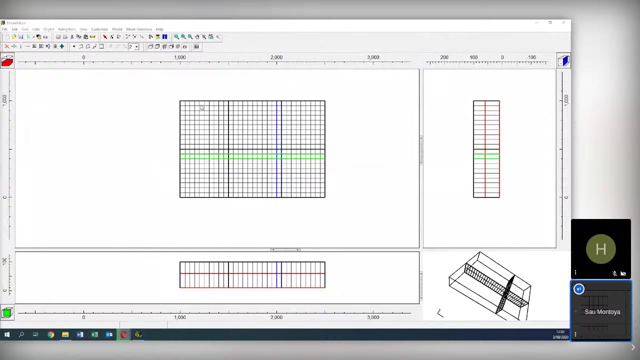 Okay, so it goes. Yeah, I will continue with the next step. Okay so let's continue. Okay, I can install Modflow 6 later. Okay, so the objectives of this second part is the learning, the function of the basic tools. 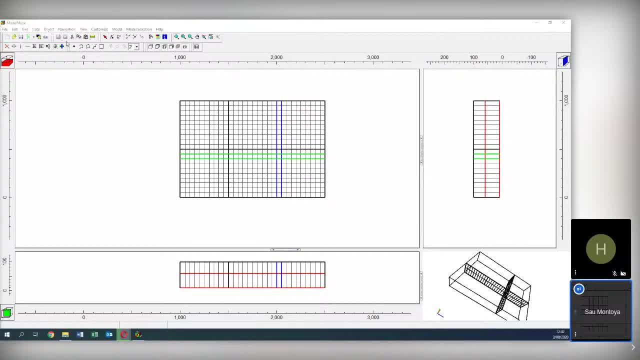 So here we have the five of the five geometries available in Modflow in modern use. Okay, so this is the point, the line, the polygon. Okay, this is the point, the line and the polygon. Point line and polygon. 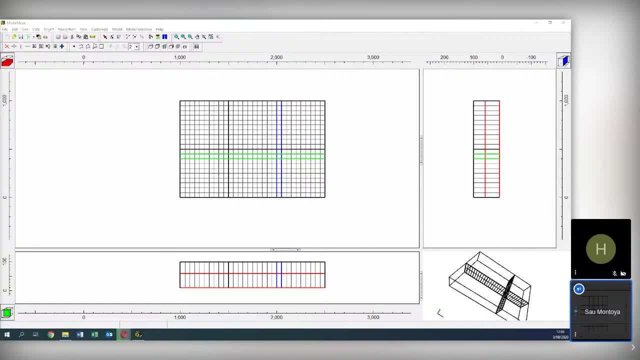 However, you have these two options that are really close. This is a straight line and a straight polygon. Okay, so what does it mean? That if you do a polygon or a line, for example, I will do, Okay, I will do. Then you will say: I will do a line Because this is more to show you. 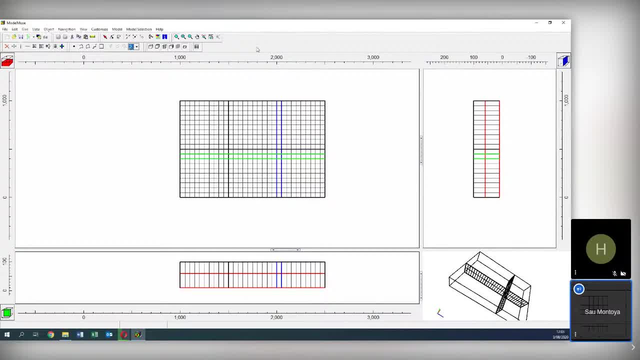 Let's go Okay. Okay, I will do a line. This is a normal line that you can find anywhere else. Okay, But however, if I select this, I can do a line, but only parallel to them. For example: 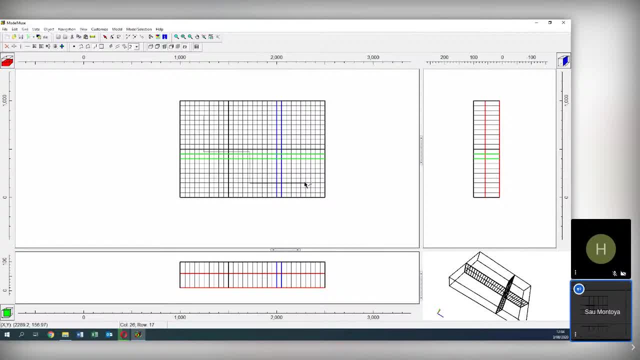 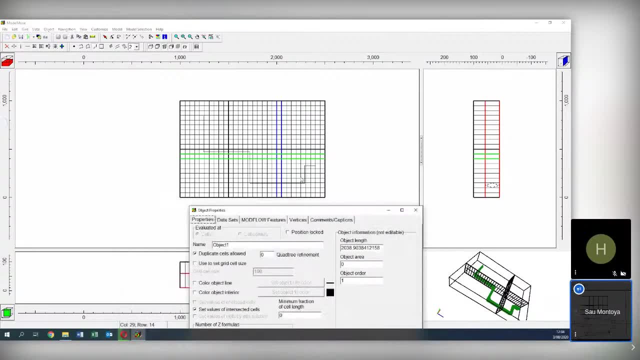 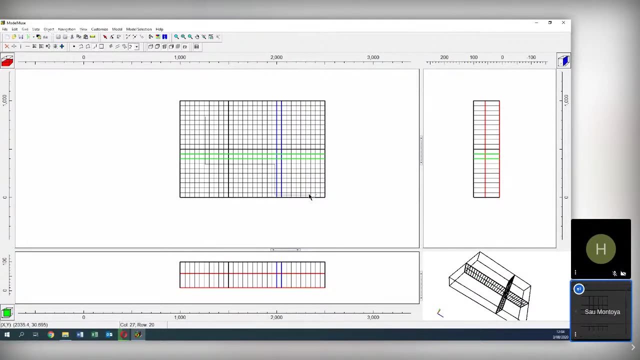 Okay, Okay, Okay, Okay, I can do only parallel to the axis. Okay, To x-axis and y-axis. Okay, So this is the. this is a line, but this is a line that can be only parallel to the x-axis and to y-axis. 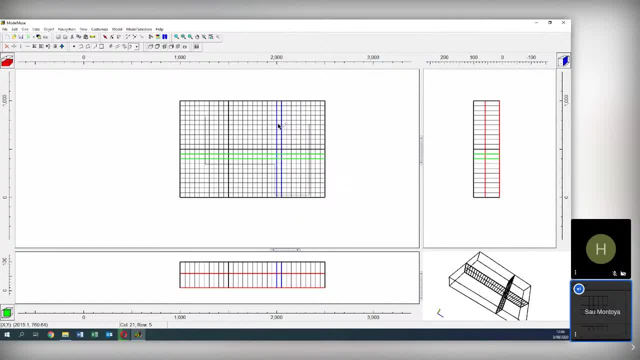 Okay, So this is the line. Okay, Great, And the. and this is a straight polygon. It's also a polygon, but it can be only parallel and it has to be a square. Yeah, Okay. So this is the difference between these two. 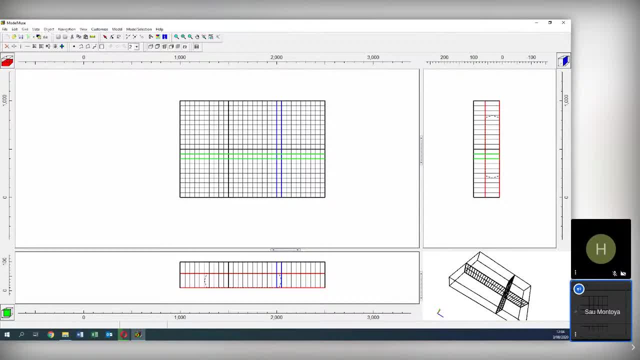 So actually those are special conditions of the point line and polygon. Okay, Great, So we have, we can, we are going to make. I mean, if you are going to select a river, you can do it with lines. 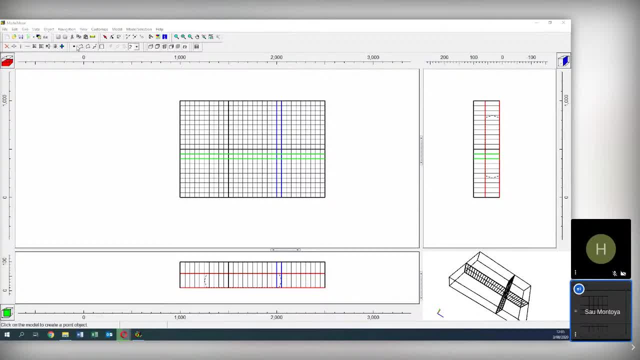 You can do it with lines or polygon. For example, if you are going to create a, well, you have to do it with points. If you want to create a polyline, you can do it with. if you want to create, represent a river, it will be a polyline. 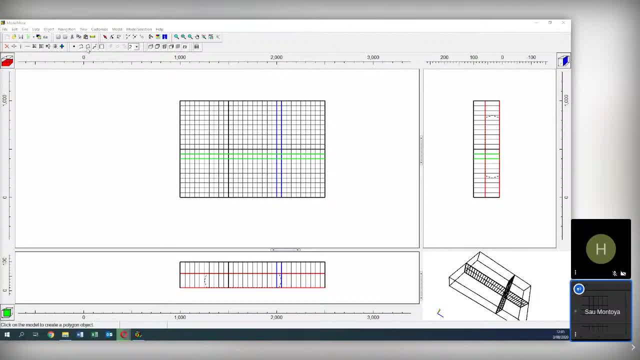 And if you want to select a wetland, you can do it with polygon. Okay, So this will be mostly related to points. This will be mostly related to streams, And the other ones will be related to wetlands or to protection zones, or will be related to contaminant sources as well. 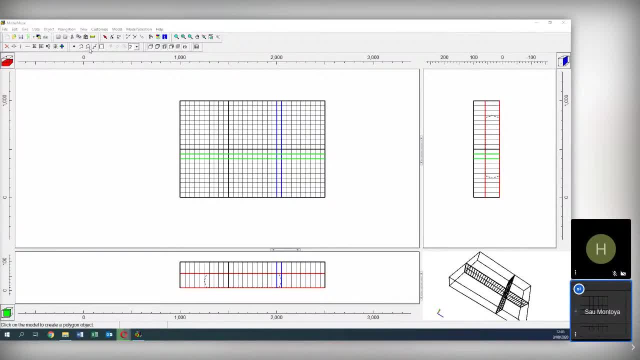 Okay, This I mean we are. you as a modeler, you have many tools And then you can use the tools, But you can also select the only tools, for the tool. I mean there is no. I mean the software allows you to do that. 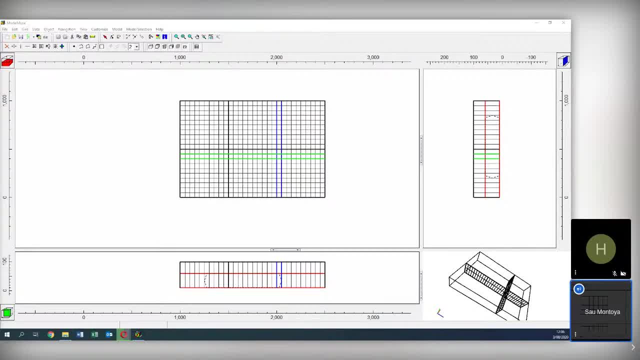 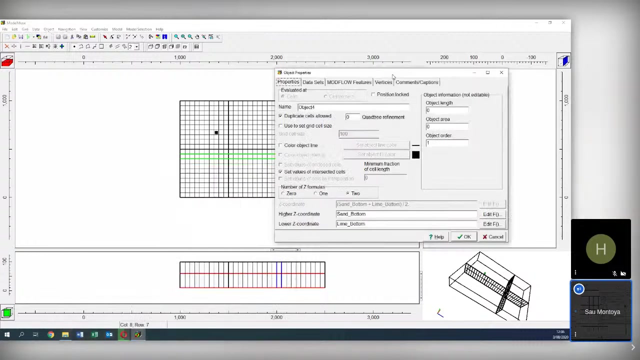 Okay, So let's. so let's create a new line, a new point. So let's create a new point, Select this one And press anywhere in your model: Okay, And then this window will appear. So, if you have, if you are here with me, type yes, 10.. 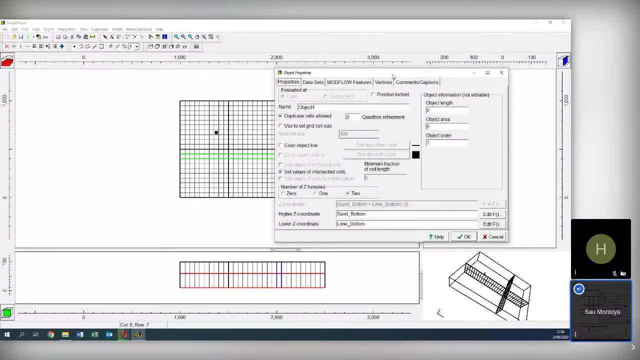 If you are here with me, type yes, 10.. If you are here with me, type yes, 10.. Okay, Let's have a look on the different. let's have a look on the different conditions here, Because it can be that for you, you have some different names here, but there is no problem. 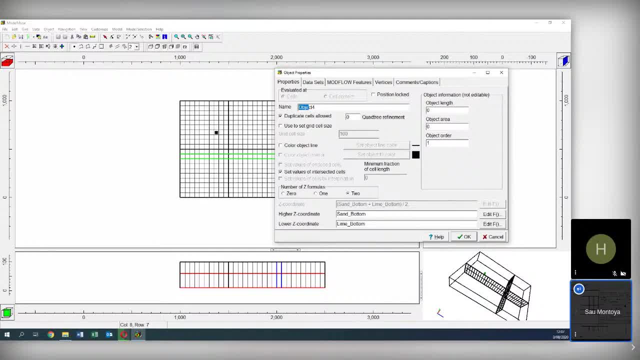 But please have a look, and then we are going to, and then we are going to review all together. Okay, So here, this is the name. The name is actually aleatory, So we can type well, for example: Well, Okay, 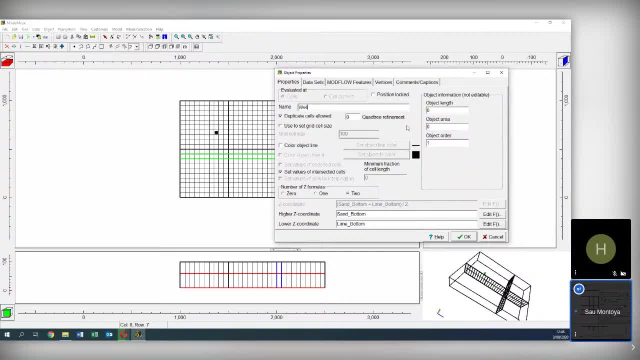 Great, Then what else? Then we have the object order. For example, for me it's the first object order. If you have done any object before and then you have deleted, actually you have a. you can have. this object order actually is the index of all the objects that are on the model. 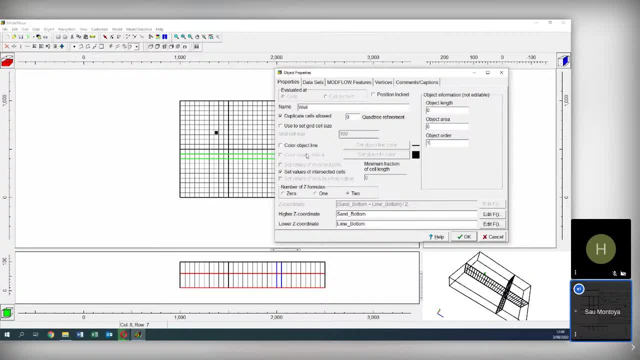 So in this case we only have one, So it will be one. If you change the color line, why not? Why not change it? Because by default it's black And if you leave it in black, actually it can be confused with the grid. 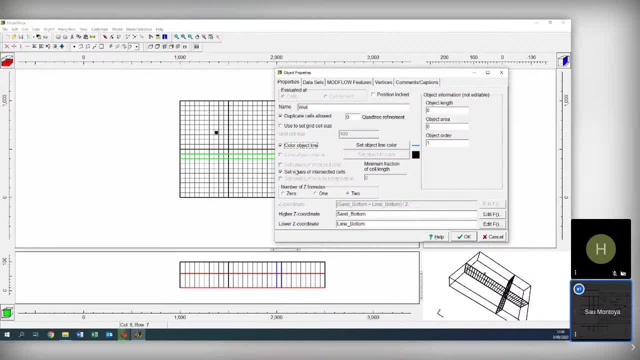 That's why I always change: Okay, So let's see. And then, for example, you can define as quatri-refining. Okay, And this is something that I will explain right now. Okay, If you are here with me, yeah, type, yes, 11.. 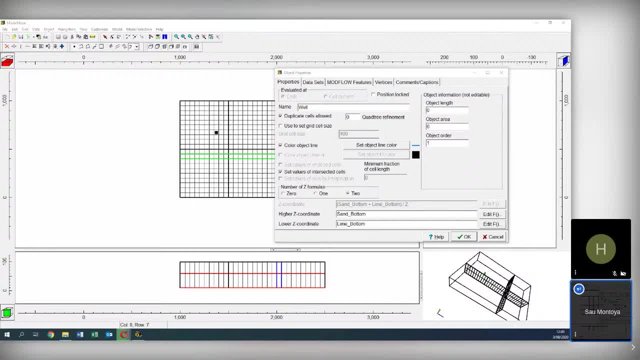 If you are here with me, type yes, 11.. Okay, We are. yeah. Yeah, I have seen that the course content was designed for one hour. We are going to do 15 and then we have already over this one hour. 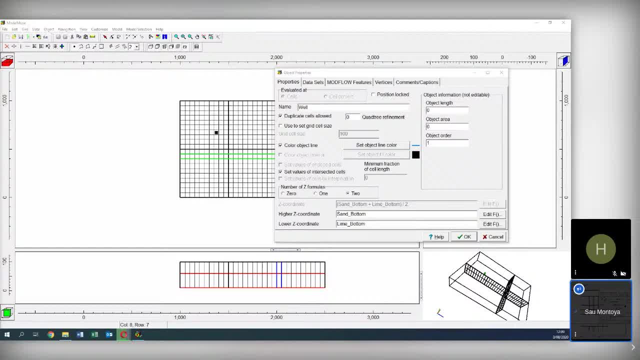 But we are going to do 15 minutes more, Hans, is that correct? Give me your approval. Fine for me, Sol. Yeah, And because I don't want that anybody that has to leave this course can be missing something for the other. 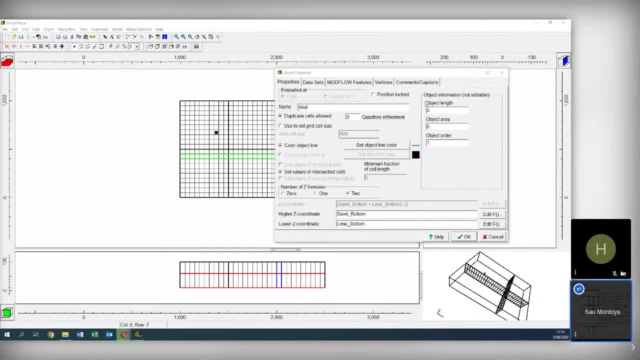 Okay, And, as I told, as in the organization, this link will be available for you to review afterwards. Okay, So let's talk about the number of set coordinates. Okay, So here we have 0,, 1, and 2.. 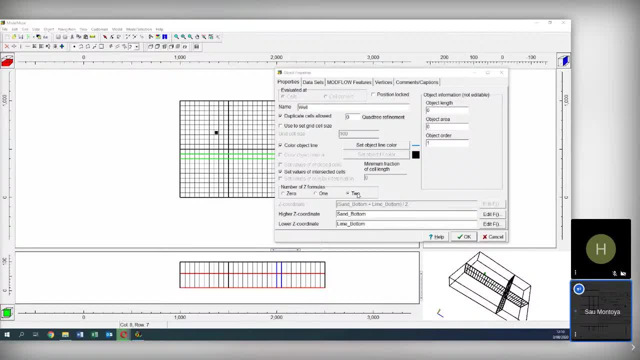 And what does it mean? Okay, Which are the objects that are not related to the elevation? For example, the evapotranspiration that we charge is not related to the elevation, It's related to the model itself. Okay, So if you want to define a special object that is not related to any elevation, 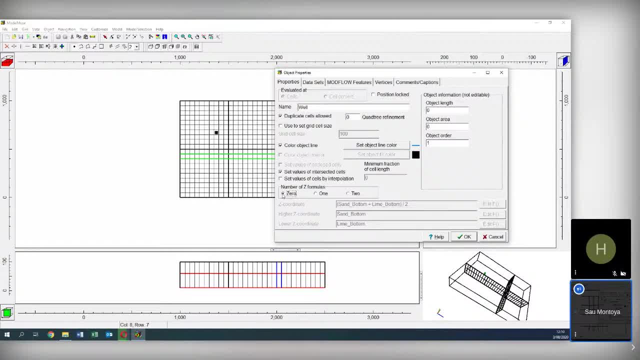 you type, you press this 0. Yeah, But if you want to define, for example, a well screen or, for example, a river location, you have to relate it to one elevation, because the river is located at just one elevation. 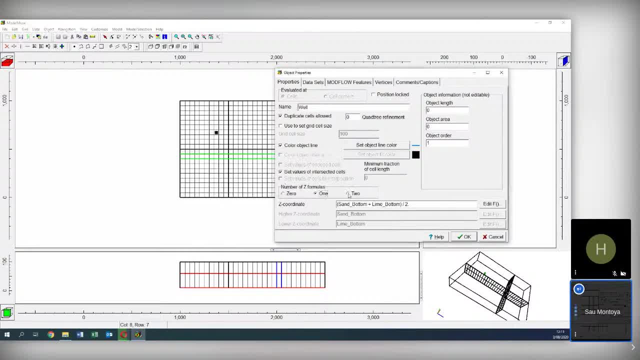 Okay, But for example, if you want to define this as a, for example, if you have a drilling log and in the drilling log you have certain material from one elevation to the other elevation, you can define this as two formulas, Okay. 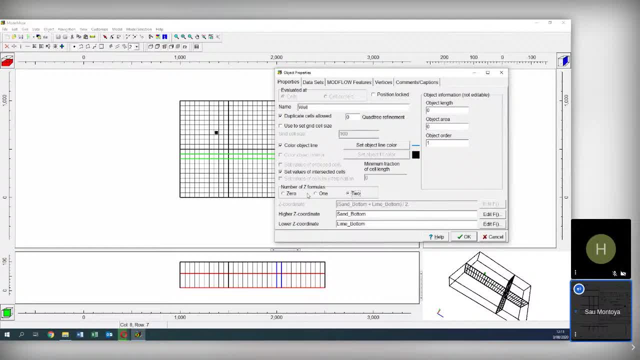 So this is how it works. These formulas define um, the, the set direction of your object. Okay, In this case, we are going to define that, since this will be a well, our well will be located 10 meters below surface. 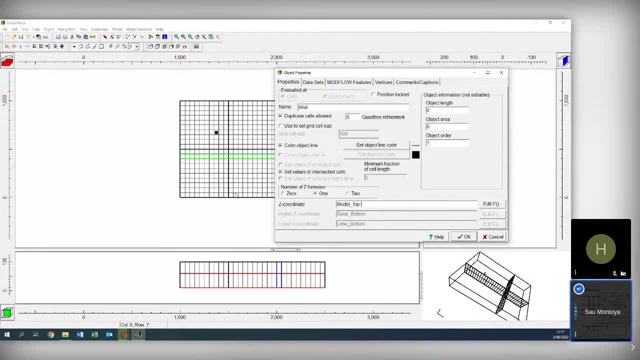 Okay, So it will be model top minus 10.. Okay, Let's see I can type model top minus 10, because my model top is 100 minus 10 will be 90. Or I can type as well, 90. It's the same. 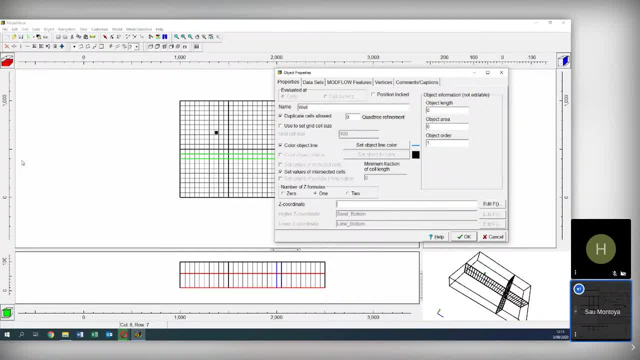 Yup So, but I will say model top minus 10.. If you are going to work with model top, just remember there has to be model with capital M underscore and capital T. Okay, Great. So with that we have our. 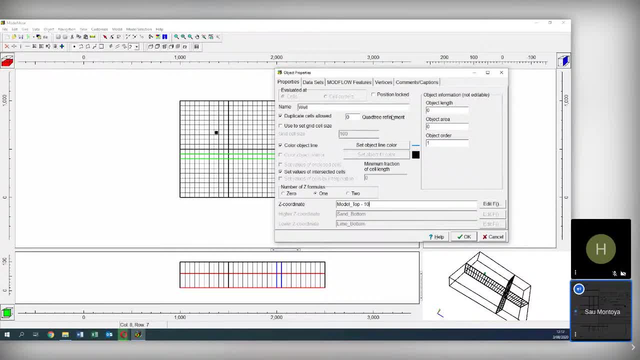 and this is the quadrant refinement. The quadrant refinement is actually, uh, not being used here, because I will tell you where the quadrant refinement is being used. Okay, So far we are only going to define the object. Okay, And then, if I go here to data, 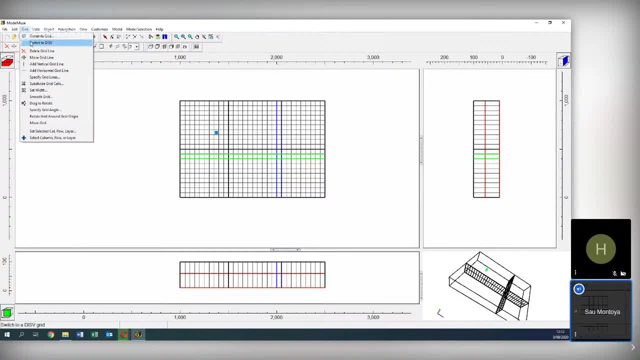 not to grid. if I switch to discretize by vertex, okay, if I switch to discretize by vertex here there in discretize by vertex, that we are not going to do, but there are tutorials on that- we can shift to. 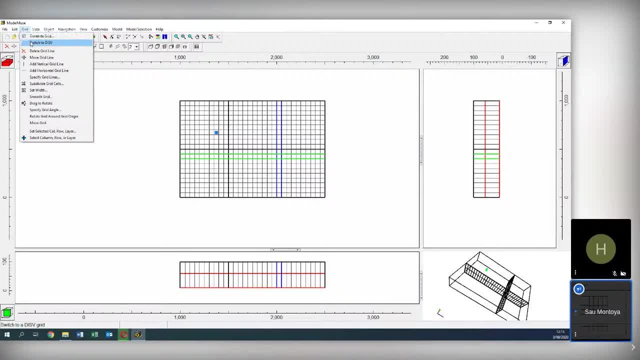 we can do quadrant refinements, Okay, That is a type of local discretization in module. Okay, But we are not going to do that, Okay, So okay. So here we have our web, and then we are going to create a ribbon. 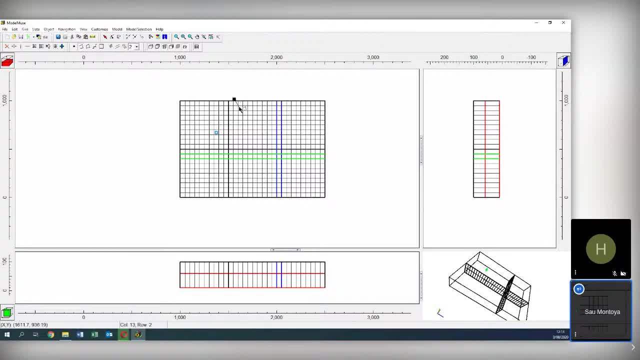 We create a river that crosses. We create a river that crosses. Yeah, The river crosses the model and actually, as you can see here, it's crossing the model. Okay, And then I do double click. I do double click here. 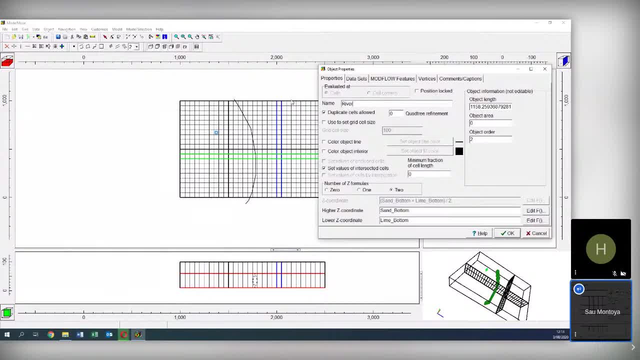 and this will be my river And change color. Okay, And then I just type one formula. and then I just type one formula because for me, my river is model top minus two. my river is model top minus two. my river is model top minus two. 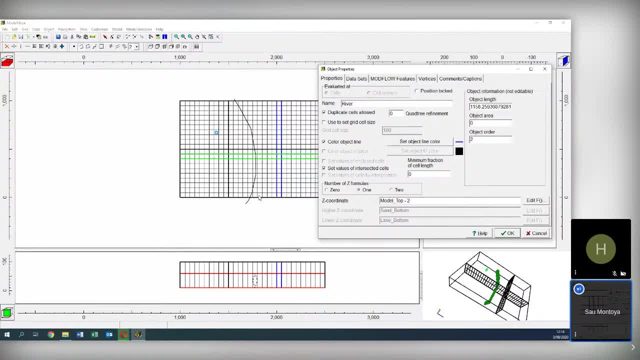 Okay, Model top minus two. Okay, Okay, Yeah, Yeah, Yeah, So this will be river and this will be model top minus two, and this will be river and this will be model top minus two. There is a 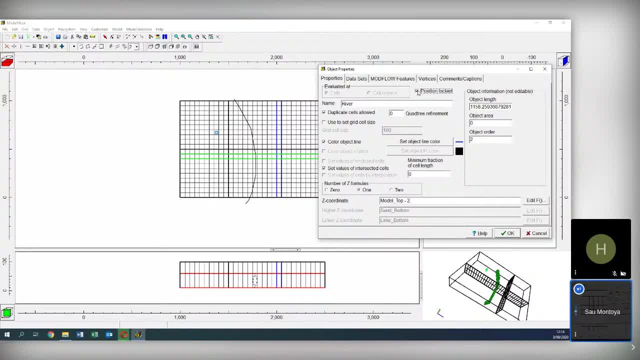 there is a, there is an option here that is position locked, And what is this option? Okay, Imagine that you have imported your river network. Okay, We are going to do- we are going to see that later- where you can import a river network. 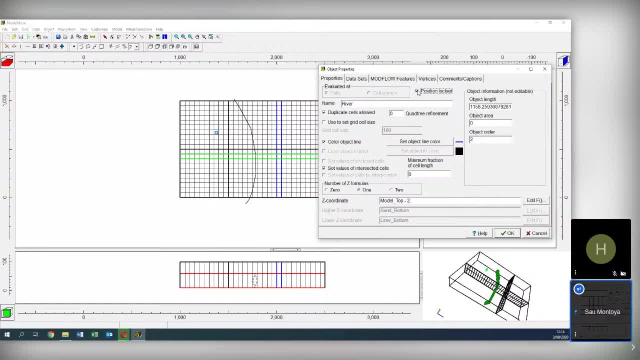 But imagine that you have imported a river network. Okay, You don't need. for example, if I don't press position lock, I can change the, I can change the location of the river. I can change the location of the river. 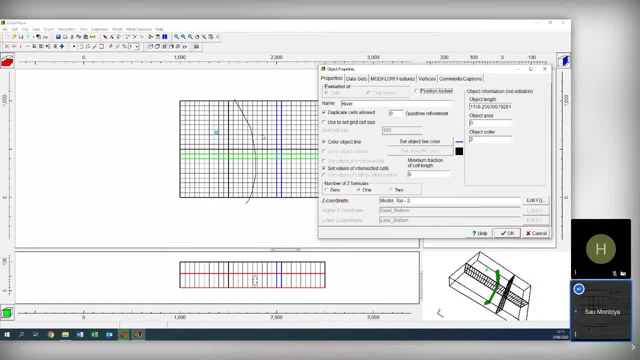 because for me I can say, okay, maybe the river wants like that, But if you import a river network you don't need to be, you don't need this option to be available, because you know that the river network is there. 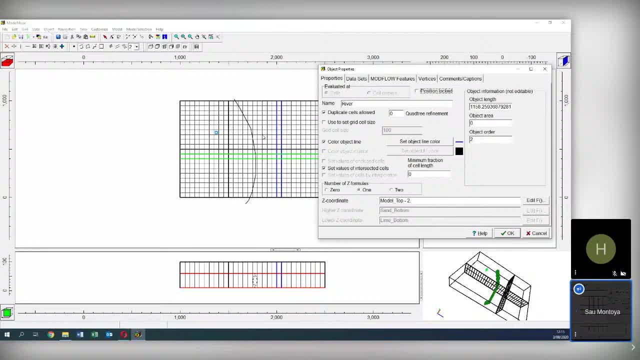 Okay. So, for example, we want that this river network, if we want that this river network won't be changed no matter what you do, we press here position lock. Okay Yeah, This is more on the for the quality of your simulations. 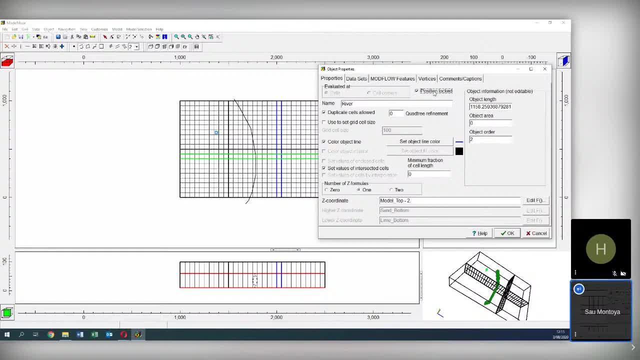 because you can um, um, you can create, you have the. you can be sure that the, that the object that you have imported- there, I mean- are in the required position. Okay, So so far, that's it. 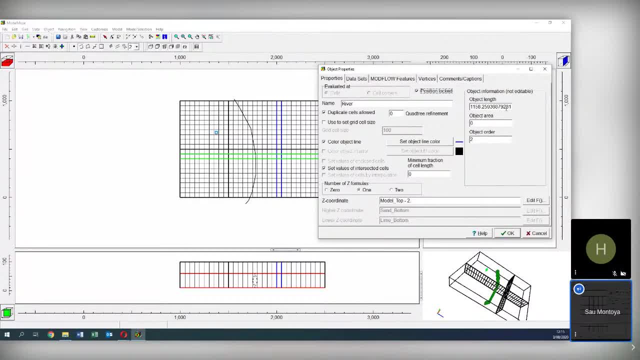 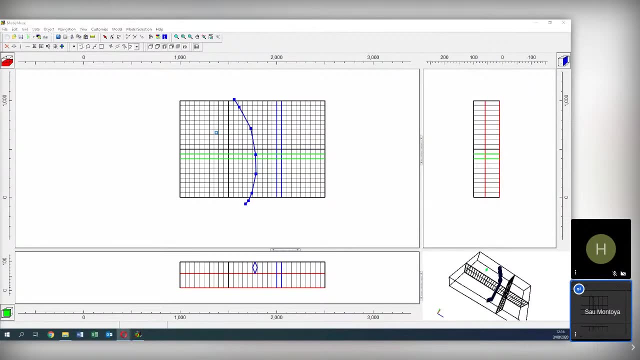 And if you are typing, if you have a line, actually the object length will appear here. Okay, And this is my second object, so the object order will be this one, And that is okay. Okay, And then I will create a polygon. 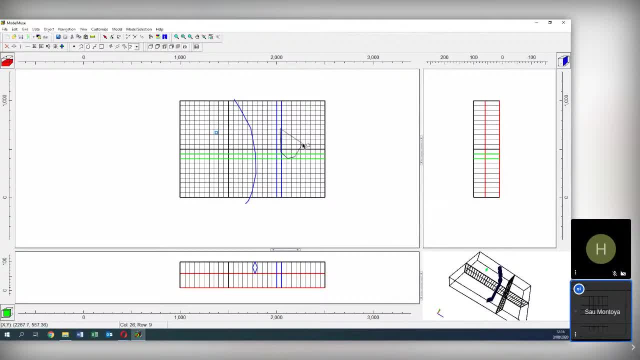 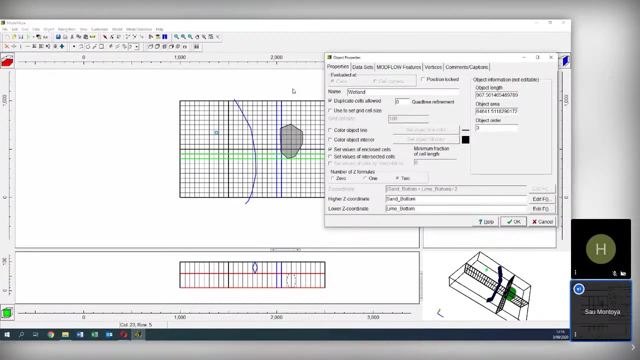 With this, I can create a polygon that is represented as a contaminant source, or something like that I can create. To finish, I do double click, Yeah, And then this is the wetland. for example, I can change color. 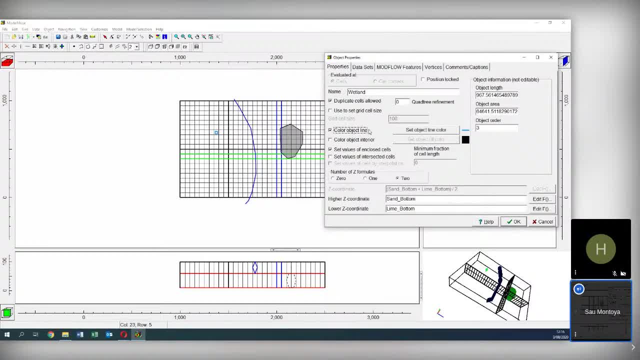 I can change the color of the outer part, But- and this, the visualization options of modern music are really, really scarce. but there is an option here to to define the inside color, the color of the polygon. Okay, And this one will. 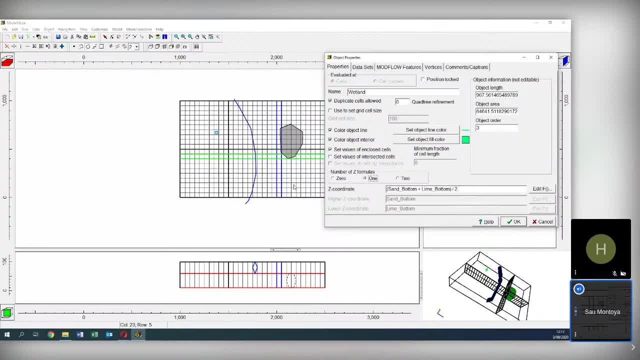 be three meters below surface, so it will be at 90 degrees. Okay, And this is this won't be position locked, because we there are options as well to to change the. there are options as well to change the position of the. 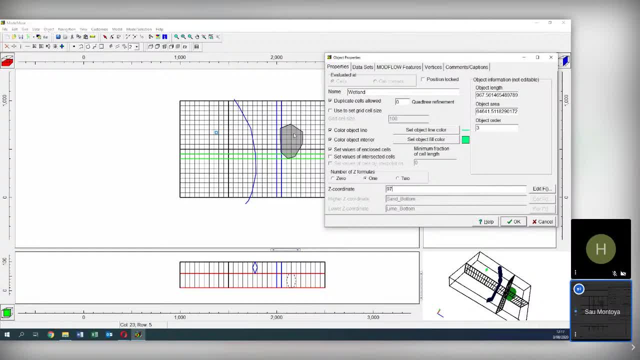 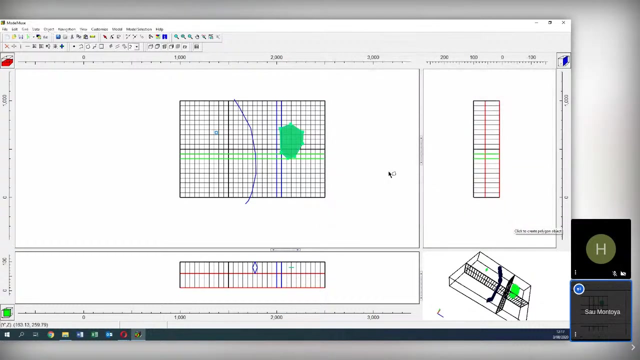 of the points. Okay, And then here, since you are working with them, since you are working with the, with the polygon, you have an area here, Okay, Okay, Everybody. if everybody is here, please guess 12. Okay. 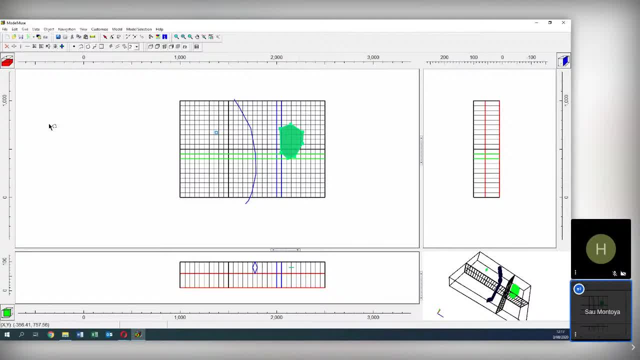 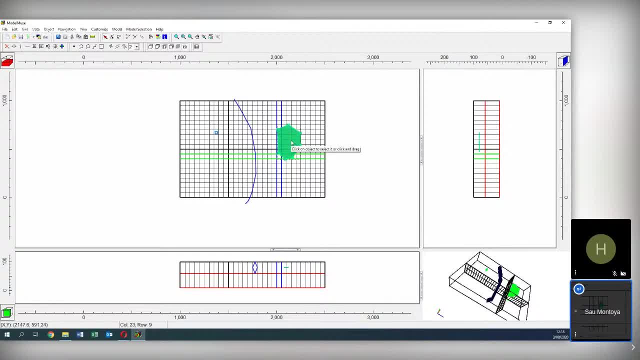 maybe this is. I mean, sometimes this can be required and sometimes this cannot be required. on your groundwater model, because you know explicitly what is your groundwater, what is, what is your object. Okay, But there are other options here. For example, I can move. 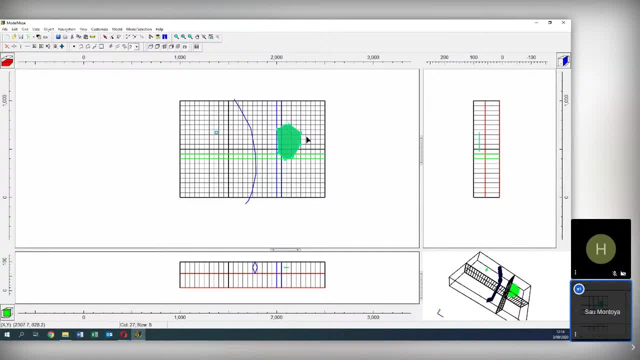 the vertex. I can select the vertex here and I can select the vertex here- Okay, And I can select it the vertex here as well and here- Okay, I can do small edits on the spot instead of, for example: 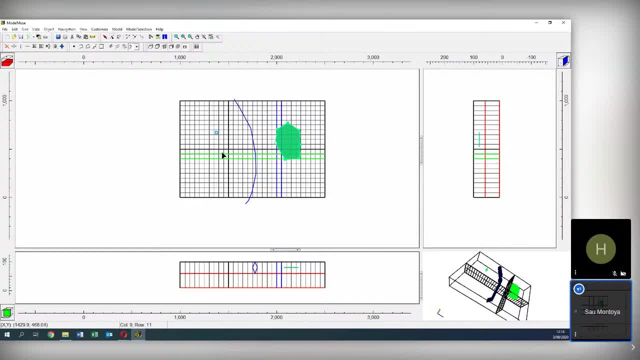 going back to GIS, to QGIS, and bringing back the and bringing back the object and doing the edits. here. I can do the edits right on monomers, Okay, Great. So with this, for example, I don't know. 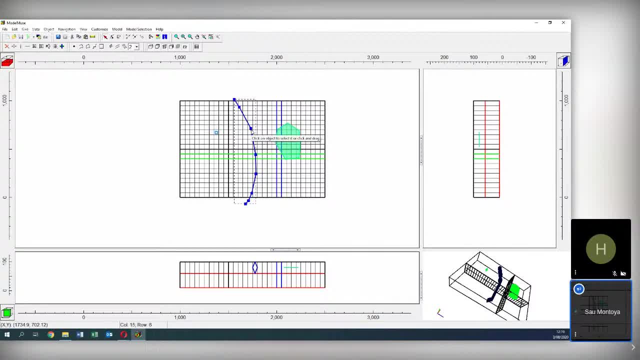 For example, I want to see if the river is position locked. I want to see if the river is position locked. I do double click with the, with the red, the red arrow, I select. When you know that it's selected because the 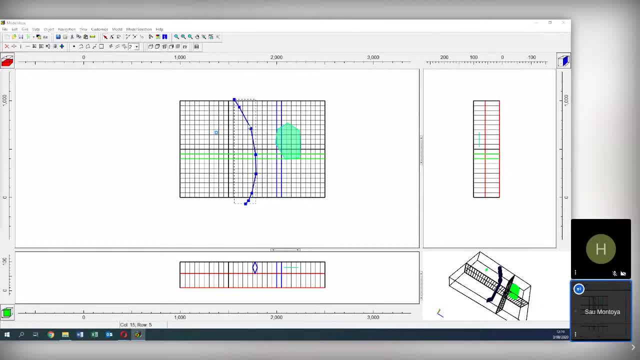 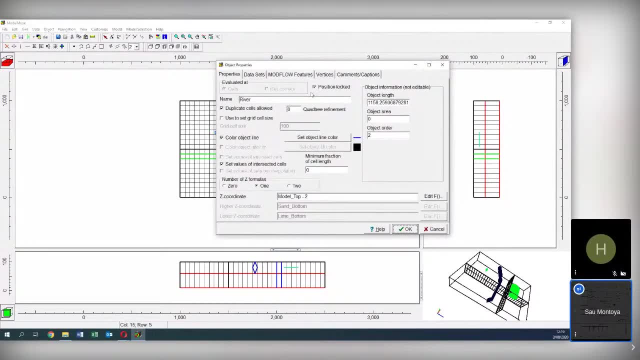 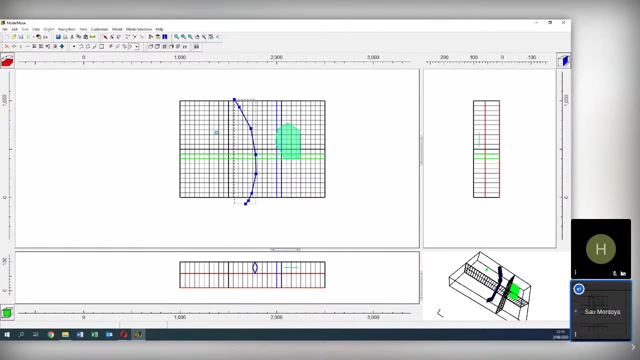 the vertex will appear, and then you do double click here and this appears here and I say, ah, it's position locked, So actually I cannot change this. Okay, So so far, that will be everything for today. 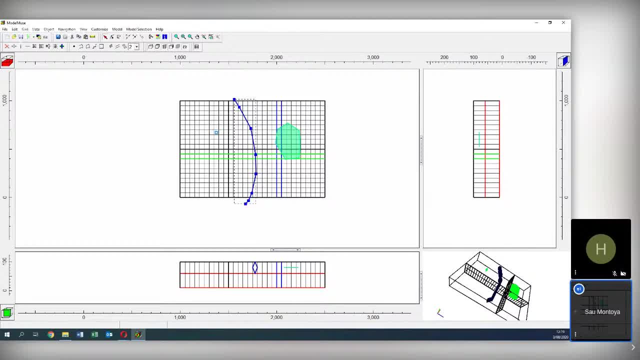 And then you were really arguing, Jose. Very mixed and very rich group of attendees and I'm really happy to have you provided this, this course, this class. See you on Friday. And there is a. there is a question of Farfan Yano. 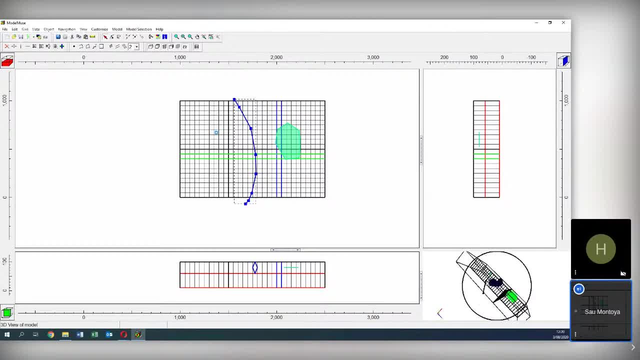 that say the river and everything is on the first layer, because, actually is, the objects are defined on the layer that intersect the object. since all of these are located in the first layer, Everything is located in the first layer. Okay, Ah Bueno. In my language say muchas. 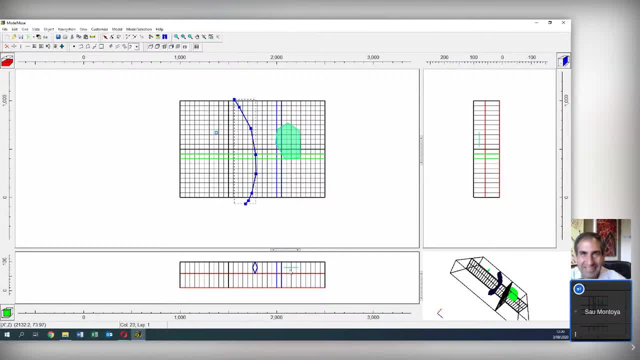 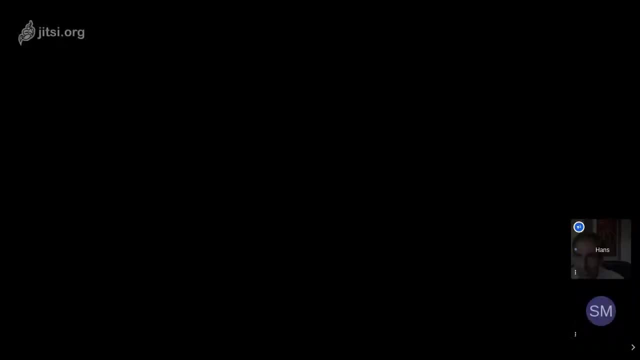 gracias. And Hans, I leave you to say goodbye of this class. Yeah, so thank you very much. Maybe you want to share your face also to say bye to the attendees, Let me. I'm very grateful that you give these free sessions, basically donated to: 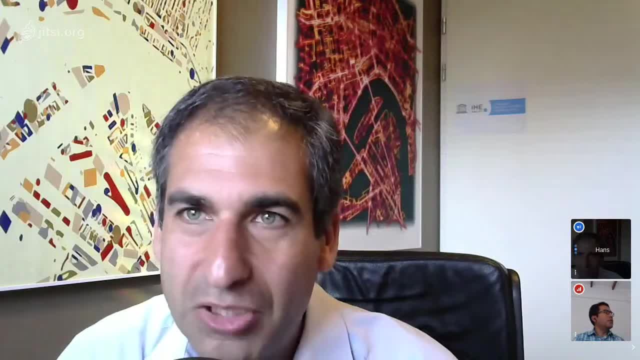 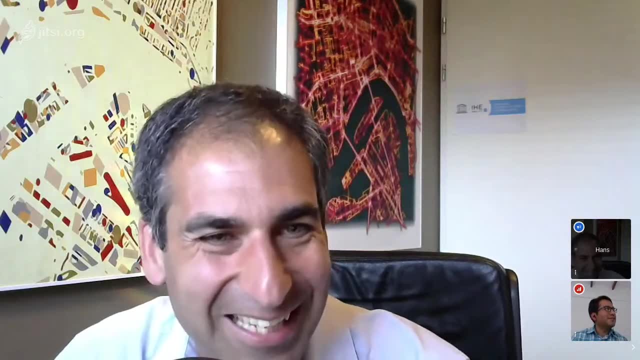 the OpenCourseR platform of IHE Delft, So looking very much forward to the next session. I'm learning also a lot from you. as a more in the, I now dive into the groundwater with you, Just to take the opportunity. I would like. 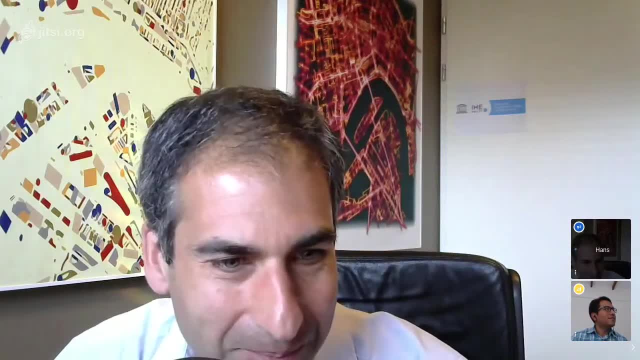 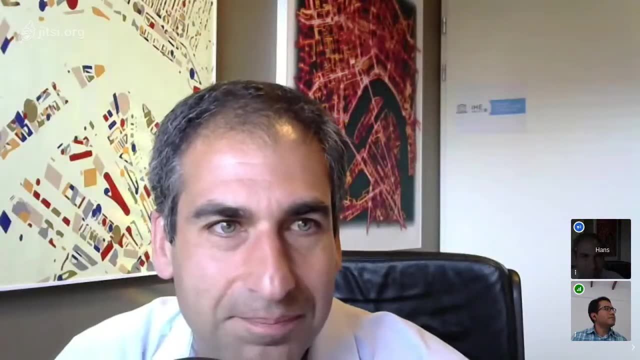 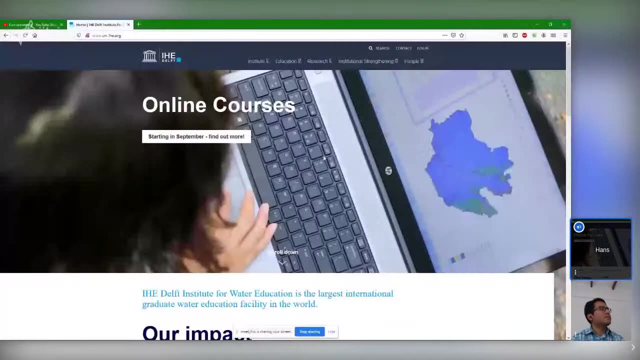 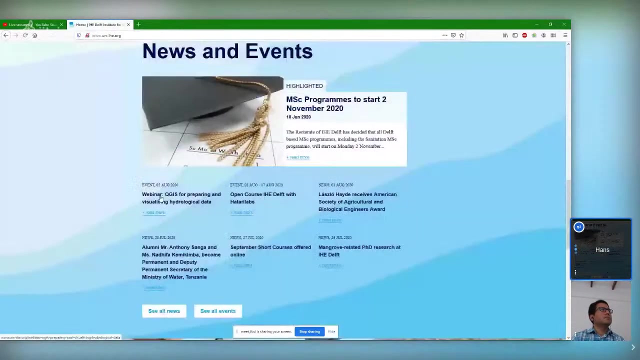 to share some other free stuff that is coming up this week already, So I'm going to share my screen One moment. So if you go to the IHE Delft website, then you will find here a link to a webinar on QGIS for preparing and 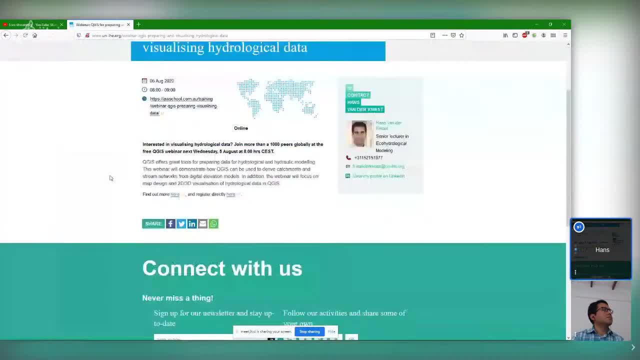 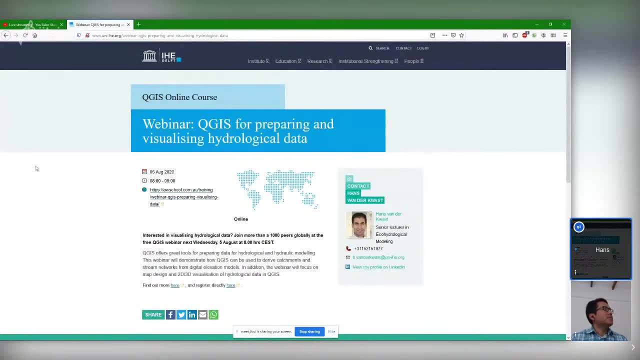 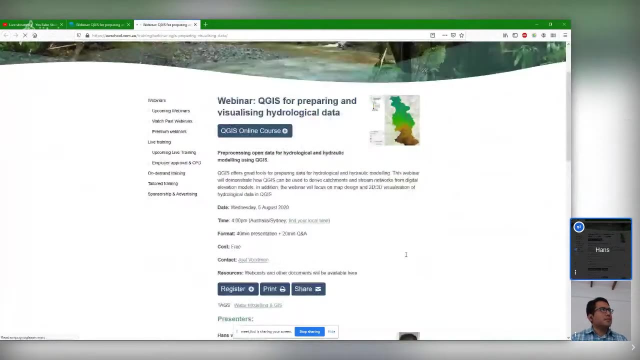 visualizing hydrological data. Already, more than thousand people have registered, So you can join it for free. It's organized by the Australian Water School, And Kurt Menke, the co-author of our book, will be speaking, And we'll have Saber Rajmoui. 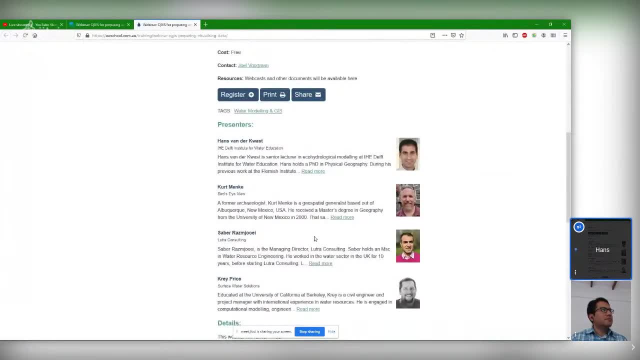 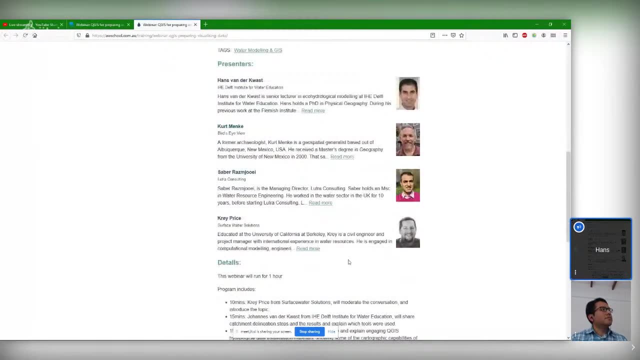 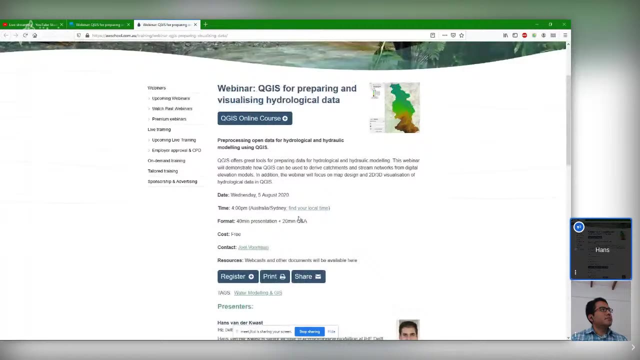 who is also working a lot with this company on the link between hydrological models and GIS, And there's Craig Price, who knows a lot about HEC-RAS modeling. So definitely nice to join this session, And after the free webinar you can also register for. 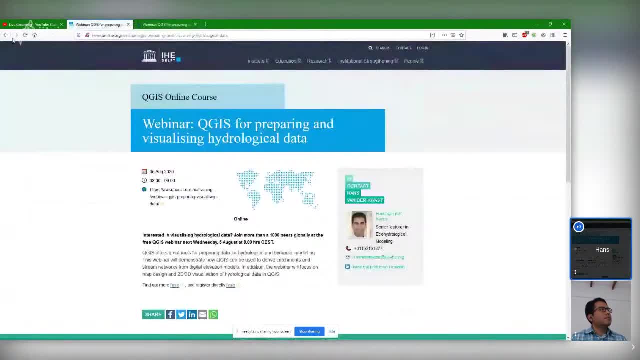 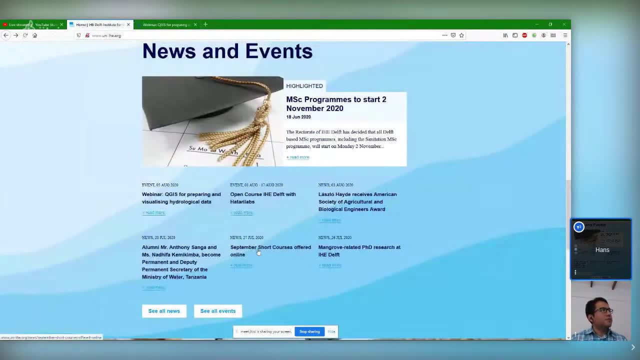 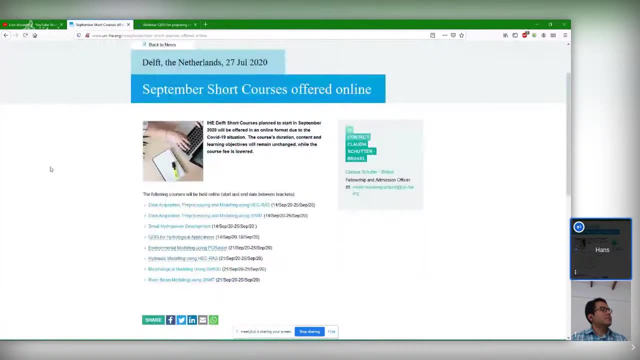 online courses. Those are paid. Another thing that I want to point out is that our September short courses are now offered online, So maybe you want to check it out. They are not free. We need a balance between, of course, what is free and what is not, But if you want, 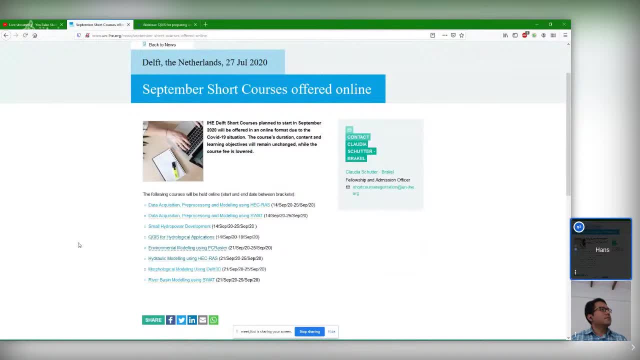 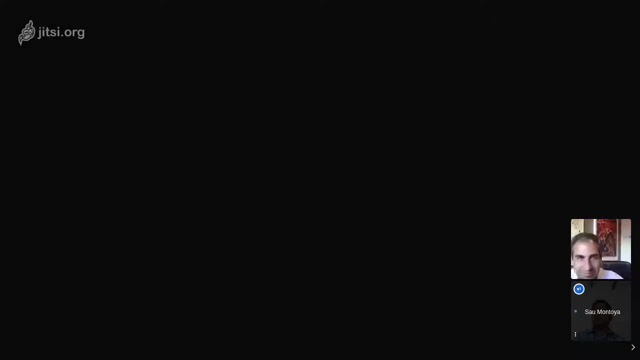 to have a certificate, an official QGIS certificate, for example- and support by Kurt Menke and myself. you can join this course now, from 14 to 18 September. Sol. you want to share something? Yes, Well, if you follow me by, 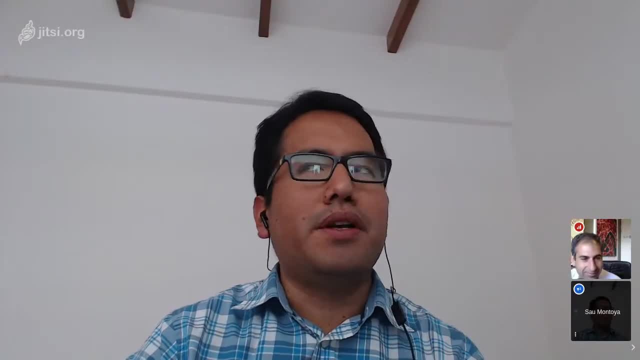 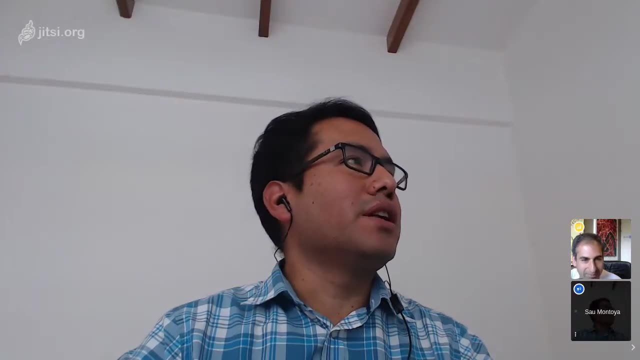 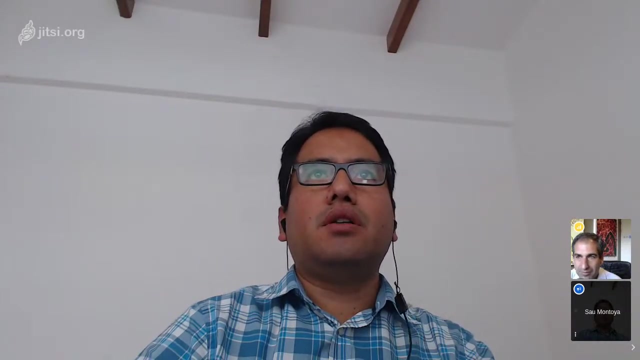 LinkedIn, you will see that I was very active in voronoi grids And I don't know if you are really interested in that. We have an e-learning platform. Ah, we have in Spanish as well. We have an e-learning platform in Spanish. 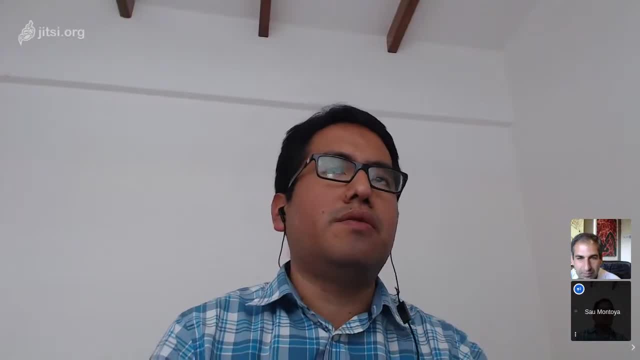 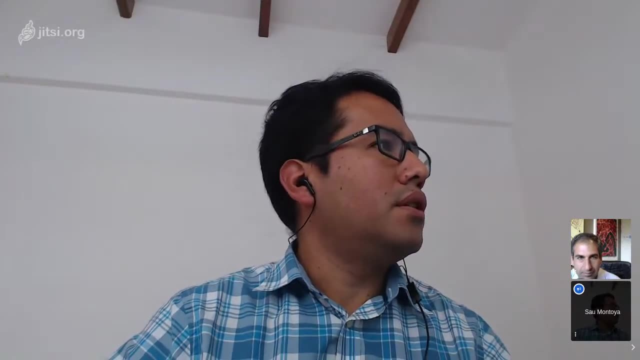 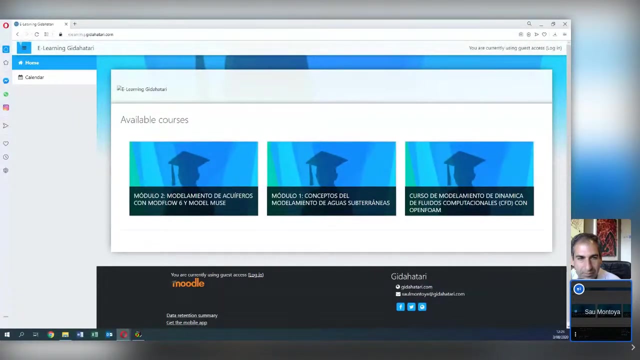 where we have some kind of diploma that is a joint of many, Where we have some diplomas that are the group of many courses in numerical modeling And next year they will be the first that we are going to provide in English And this is related. 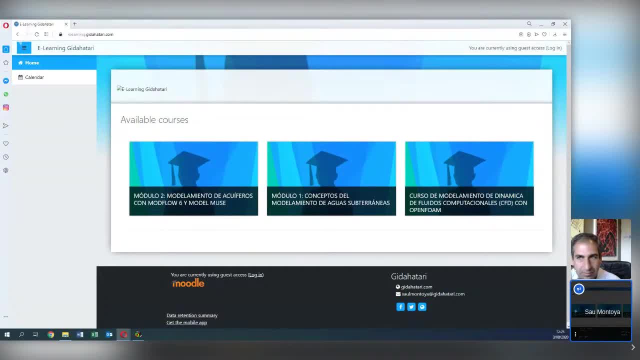 for some people that want to do like comprehensive or like they want to have a level where they can do a master thesis, or like working in numerical modeling. In English we have in the diploma. in English will be next year, but in Spanish we have been doing. 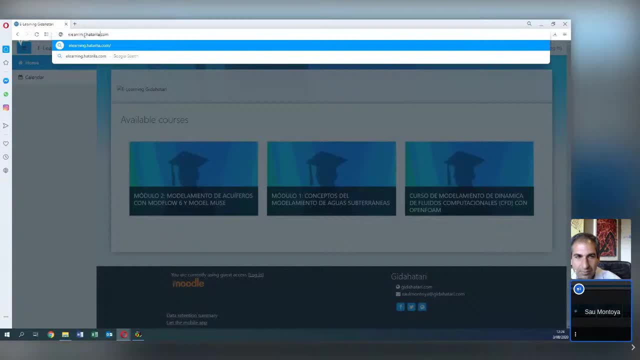 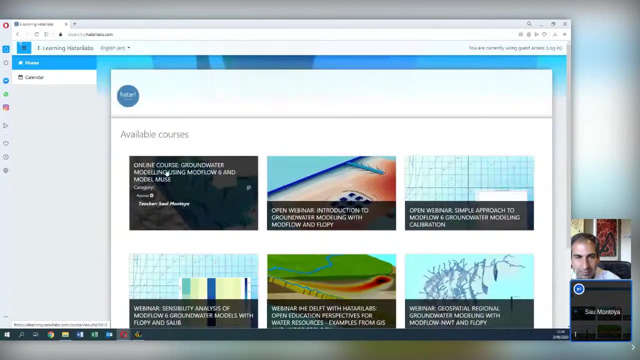 like. this is the form, And there we in English, we have an online course in groundwatering with mudflow a model used. This was a course that was even recently And there will be. there will be a course on mudflow and flowpipe. 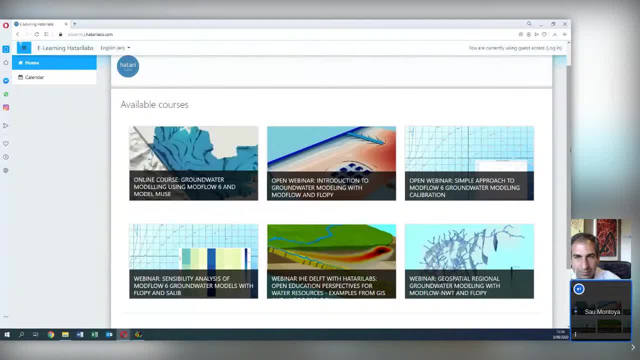 soon coming And there are some webinars of calibration, sensibility analysis and so on. If you are interested, you can. for example, this one is free so you can create your account, and this one is free as well. This one is paid because you see, because you. 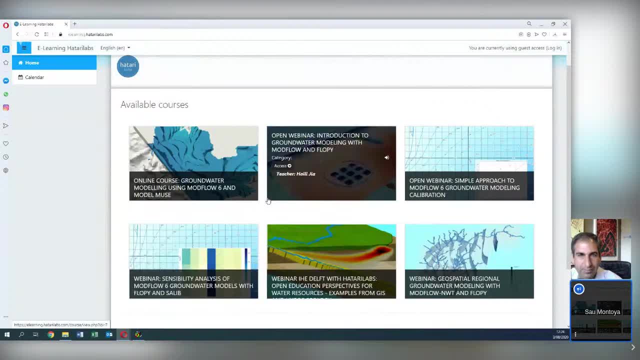 paid through Paypal. Okay, so, as well as Hans has said, there is this equilibrium of what is free and what is paid. but just to remind you that everything that we do, we do it because we love what we do and we do with passion to our